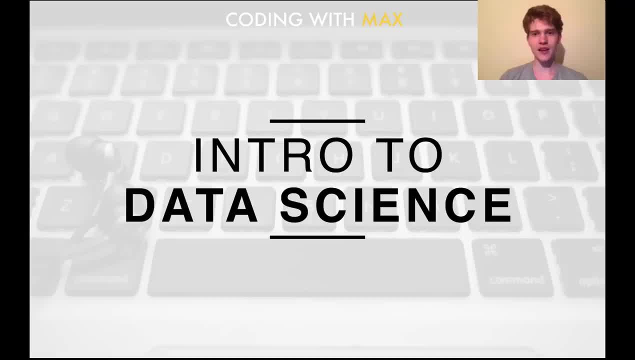 a lot, but its actual definition is quite vague. This mini-course is designed to help those of you who are curious about data science develop a better and more specific understanding of the topic. There are definitely more advanced techniques within data science, such as machine. 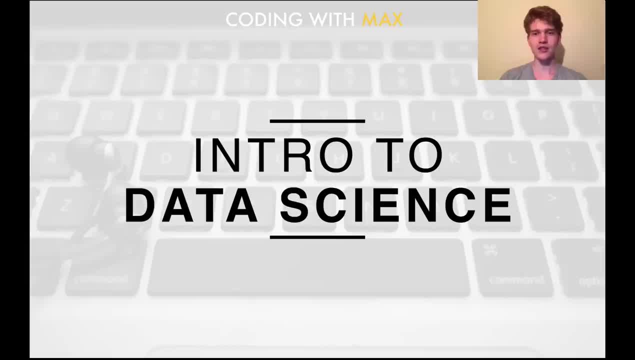 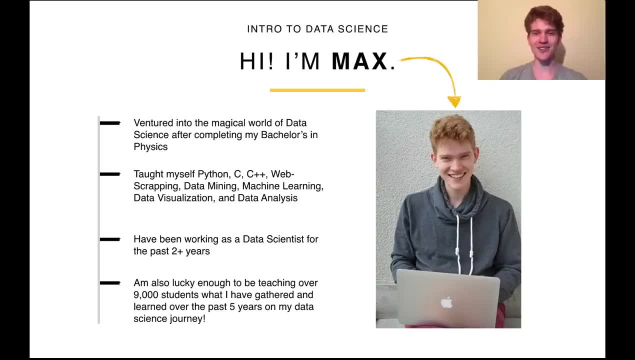 learning, but even these can be traced back to the three essential components that we'll cover. Before we get straight into it, I thought I'd quickly introduce myself. My name is Max and I work as a data scientist After getting my degree in physics. I find myself more and 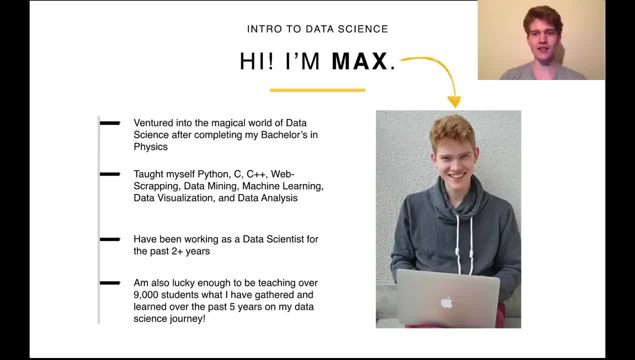 more drawn into the world of data science. So, instead of diving into the realm of physics research, I taught myself all the tools and techniques a data scientist needs, and shortly after that I became a data scientist. I've since also started teaching data science to others and have been fortunate enough. 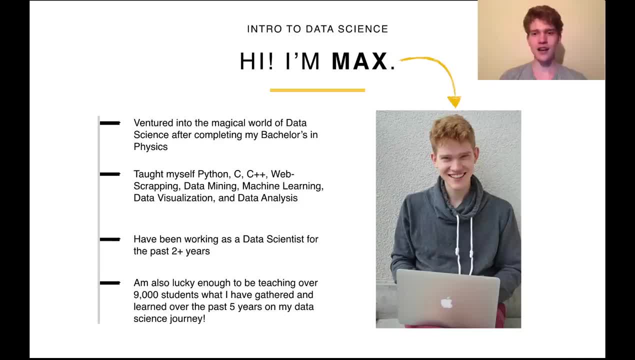 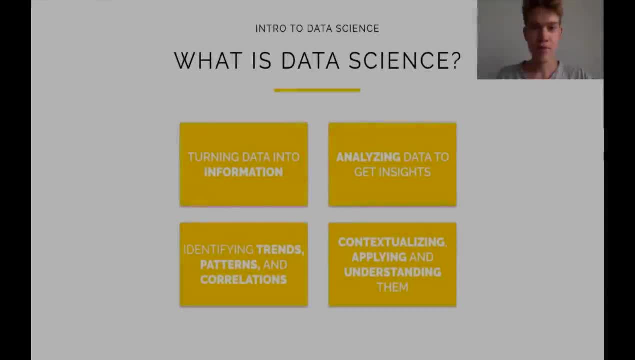 to teach what is currently over 9,000 students, the skills I've gathered and learned over the past five years of my data science journey. So let's jump right into it. So what is data science? Well, data science is. you can kind of summarize it in different 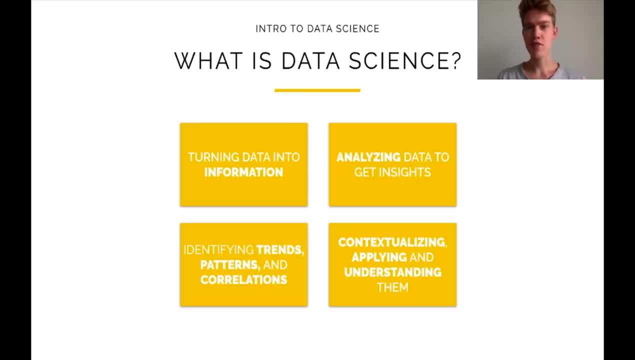 ways, but the main parts of it are transforming data into information, And this is a really big step because it's a very important part of data science. And it's a very important step because a lot of people talk about, you know, data and big data and all of these. 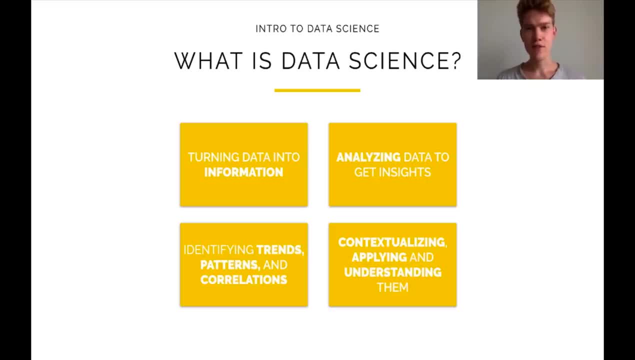 things. but data by itself isn't really that useful until you can turn it into information, And so if you just have a bunch of numbers appearing somewhere and it's just, you know so much of it, no one can make sense of that, And that's where you need a data scientist. 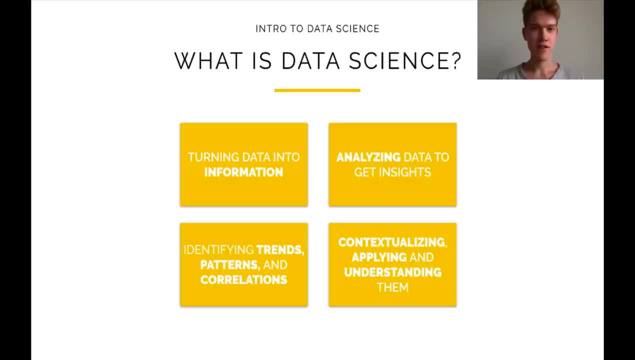 to be able to transform all of these, all of this vagueness and kind of this noise too. that's going on, and you need to be able to extract information from it, And that's what a data scientist does Now- what you do with this too, with this information, or how you get this information. 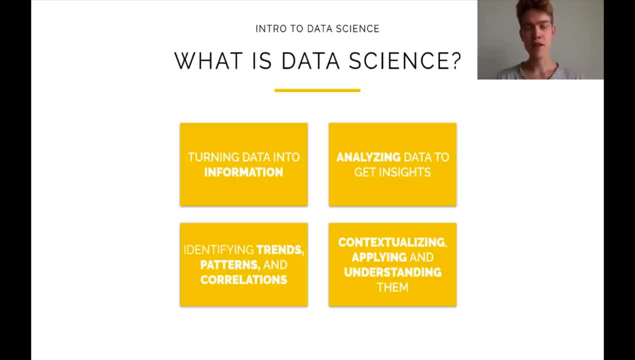 it's through analyzing your data. So a big part of it would be, you know, cleaning things up, doing some, some processes on it, and then you analyze once you've cleaned things up a little bit, And that is one of the ways that you can then get information out of your 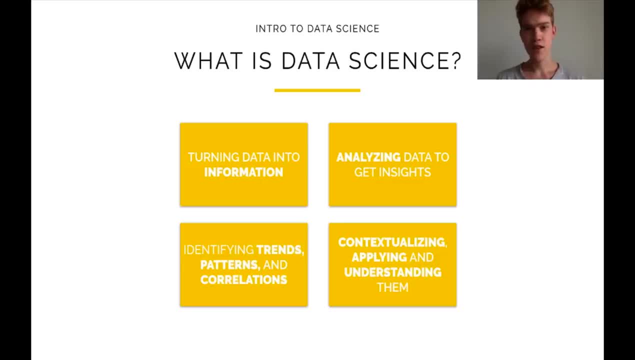 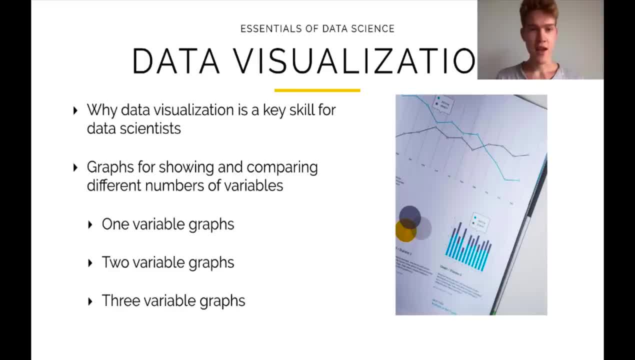 things again do a lot of work, and all of these things again do a lot of work, and all of these things again do a lot of work, and all of these things again do a lot of visualization, And we'll see why data visualization is a really key skill for data scientists, And 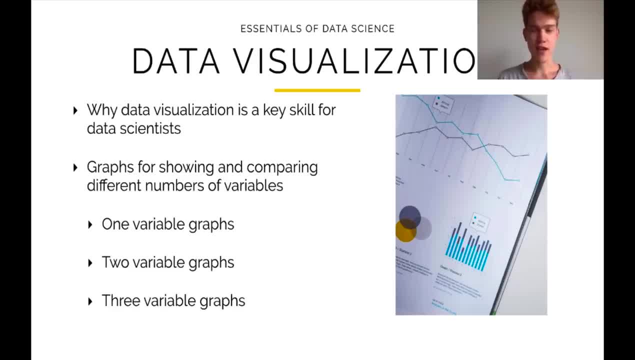 then we're also going to be covering different types of graphs that you can use and how you can compare different number of variables. So, for example, you can have one variable graph where you only look at one thing and you only want to look at this and you want to see how these, how, 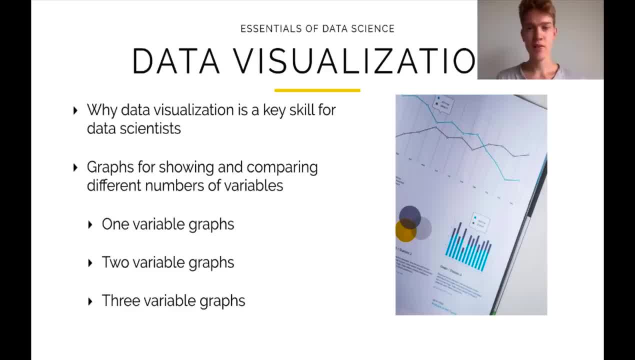 this changes. you have your typical two variable graphs, which you probably know, where you have this x and y axis, And then you can kind of see how two variables relate to each other, where you can have three variable or even higher variable graphs and where you plot maybe three different. 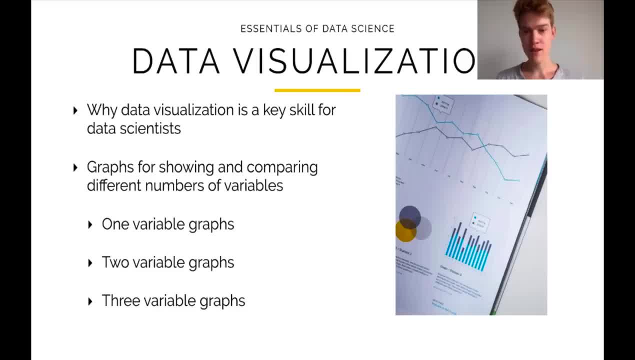 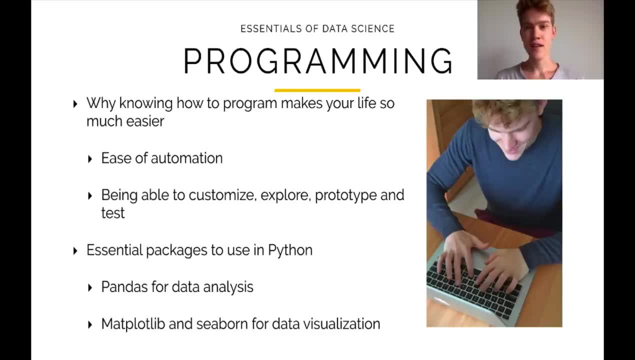 things- or even more if you want, as long as it makes sense- next to each other, so that you can compare multiple things at the same time. All right, And now we come to the other big thing that you're probably going to need as a data scientist, which is going to be the ability to 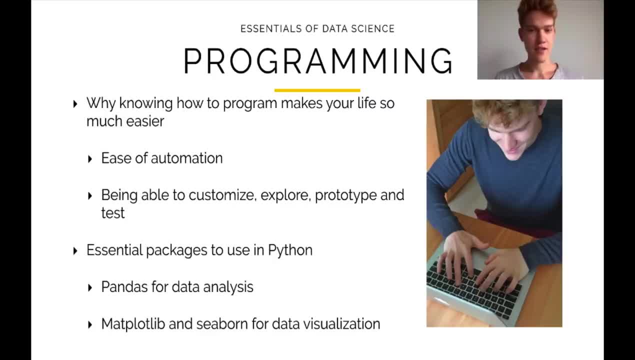 program. Now, not every data scientist is going to be able to program, So you're going to have to learn how to program, And I know a lot of data scientists can do this- But this is really, really essential, in my opinion, to your role as a data scientist, because knowing how to program is 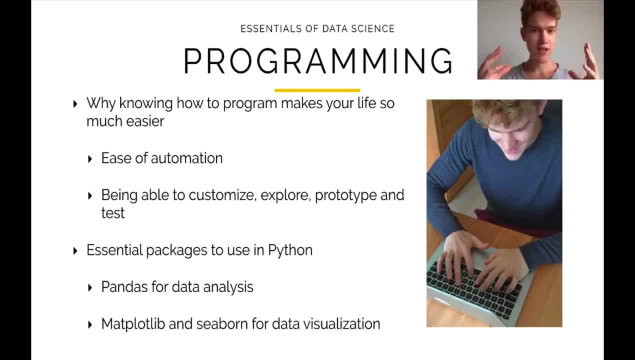 going to make your life so much easier. If you know how to program, you can kind of take your ideas and your thoughts and you can put them into actions in the computer And you can just automate everything. you can customize things, you can explore, you can prototype, you can test and 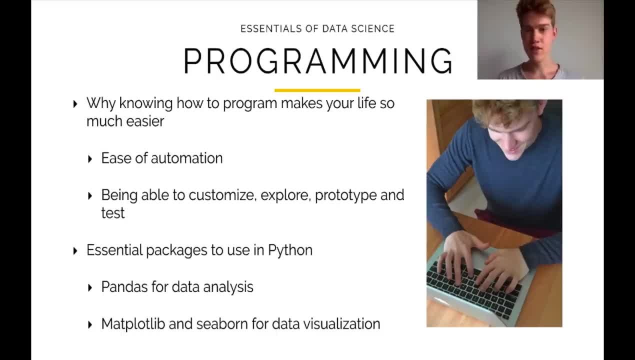 you're not reliant on some. you know application. you don't have to master some application And if it doesn't work, or if one thing doesn't work, you can just go ahead and do it, And that's kind of the 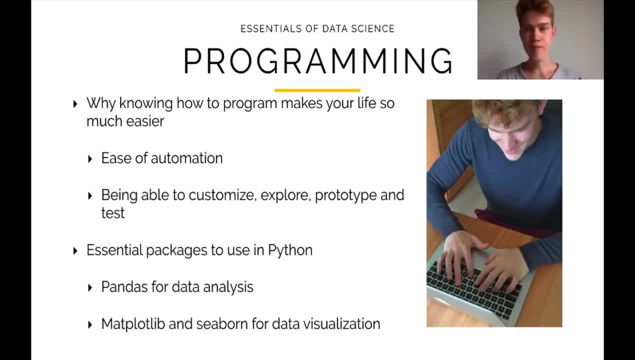 thing that you're going to need to do, And that's kind of the thing that you're going to need to do, And feature isn't there. you have to contact customer support And maybe it's not even possible And then you have to wait for an update or maybe something is bugged With programming. there's 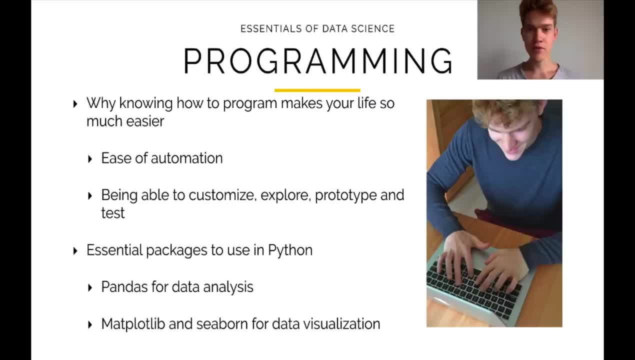 just you're so much more reliant on yourself And you can really just do whatever it is you want to do, And you're not reliant on other people or on the tools that other people have built for you, But rather you can just pretty much go and you know, just do what you want to do without there. 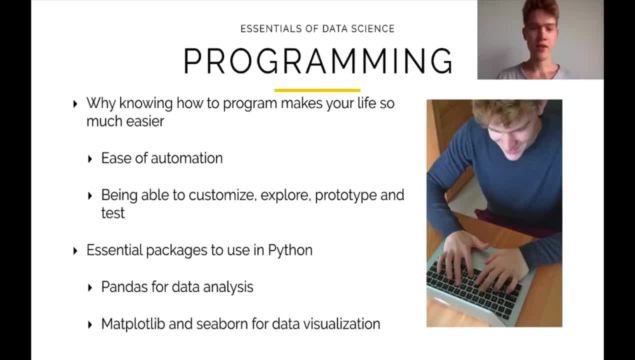 being major roadblocks, And then we'll also look at some essential packages in Python. So in programming you never want to reinvent the wheel, you always want to start off where the last person left off, And so the ability to program and be able to write simple programs you would. 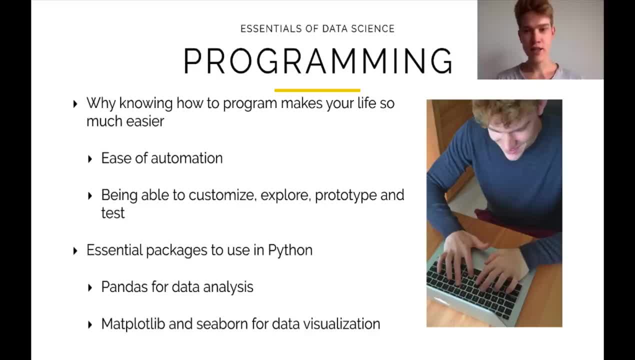 need to teach yourself, but you wouldn't need to write highly complex mathematical packages or data analysis packages. Those are already out there. all you need to do is be able to download them and implement them in your code And they're going to work. you know, they've been tested a lot. 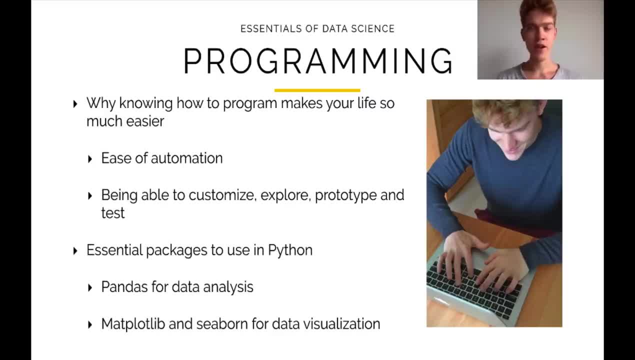 there's a huge communities working on them, on improving them and everything. All of this is for the community And so the whole community kind of works together to improve it. No one's really directly trying to make a lot of money off of it, So they're not going to charge you all of these service fees and everything Everyone's. 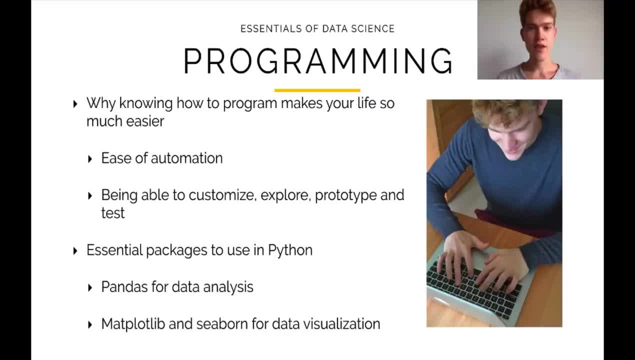 just trying to improve their package, because if it improves, everyone also benefits from it, And so we'll look at some of the libraries, or we'll talk about some libraries that you can use, especially in Python, and to help you along your way with data analysis and to become a successful 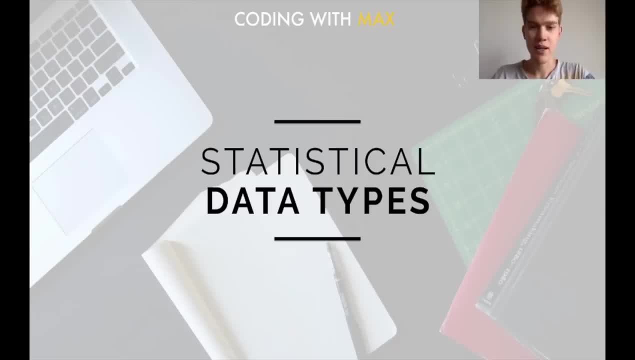 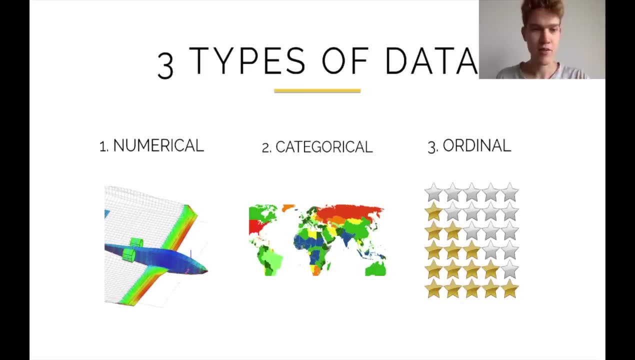 data center scientist. In this chapter, we're going to talk about statistical data types. Now we're going to look at the three different types of data, which are summarized as numerical, categorical and ordinal types of data. Now, these are the types of data that we talked about before. how you can't. 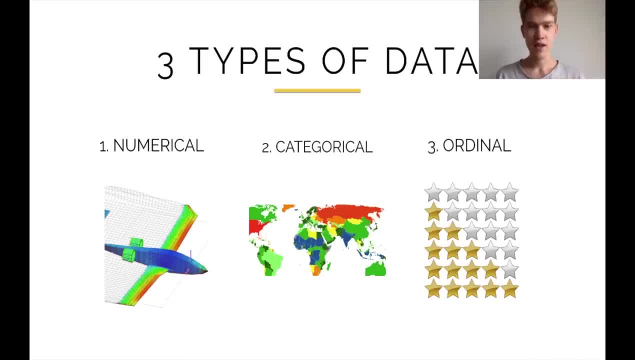 just expect your data to be cut, be kind of numerical, And so we'll see numerical data, but we'll also see the two other types of data that you may be, you know, encountering in your career as a data scientist. Alright, so let's talk about numerical data First, though. 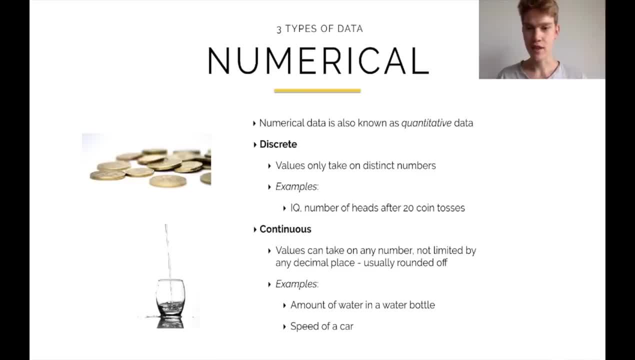 numerical data is also known as quantitative data, And it's pretty much things that you can kind of measure. it's great numerical stuff that you can do math with, you can compare it. you know, saying this plus this makes sense: A is greater than B. 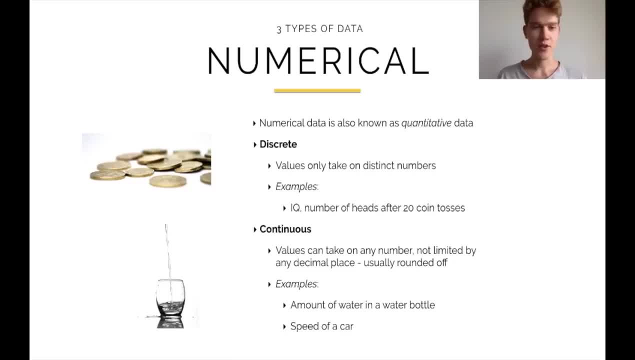 These are, you know, all examples of numerical data. numerical data can be split up into two different segments. One of them is going to be discrete, And so discrete means the values only take on distinct numbers, And an example of this would be, you know, IQ or something like that. 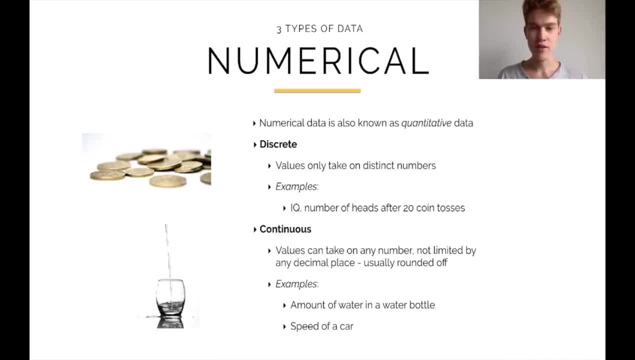 a measurement of IQ or if you do a coin toss, the number of times that you toss heads. so you can, you know you can have 15 heads, you can have 12 heads out of you know, 20 coin tosses. 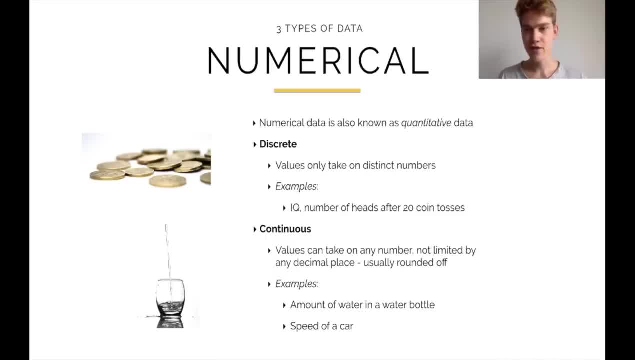 you can have 500 heads out of 1000 coin tosses, or 500 out of 600, or all of these things, But all these are distinct numbers And now they don't have to be whole specifically, but they do have. 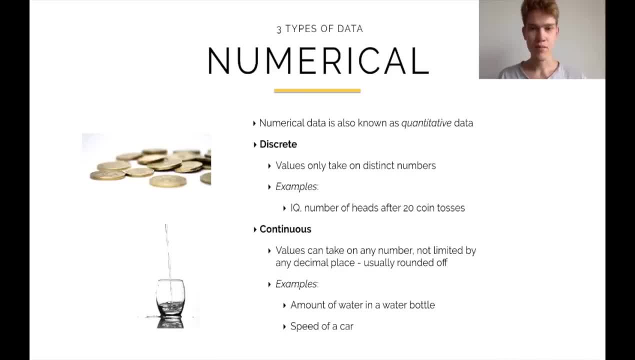 to be distinct. So that's, that's the kind of very important part that you know. there's a kind of step size that you're dealing with And of course you can still say: hey, you know, flipping eight heads out of 20 is better than flipping seven heads out of 20.. If you want to flip heads, that 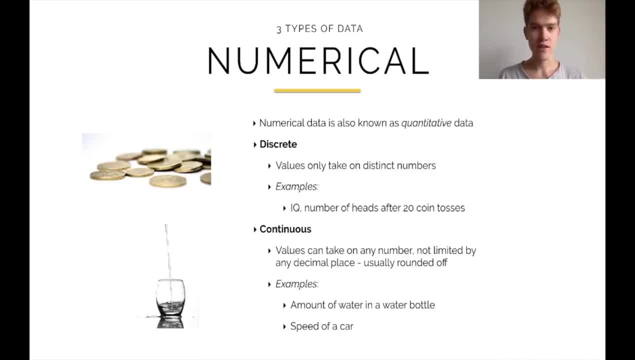 is, or flipping eight out of 20 is worse than flipping seven out of 20, if you're going for as many tails as you can. So all of these kind of comparisons, they make sense. So that's the discrete part of numerical data. 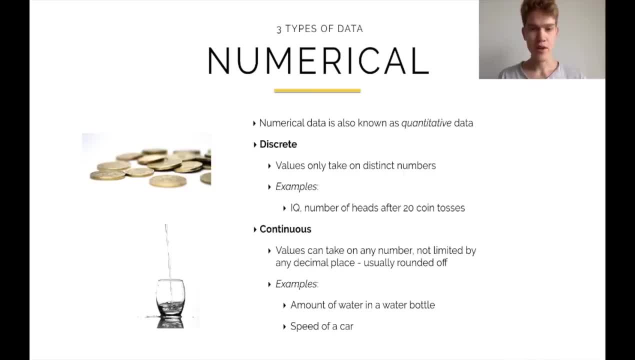 Then we have the continuous part, And now the continuous part is really that values can just take on any number and they're not limited by decimal place. So a value that can you know can be like 1.1., And then the next value would be 1.2.. That's not continuous, that's still. 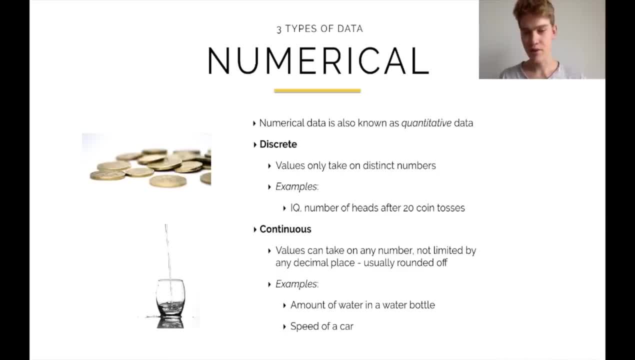 discrete because you have this step size of 0.1.. Continuous means literally every number, from start to finish, can be taken on, And this doesn't mean that every possible number in the universe, from negative infinity to plus infinity and all imaginary numbers and everything that comes with. 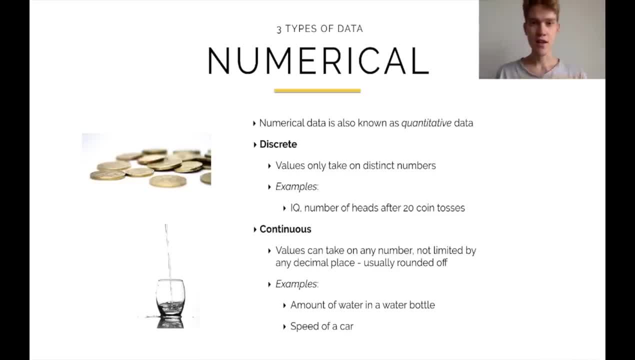 it. that doesn't that that's not required for continuous. it could really be that just every number between zero and one can be taken on. So, for example, let's say you have a bottle of water and this bottle of water can hold one liter. Now if you fill your bottle up and it starts off empty. 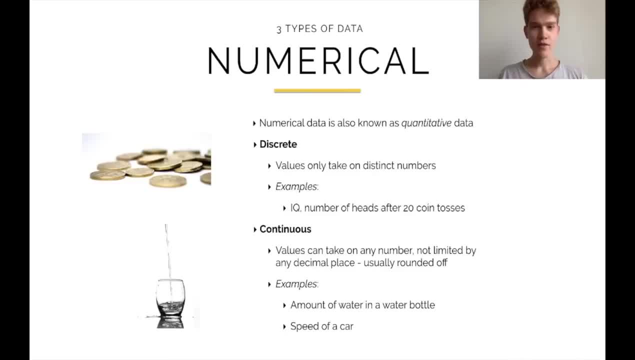 and you fill it all the way up to the top the amount of water that you've had needed to take on every single number between zero and one, because you can't just fill up water, you know kind of small increments of say, hey, I'm going to put in 0.2 liters every single time because 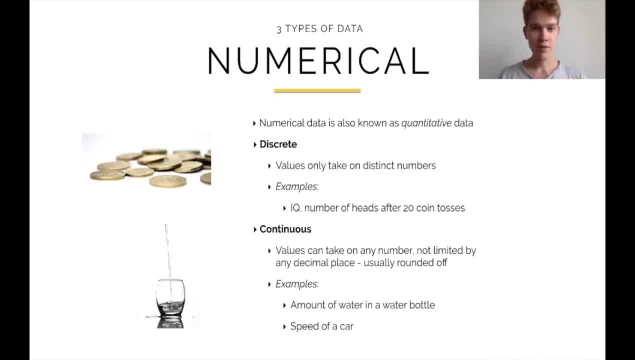 the water doesn't just, you know, teleport from A to B, But when you're pouring in water it's more like we see in the stream here, and the water level rises and rises, and rises, And so the amount of water that we have in our cup needs to take on every value between zero and one. So that's an. 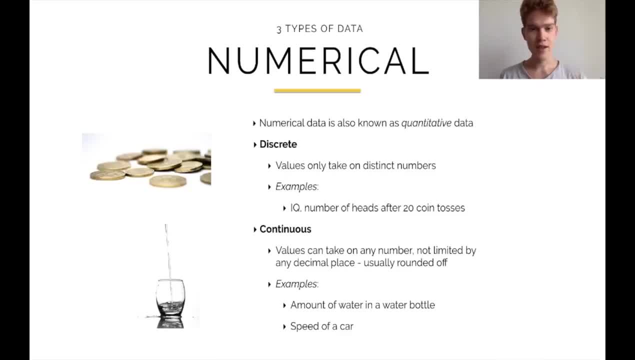 example of continuous data for. But you see that you know we can be limited to zero and to be between zero and one. we don't have to, you know, start at zero and go all the way up to infinity or something, But it's just that the range that we're looking at, every single number can- can be applied. 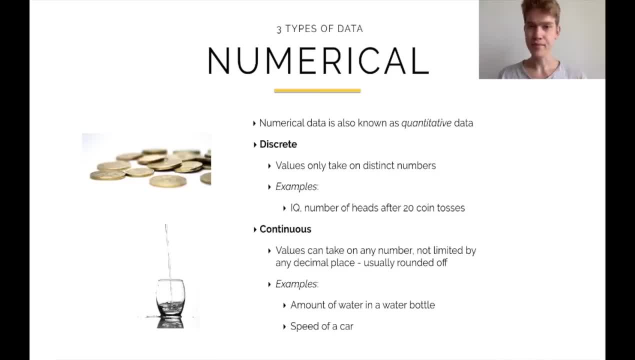 or every single number can you know happen? Another good example would be the speed of a car. If you start and you know you're standing still and you're starting, you're standing at a stoplight and then you want to accelerate. 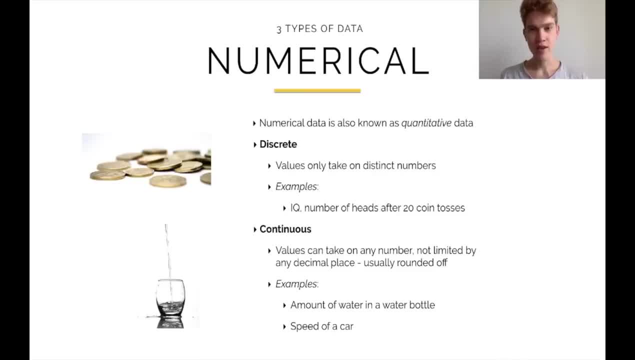 and the speed limit is, say, you know, 50 miles an hour or something. to get to 50 miles an hour from your starting position, your car has to take on every single speed in between And of course you won't see that you know on your spot. on the speedometer it would say something like: 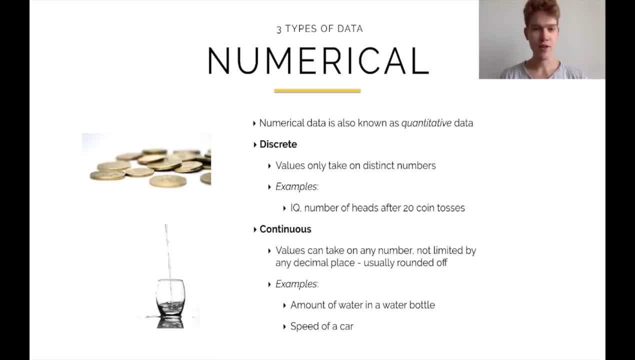 zero miles an hour. one mile an hour, you know. maybe you can go to like it's going 0.1,, 0.2,, 0.3, or something like that. So it may look discreet to you. But 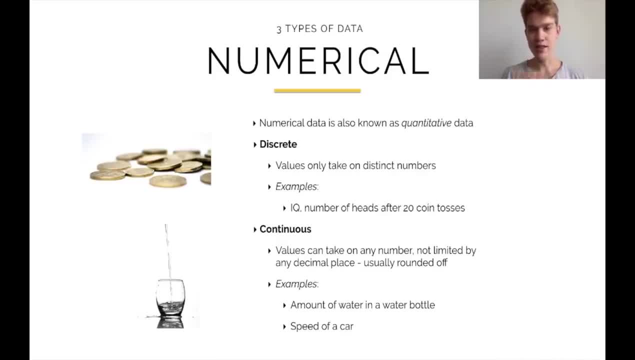 that's not how your car is going. Your car doesn't say like, oh, I'm going to go in these step sizes of speed. it's going to accelerate And it's going to take on every value, starting from zero, going up to 50 miles an hour. And you're going to when you're in this transition, you're going to take on. 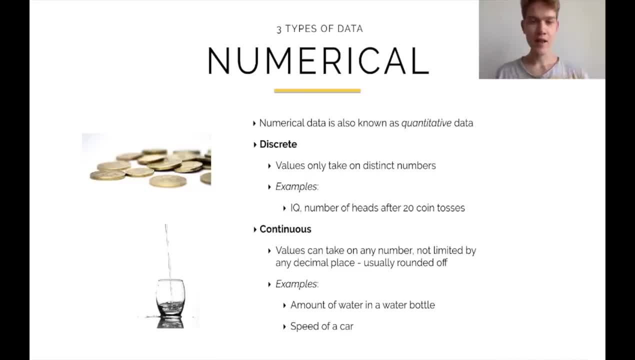 every single one of those speed values. So that's how continuous data looks like, And it's important to know that you're dealing with continuous data. And you're dealing with continuous data rather than discrete data. And you're dealing with continuous data rather than discrete data. 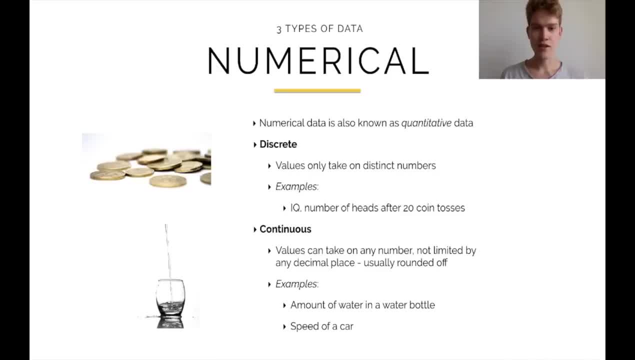 Now, of course, if we're dealing with computers, our computers can't deal with infinite numbers in the decimal places. we have to cut it off somewhere, And so usually continuous data is going to be rounded off at some point. But it's still important for you to know that you're 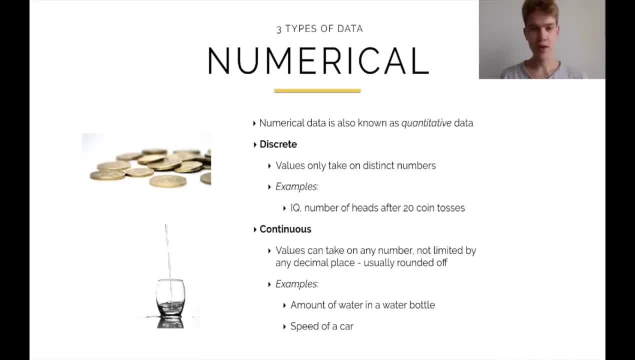 dealing with continuous data here rather than discrete, so that you know, hey, there can still be other stuff in between here and or all of these things, rather than you know having a big step sizes and all you see is just kind of a bunch of lines at every step size. But you can. 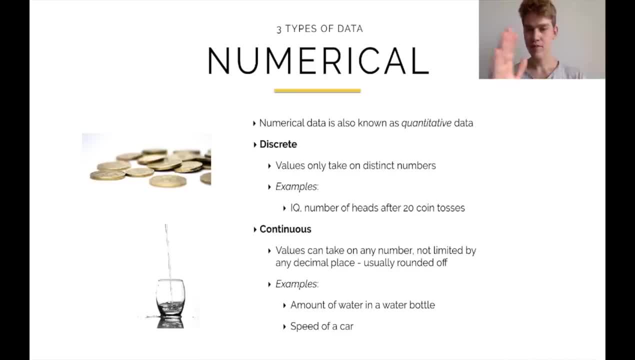 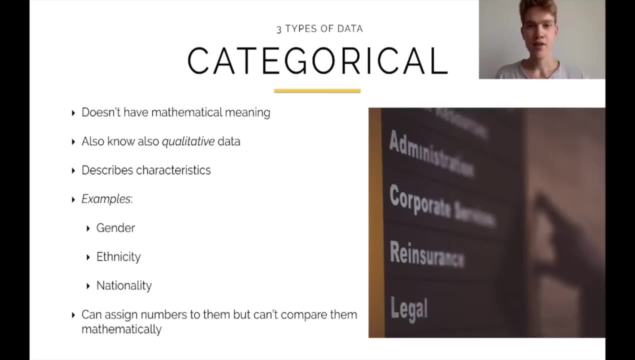 expect that when you have continuous data, that everything is just kind of filled, filled up, that everything can and may even well be in between certain places. So that's that's kind of the important thing to note between discrete and continuous. Alright, so the next type of data. 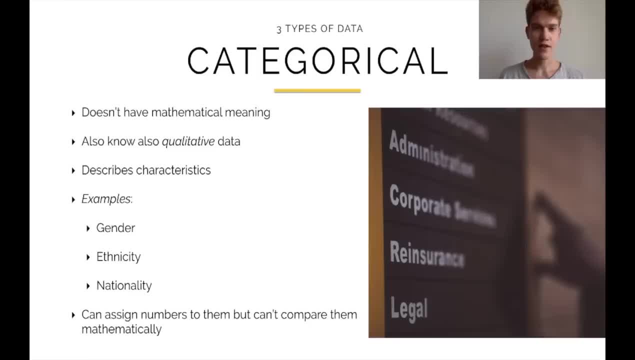 that we'll have is categorical. Now, categorical data doesn't really have a mathematical meaning. may also know it to be qualitative data and categorical data it describes characteristics. so a good example of this would be, for example, gender. so here there is no real mathematical meaning to gender. of course you know if you have. 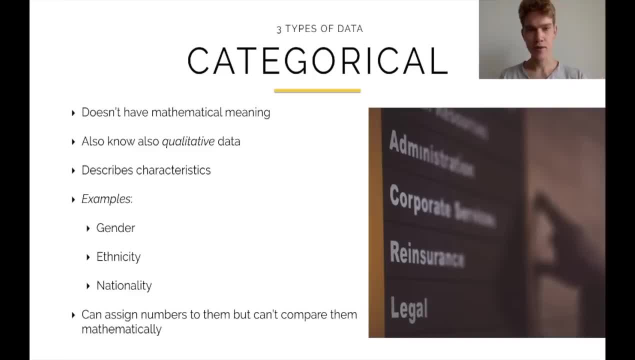 the data. you can say: male is 0 and female is 1, but you can't really compare the two numbers, even though you assign numbers to them, and you may just do this so that you can split it up later on. there your computer can understand, but 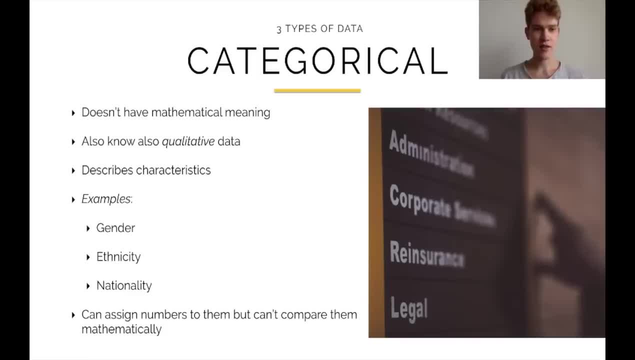 it doesn't really make any sense to compare. you can't say: you know, is male equal? you wait, you can say male is not equal to female, but you can't really say is 1 greater than the other or is 1 approximately equal to the other? those 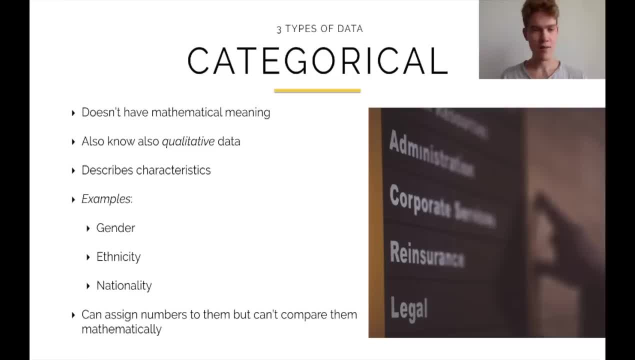 things don't really make sense because they're not well-defined. what does that mean? and you can't really add them up either. you can't say male plus female, but that doesn't, doesn't give you a third category or something. so categories they. you really apply math to them. but they're nice ways to kind of split up or group your data and they. 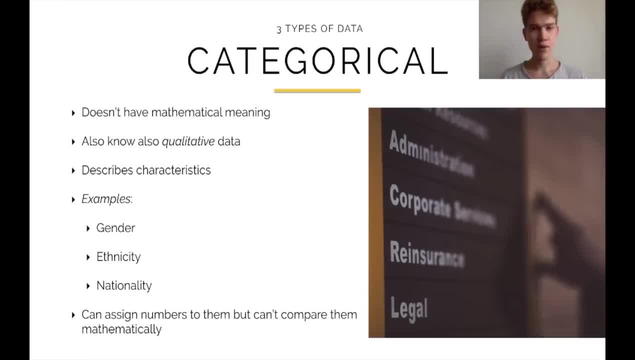 provide these nice qualitative pieces of information that are still important. it's just you can't really go that well about you know, like plotting them on a line or something like that. so those are important things to note with categorical data, and then another example would, for example, be ethnicity, or you could also have nationality, all of these things. 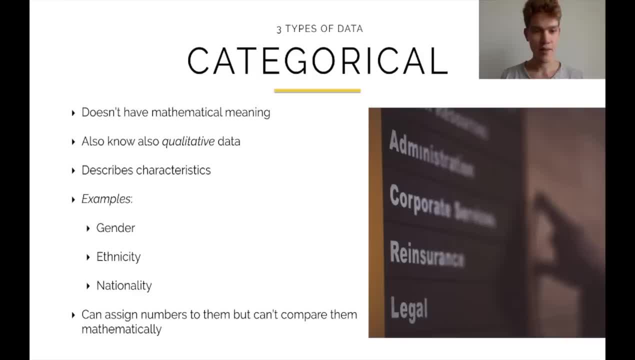 and are examples of categorical types of data. yeah, and so, like we said, you can assign numbers to them, but that's really just for your code, so that it's easy to kind of split them up, but you still can't really compare them. how are you going to compare nationalities? there is really no definition for 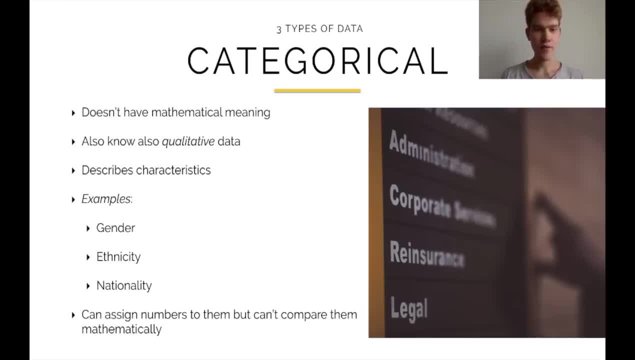 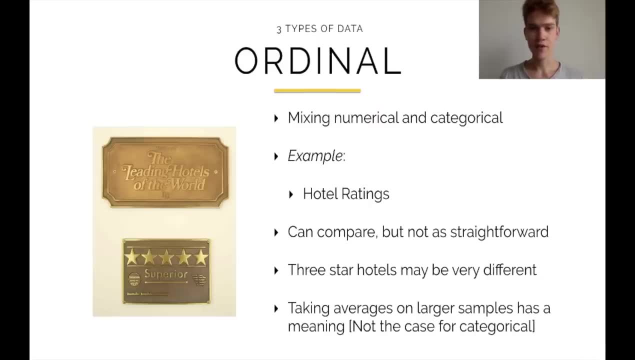 you know, comparing one type of category to another. all right, and so the third type of data that you can encounter is something called ordinal data. now, ordinal data is a mixture of numerical and categorical data, and a good example of this would be hotel ratings. so you have, you know, star ratings there of zero, one, two, three, four or five stars, or maybe even six. 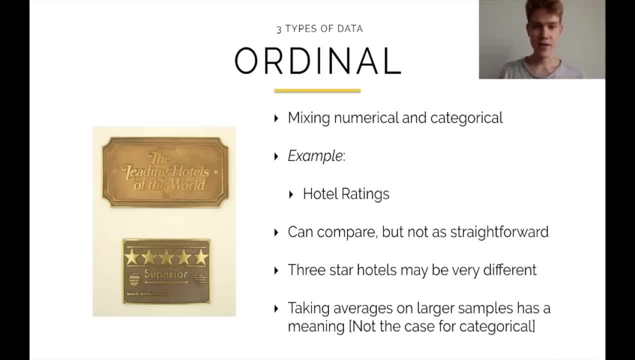 stars or you know whatever it is, whatever the hotels go up to these days, um, but it's still not as straightforward to compare. so i'm sure you've seen two different types of three-star hotels. one of them, you know, had the bare minimums. the beds were okay, but it wasn't really anything. special, and so the third type of data that you can have is like the number of hotels that you can compare. so there's a mixture of numerical and categorical data, and a good example of this would be hotel ratings. so you have, you know, star rating zero of zero, one, two, three, four or five stars, or maybe even 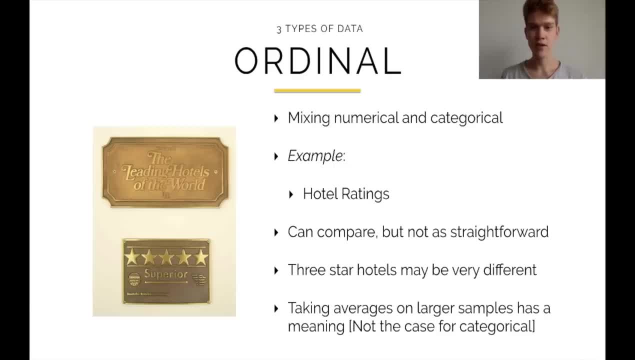 And then you had those three-star hotels that you could have sworn were at least four-star, And so star ratings do make sense. We can say: you know, a four-star hotel is probably better than the three-star hotel because there have been standards. 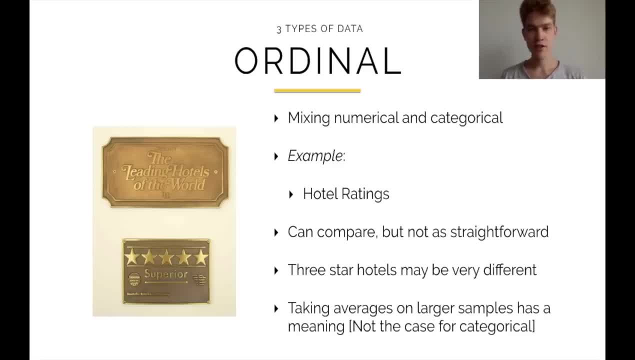 There are standards for these things. They have been checked. you know, If you go to a four-star hotel, you know what to kind of expect, But still it's not completely defined. So, like you know, coming back to this three-star example, 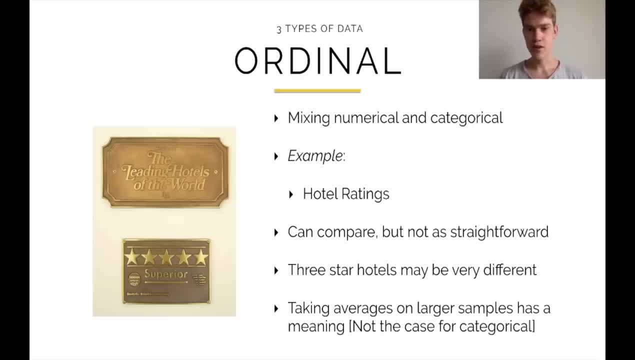 it's very hard if you just say, hey, we're going to a three-star hotel. It's very hard to know exactly what to expect, because there are different parts of three-star hotels. There are three-star hotels that have developed on to, like, have a swimming pool maybe, or something like that. 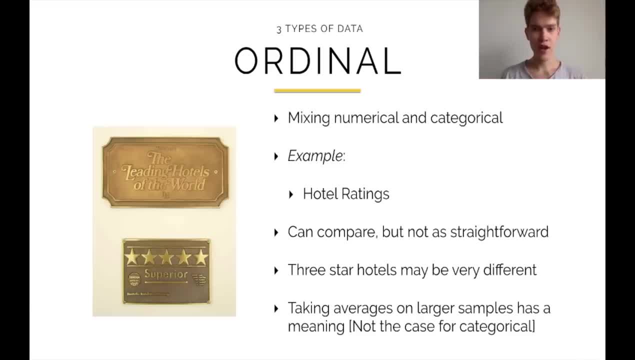 And there are those three-star hotels that are really more like hostels or something that have just made it past the two-star place, And so there it's much harder to kind of define or to know what to expect Now if you take averages of these star hotels. 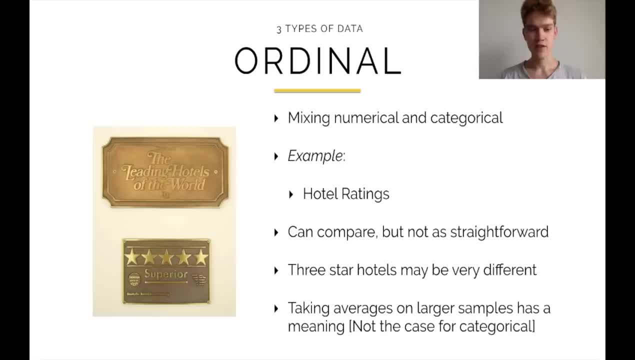 our systems, though, then you do get a much better idea of what's going on. So if you have, you know, consumer reviews or something like that, and you say, oh, from you know 500 reviews, our hotel has an average rating of like 3.8.. Then you know that the three-star hotel that you're looking at is pretty much a four-star hotel. It feels like a four-star hotel, even though it may not have all of those qualifying characteristics. That's the kind of feel you get from it. 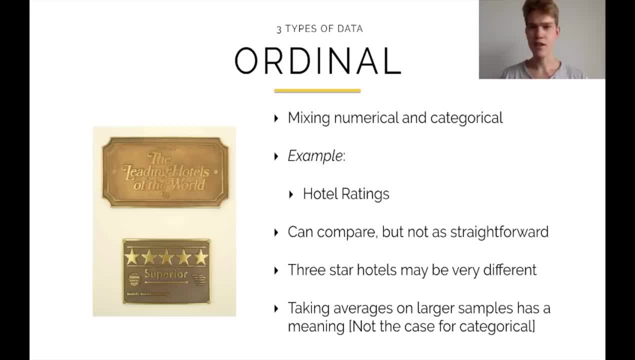 Whereas from another three-star hotel you may have a rating of like 2.9 or something, and there you know. ah, you know, this hotel is more towards the lower end of the three-star. Some people may not even consider it to be three stars. 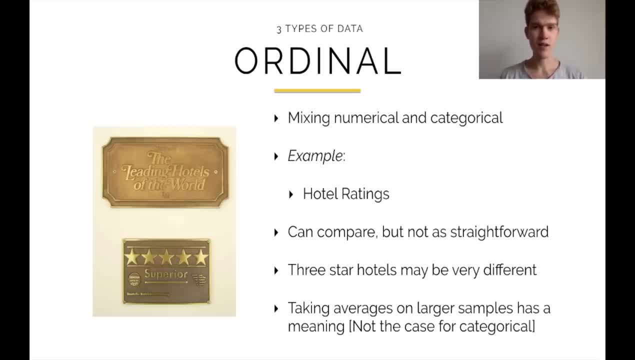 And of course you know this rating may be a little bit biased, because they went to a different three-star hotel first and then they went to this one and they were expecting something completely else from a three-star hotel. So they said: this can't be three stars, This is two stars. 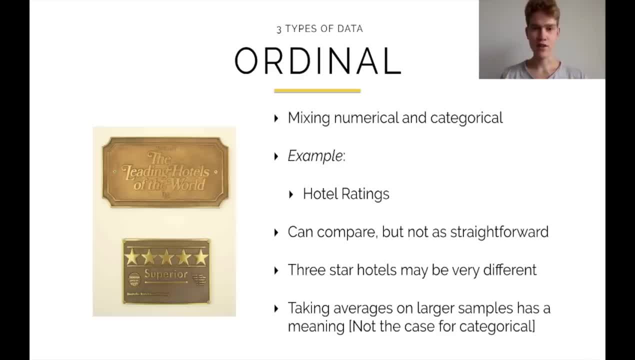 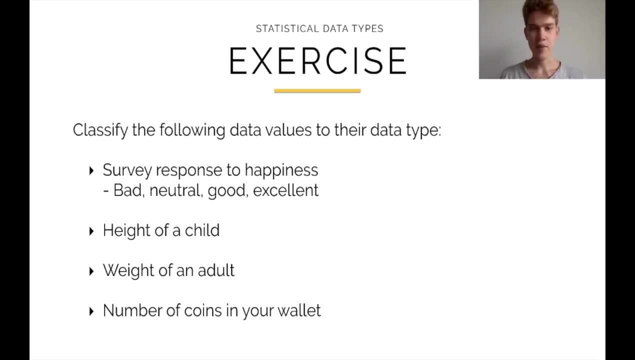 But it's because of the way that the ranking system is defined, underneath and everything, And so when we have these averages with these ordinal numbers, then they kind of start to make a little bit more sense. Alright, so let's go over a small exercise and see if we can identify what type of data we're dealing with. 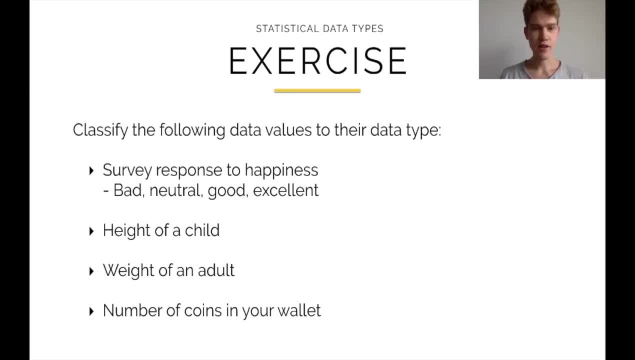 So the first thing we'll look at is going to be the survey response to happiness. Now you have people filling out a survey and then one of the questions is: you know how would you rate your happiness? and it's going to be bad, neutral, good or excellent. 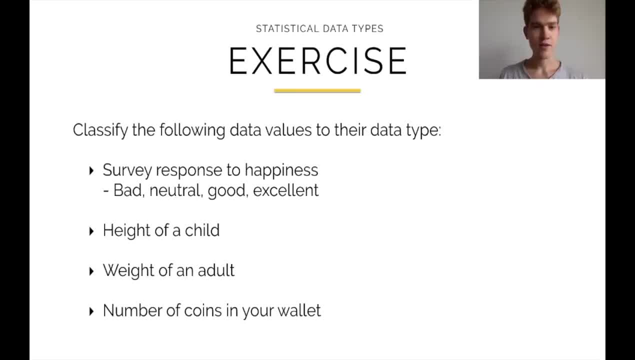 What type of data would this be? Well, this would be an ordinal type of data, because it's still a form of categories and you're asking for the subjective opinion. but it does make sense, So you can still compare them. You can say: excellent is greater than good, Good is greater than neutral, Neutral is greater than bad. 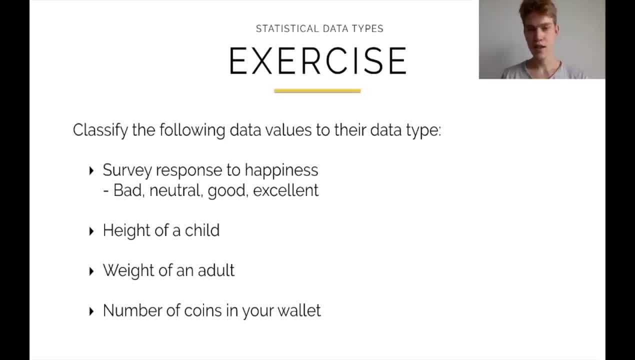 But what exactly does it mean to be good and excellent? You know where do different people draw the line for this, So there's it's still a little bit of vagueness involved, but generally it does make sense and you can compare it. 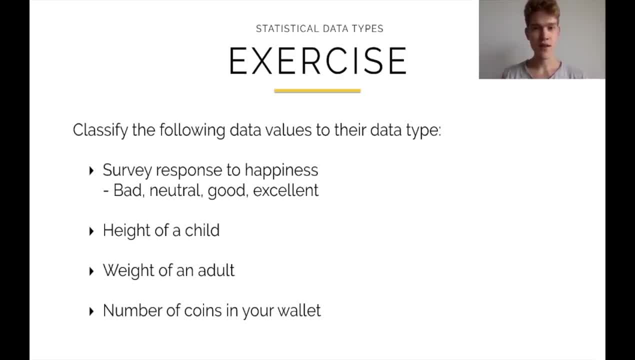 And if you have a lot of surveys and you average them, the values you're going to get are probably going to be very well representative, or at least pretty good representative. Alright, so if we look at the next thing, which is going to be the height of a child, 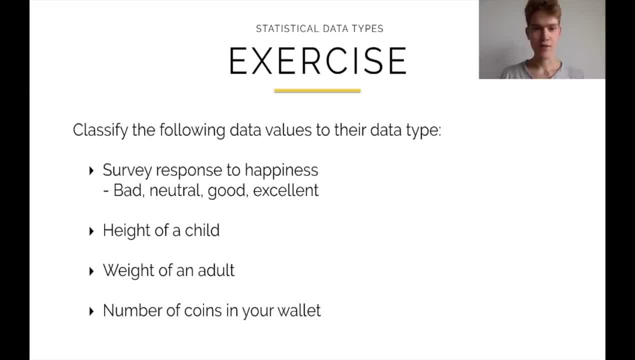 What type of data is that? Now we can say it's probably numerical. and well, it actually most definitely is numerical. So the height of a child is a numerical value. but let's go a little bit deeper and say: is the height of a child discrete? 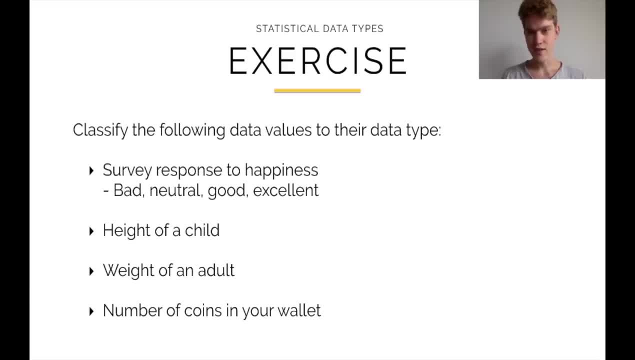 Or is the height of a child continuous? Well, even though when you measure height you get something like you know five foot, I don't know five foot three or 160 centimeters or something like that, It's not a discrete value, because to get that height you have to have reached every single height before. 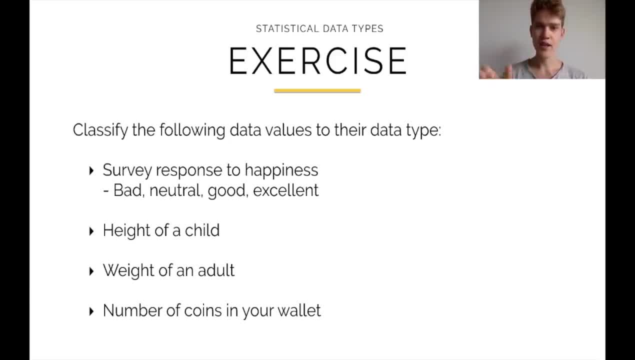 And so, even though at the moment you may be measuring it, you're kind of rounding it off to how much you're measuring tape can measure. So, like you're measuring tape is kind of limiting the height, But if you had a super, super precise measuring instrument you could measure not just, you know, five foot. 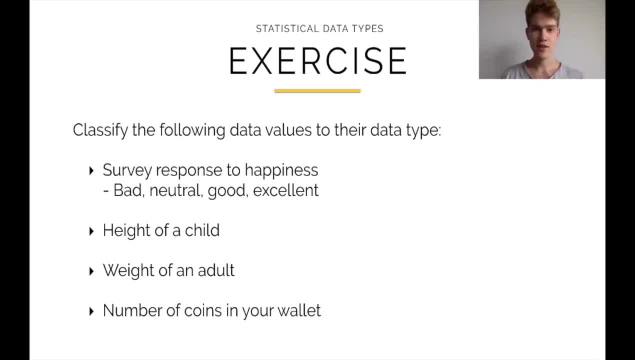 three or something like that. You could really go into detail with the inches and the decimal places in there and everything kind of going on. So the height of a child would be a numerical data type, but it would be continuous. Alright, now let's talk about the weight of an adult. 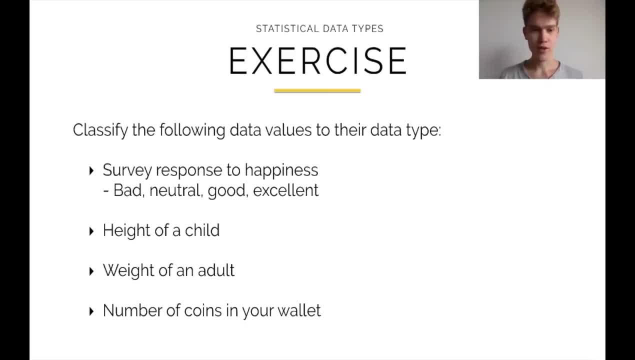 Do you expect the weight of an adult to be either discrete or continuous? So we can probably agree that it's numerical because it's a weight value. It's pretty much defined to be a number. But do you expect it to be discrete or continuous? 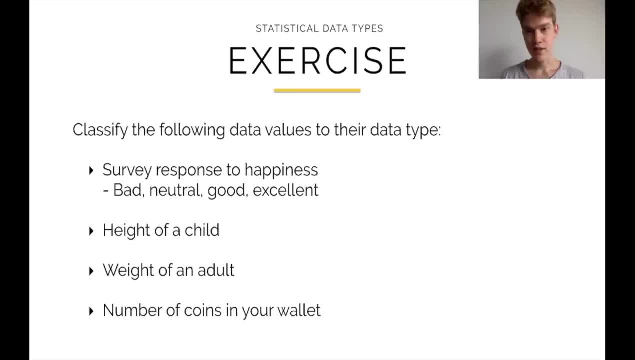 Well, the right answer here is going to be continuous again, because to reach a certain weight, they would have had to have reached every single weight in between before. So, again, the weight is something that we can consider to be continuous. Alright, and so finally, 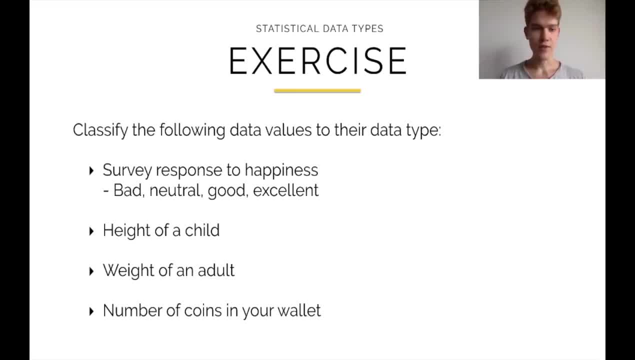 let's look at the number of coins in your wallet Again. we can already, by the name. it says number of coins. So we can probably agree that this is a numerical type of data. but the number of coins in your wallet? would that be discrete or continuous? 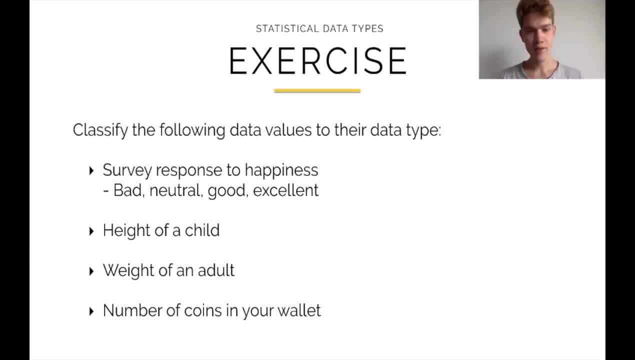 Well, the answer would be discrete, because it doesn't really matter what your coins are. They could be 50 cent pieces, they could be 25 cent pieces, 10 or 5 or 1s or anything you know, like a 2 or something like that. 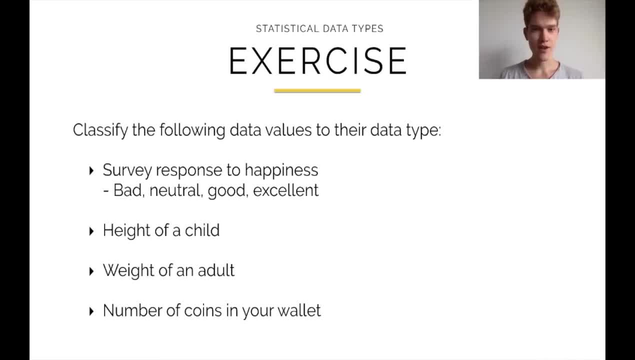 But they're not going to be, but the number of coins that you're going to have, we're going to sum up to a whole number, So you can have one coin, you can have two, you can have three, all of these things, but you can't have. 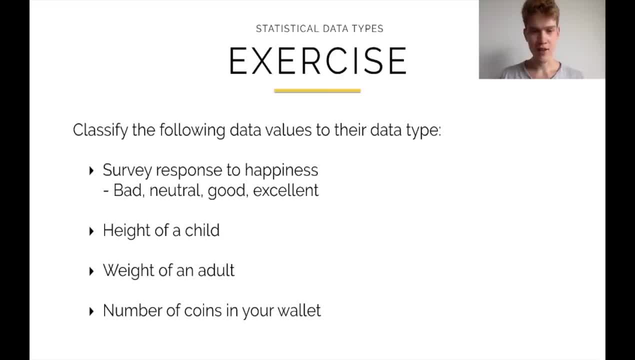 infinite fractions of a coin. You can't have, say, you know, the square root of two number of coins. That doesn't really make sense. So you have a defined step size, You have one coin, and then, if you have a second coin, then you have two. 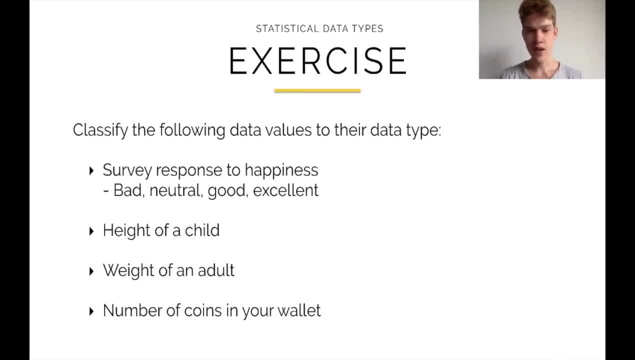 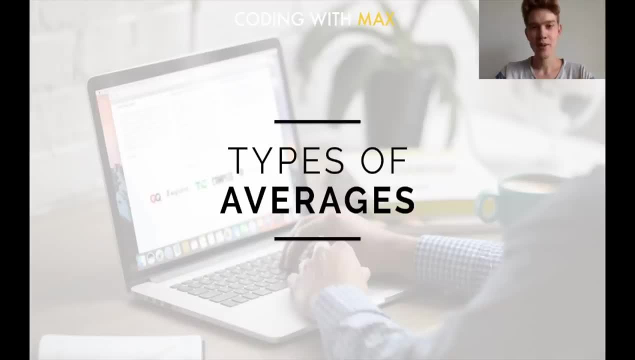 If you have a third coin, then you have three. You're going in step sizes of one, So for the number of coins in your wallet we'd be having discrete numerical data. In this tutorial we're going to talk about the different types of averages. 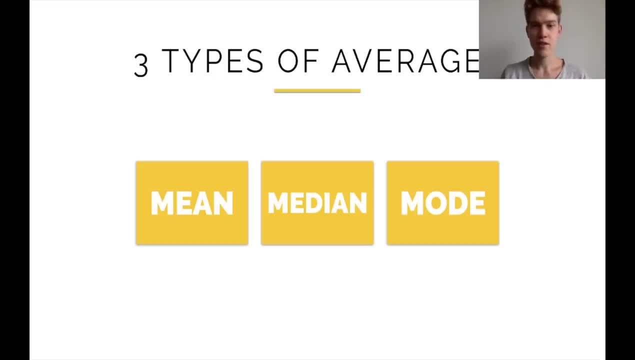 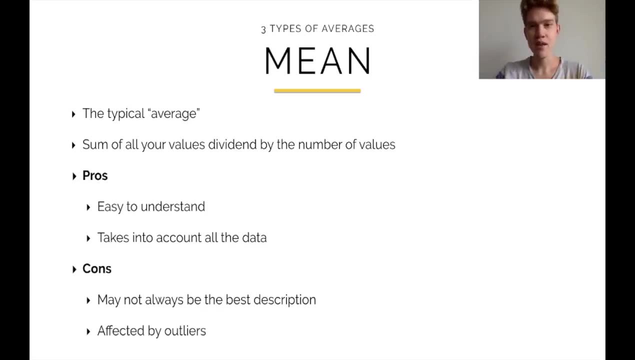 Now we're going to see the three different types of averages, which is the mean, the median and the mode. Alright, let's get started. So we'll start off with the mean Now. the mean is the typical average that you know. 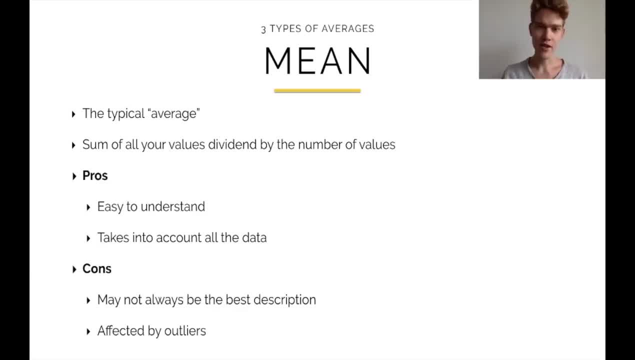 And really what the mean is is you just sum all of your values up and then you divide them by the total number of values that you have. Now, the great pros of the mean is that it's very easy to understand. It makes sense. We just have everything we have and we just kind of 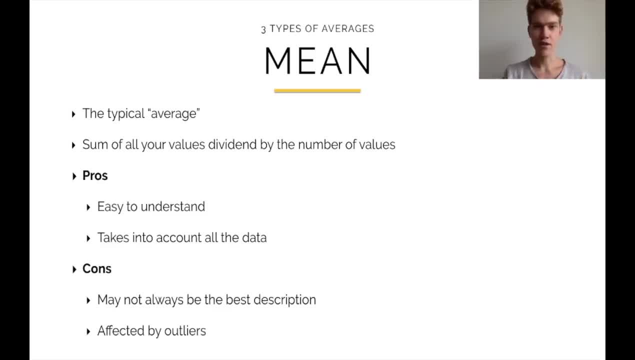 add that all up and then divide it by what we have, And that should give us a good representation of what is the average, And it also takes into account all of the data. So, since we're adding everything up and then dividing by how much data we have, we're taking into consideration every single data point. 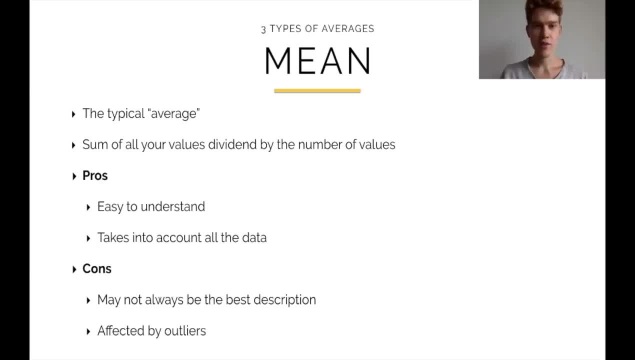 Now there are some problems with this. So one of the problems is that the mean may not always be the best description, and we'll see why when we look at examples for when we should use the median and the mode. And the mean is also very heavily affected by outliers. So, since we're 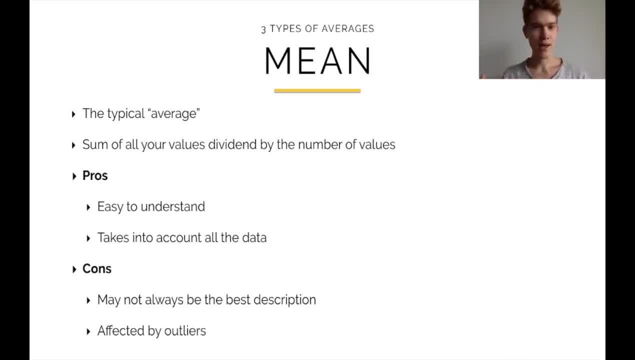 taking everything into consideration, if we have big outliers, that's really gonna change how our mean looks like. So if we just have normal values- you know between like 1 and 5, and all of a sudden we have like 10,000 in there, 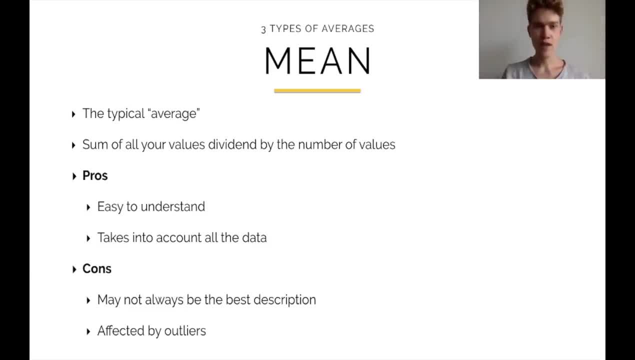 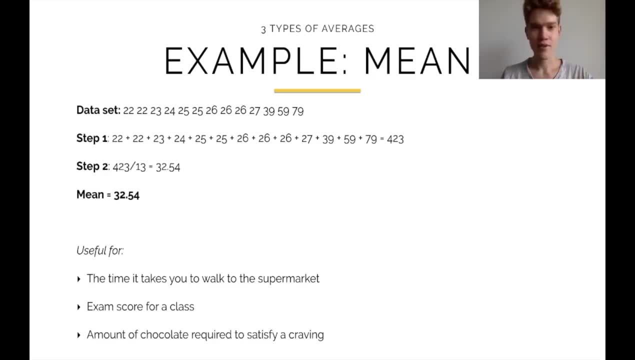 that's really gonna affect our mean. So the mean is heavily influenced by outliers, And the bigger the outlier, the more the mean is influenced by it. Alright, so let's see some examples of the mean. We'll go through a worked example first and we can see our data set here, which is just a bunch of numbers. 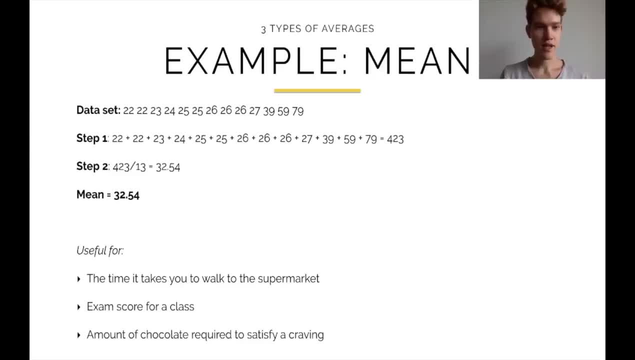 And what we're gonna do to calculate. the mean is we're just going to take every single one of these numbers and we're gonna add them up and we can see the total result that we get here. And then the next thing we're gonna do is we're gonna take this total result. 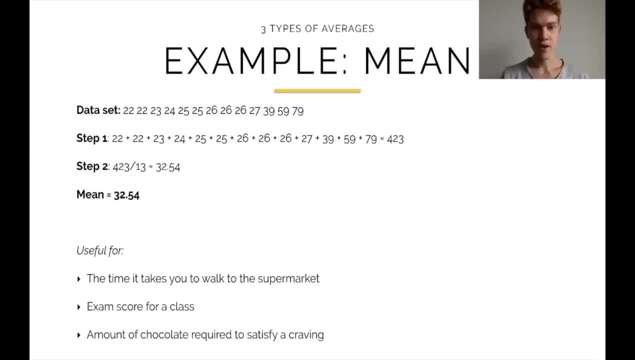 we're gonna count the amount of data points that we have and we're gonna divide one by the other, which then gives us our mean, as we can see here. So that's an example calculation of the mean. but let's see some example applications of the mean. 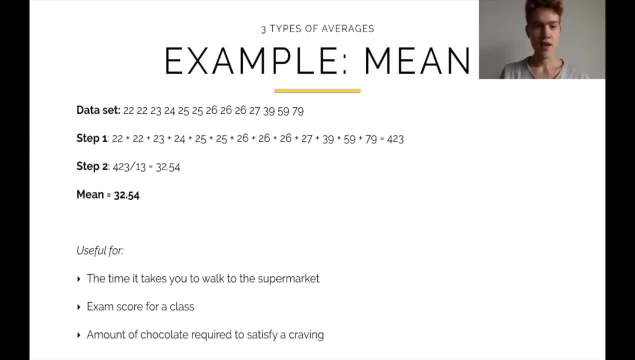 So when would we use it? Well, a good application would say: if you look at the time it takes you to walk to the supermarket. So sometimes you walk a little bit faster and maybe it takes you 20 minutes to get there. Sometimes you walk a little bit slower, it takes you 25, but on average it takes you somewhere like 22,. 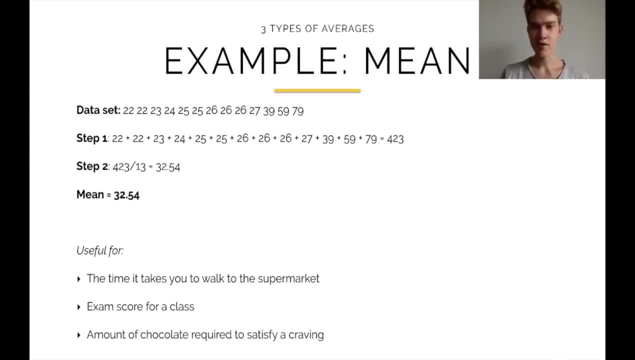 or maybe 22 and a half minutes or something like that. So if you say I'm gonna go to the supermarket, you're like it's gonna take me this much time to get there. Another good example of the mean would be exam score for a class. 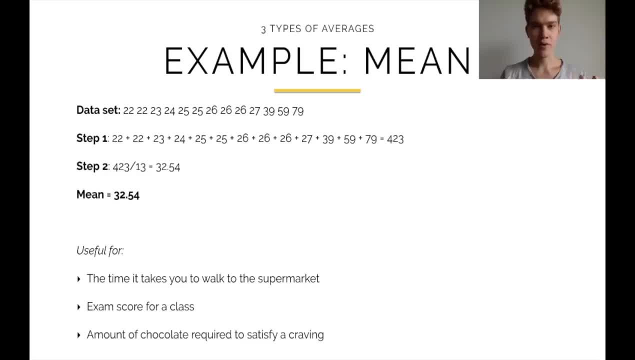 So to get a good understanding of how people do in an exam or in a class, you can look at the mean exam score last year And since our exam scores are kind of in a smaller range, a mean is going to be good to use. 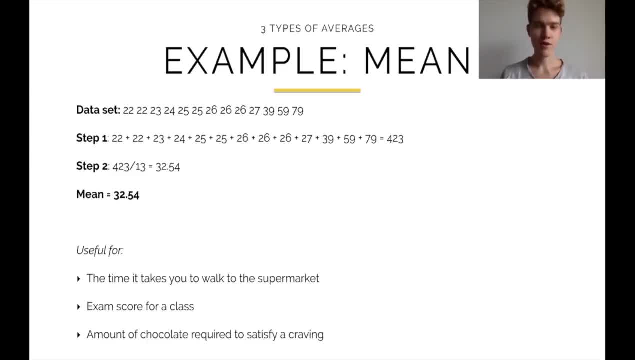 Because you can get anything between 0 and 100, but realistically speaking, no one's probably going to get a 0. So your range is even smaller and so you're less affected by outliers and you kind of know how hard a class is going to be just by being able to compare their means. 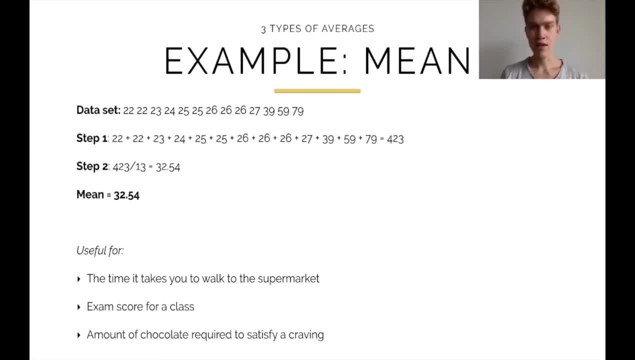 So if you look at one class and its mean is higher than the other, but they have a large number of students or something, then you can probably say, hey, it's easier to get a good grade here, or something like that. Or maybe you know some of these. 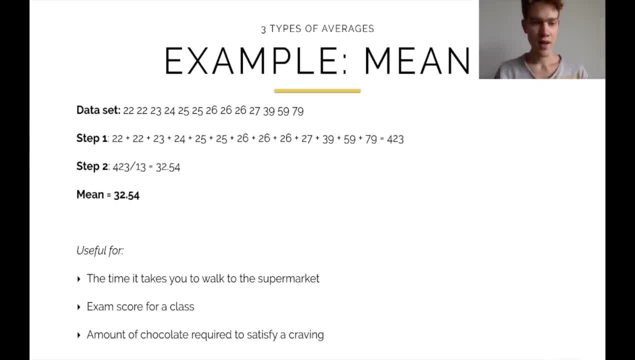 or simpler overviews, without diving too deep into it, All right. another good example of the mean would be to say: how much chocolate do you require when you get this kind of sweet craving, And you're not going to say like, oh you know, I require one chocolate bar. 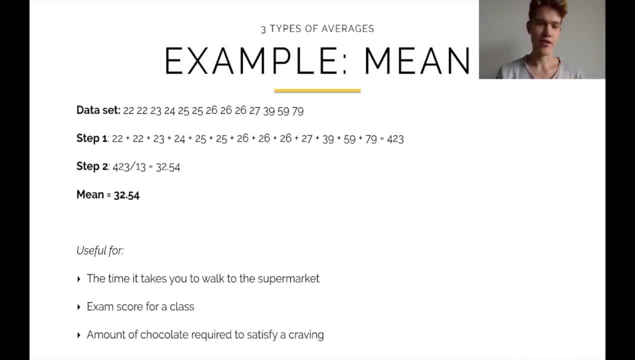 or two chocolate bars or three, But like you're going to say, oh, on average, you know, I require, you know, maybe three quarters of a chocolate bar, And sometimes I may want a little bit more because I feel like it. 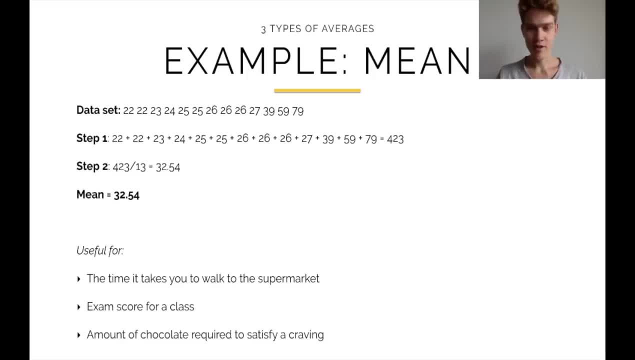 And when I start eating chocolate, I crave it even more. And sometimes, you know, I have it at first and like the taste just doesn't sit right with me right now, And so I have a little bit less. But these are kind of the amount of things. 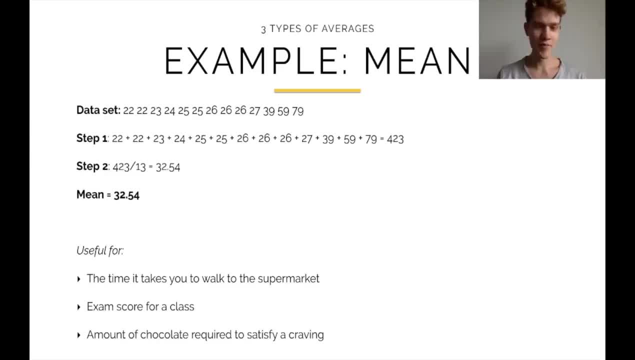 So, like, if you have this craving, you know, either you say, oh, I'm going to try to be strong, or you're like, hmm well, I know this feeling And I know if I eat about, you know, three quarters of a bar of chocolate or something. 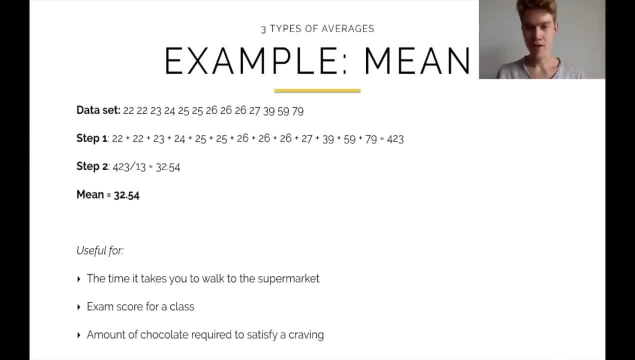 I'm going to feel good, My craving is going to be satisfied, So you kind of know what to expect. So these are some of the examples for how we would deal with a mean, or when we would use a mean. All right, 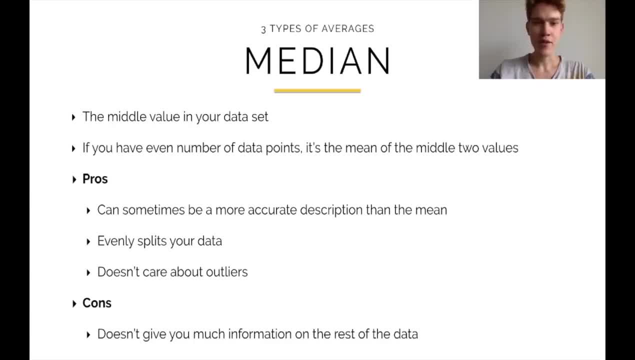 So let's look at the next thing, which is going to be the median. Now, the median represents the middle value in your data set. Now, if you have an even number of data points, you don't really have a middle value. 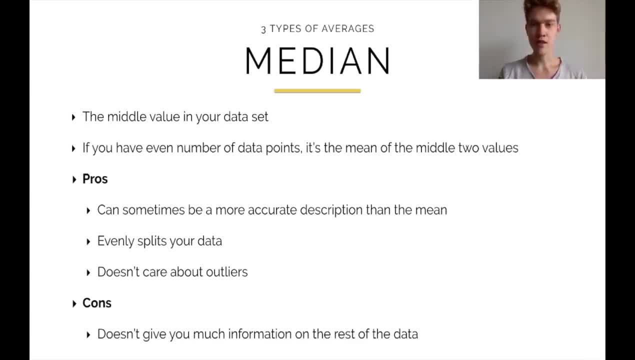 And so in that case the median is going to be the mean of the two values. So it's going to be the two median values added together and then divided by two. So the pros of using a median value is that the median can sometimes be more accurate than the mean. 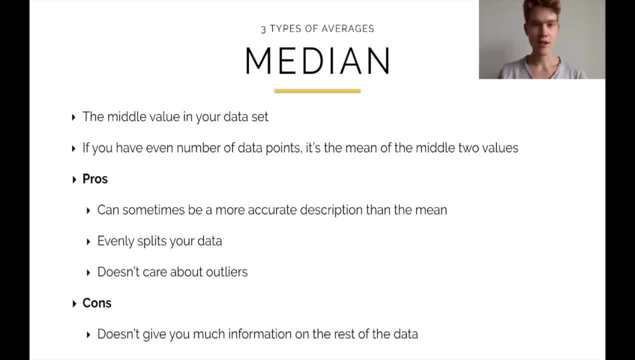 And we'll see some examples of this. The median also evenly splits your data. So you're not really, you know, affected by the mean in the sense that if you have an outlier in the mean and it drags everything to the right, it could be that your outlier drags things so far to the right. 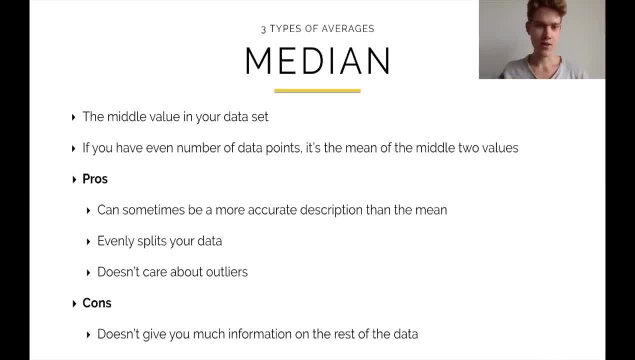 that all of your data is to the left of the mean and only the outliers to the right. So that would be an extreme case, but that can happen, Whereas the median, you know, it's always located directly in the center of your data. 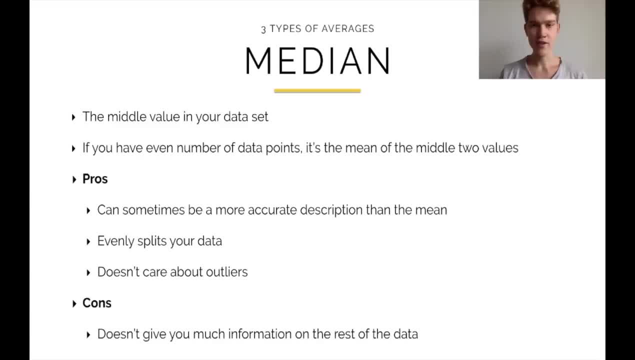 And the median also doesn't care about outliers. So if you have huge outliers at the beginning and at the end, it doesn't really care, because outliers by definition aren't very common, because they're outliers. And so if you have some at the beginning or have some at the end, 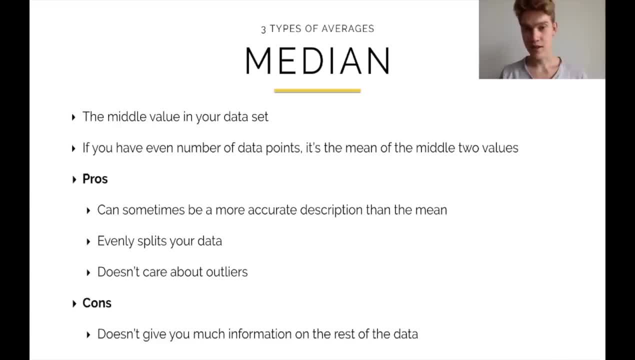 they're going to be very few in number, which makes them outliers, And therefore the median doesn't really care about outliers that much. A con, though, is that the median doesn't really give you much information on the rest of the data. 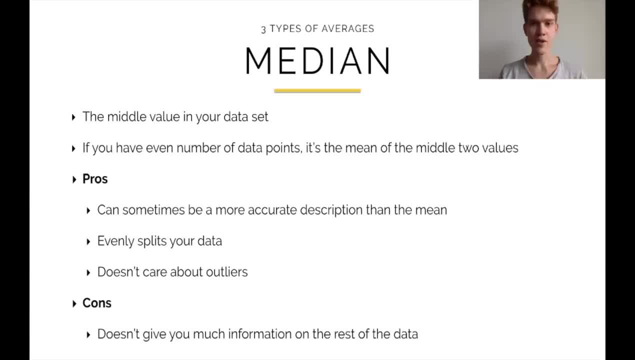 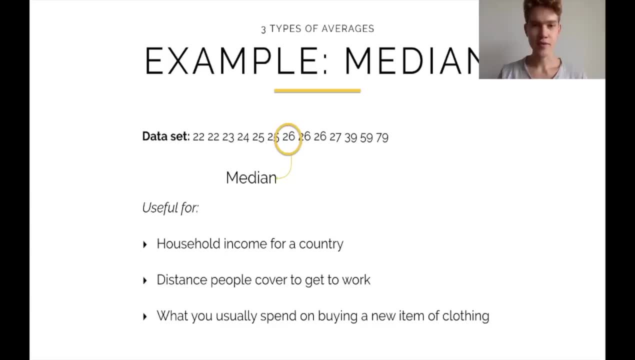 Sure, you know. you know what's at the center, but you don't know how does everything arrive, How does everything around me behave? You only know where is the center of our data. So let's see some examples. We'll do a worked example first, where we see our data set here. 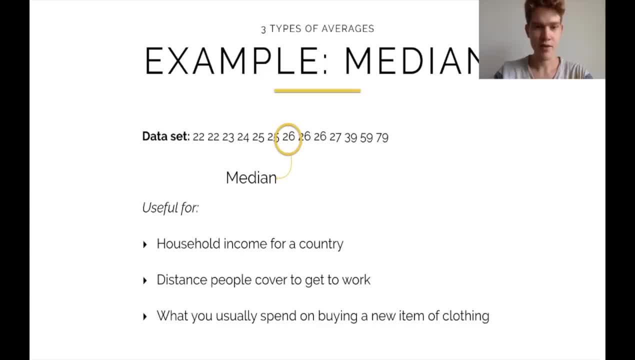 And we can count how many values we have. If we go from left to right, then we can say we've got 1,, 2,, 3,, 4,, 5,, 6,, 7,, 8,, 9,, 10,, 11,, 12, and 13 data points. 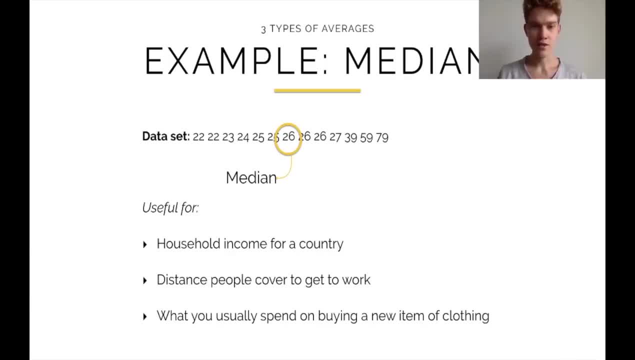 So we've got an odd number And so our median value, our center value, is going to be the seventh data point, because it's 6 from the beginning and it's also 6 from the end, So it's equally spaced both from the beginning and from the end. 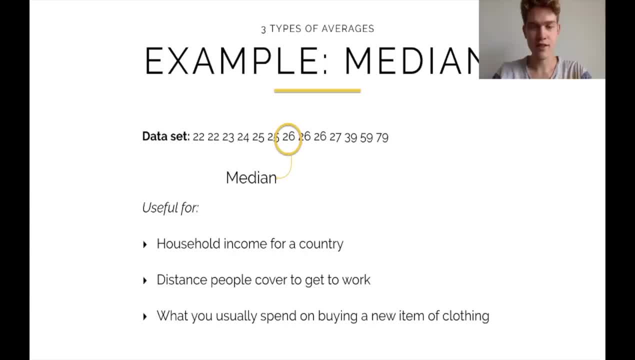 And so that's why we see our median value here is 26.. It's located directly in the center. Now, what is the median useful for? Well, the median is often used. if you look at, you know, household incomes for a country. 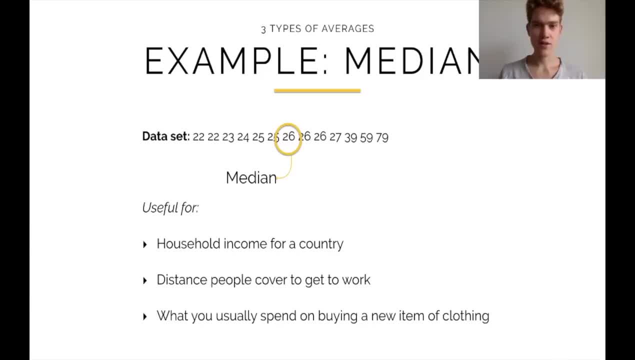 Because if you were to use the mean, then these billionaires, they would just completely you know, they would give you a false description of what really an average household income is, Because normally if you have, you know, like an average value and you can say: 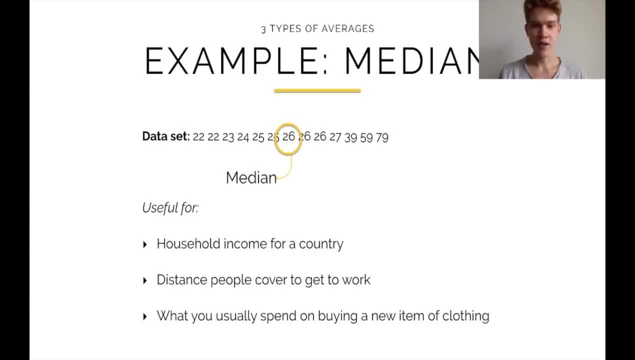 oh, the average household income from this family would be, say, $40,000 or something like that, Or that would be the median value, But if you were to use the mean instead, then all of the billionaires and all the millionaires in the country. 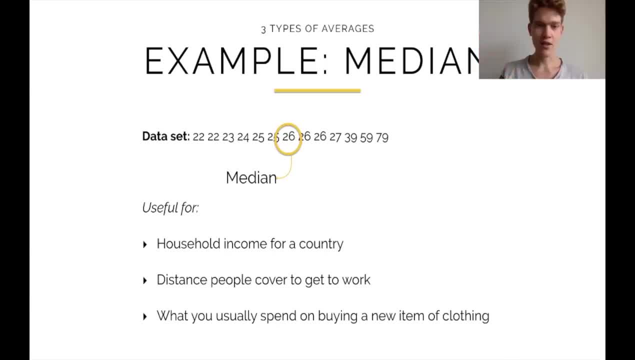 they would change that household income And then you would say: oh you know, the average household income per family would look like, say, $60,000. And that's a bad representation because that doesn't actually give you a realistic look. 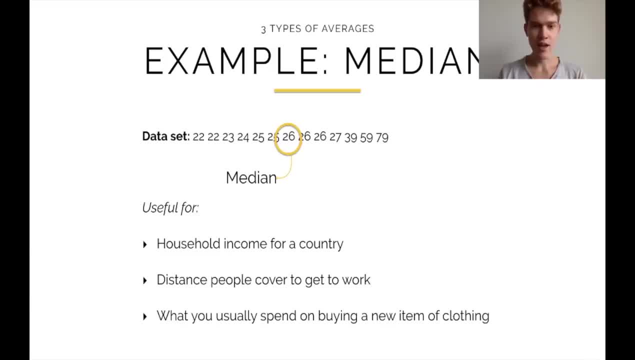 at what the average household family has. And the average household family really does. It's, you know, centered at like $40,000. And sure, there are people below and there are people behind, But that's what's in the middle. 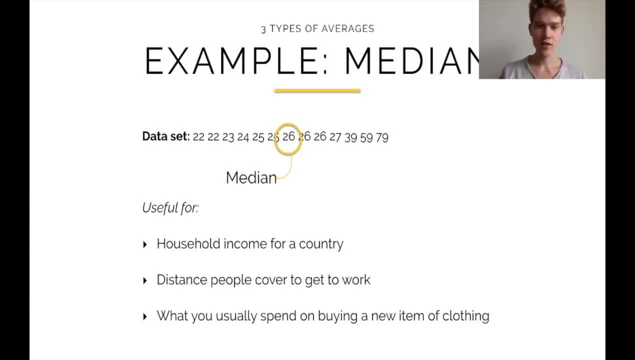 Whereas if you were to use the mean instead for your average, you would kind of get this inflated household income which wouldn't be representative to the rest of the country. Another good example of the median would be the distance that people cover to get to work. 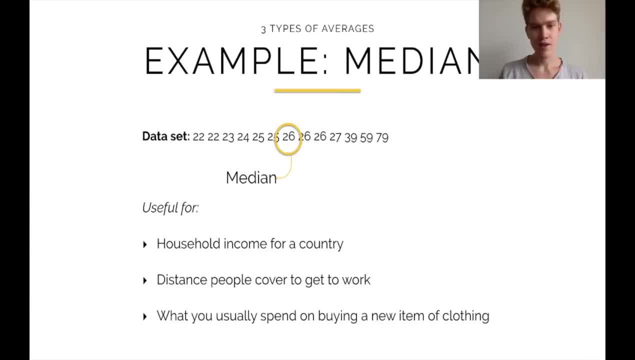 So if you look at this in terms of you know kilometers, then you can say like: oh, you know some people. they walk to work and it's like you know one kilometer at most, So something like that. 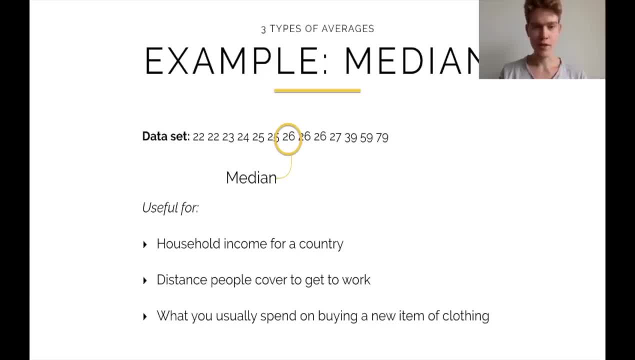 And then you can expect people to travel. Most people travel around three kilometers to work And sure there are some, you know, that travel much further because they want to live outside of the city And there are some that travel very, very short distances. 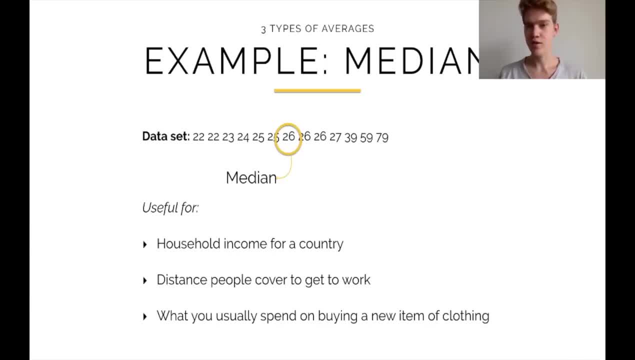 because they have a house right next to the office, where their house is the office or something like that, depending on where you're working. But then you can look at. you know, like, where in the middle, how do people travel to work? 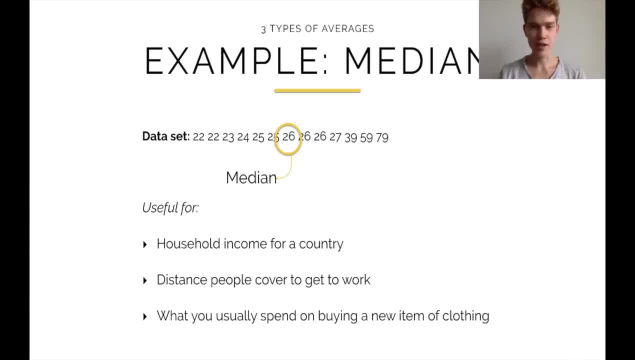 What time or what distance do they need to cover, And so that would be another good use of the median. Another good median value is: what do you usually spend when you buy a new item of clothing? And so sure you know, sometimes you may go to that expensive clothing store. 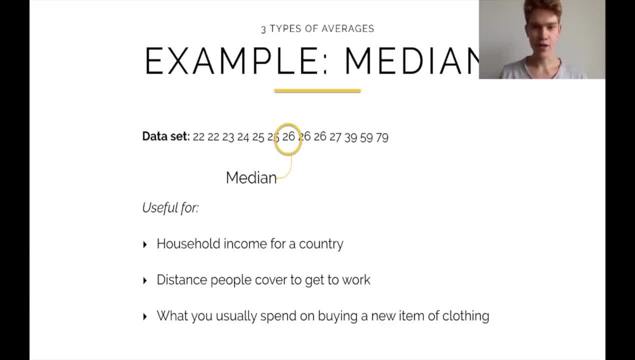 and you could get a jacket that costs I don't know, north of a couple hundred euros or dollars, whatever system you want to use, And sometimes you can go to a secondhand store and get it for very cheap. But usually if you go into stores, a jacket would- I don't know- maybe cost you like $100 or something like that. 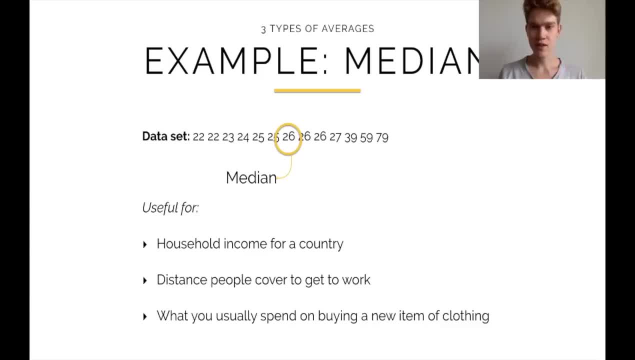 And so you know if you go out you can expect to pay about $100.. No, not really you know, taking that much account into what store you're going into. So most of the stores that you're going to visit, 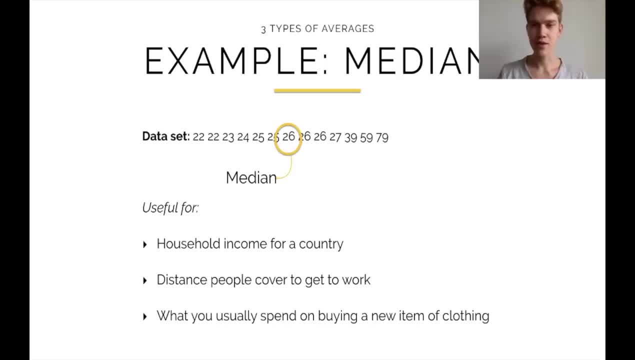 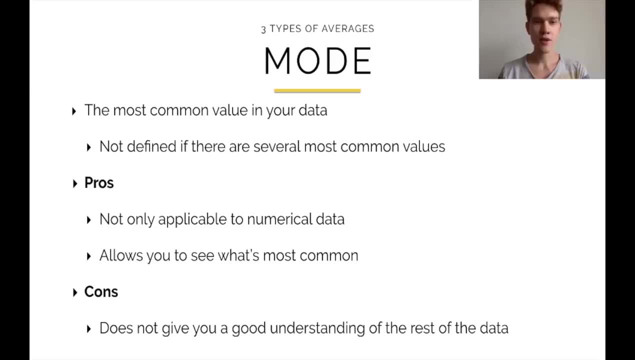 are going to have that price for the jacket, So that would be another good use for the median. All right, let's look at the third type of average that we can do, which is the mode. Now, the mode looks at the most common value in your data. 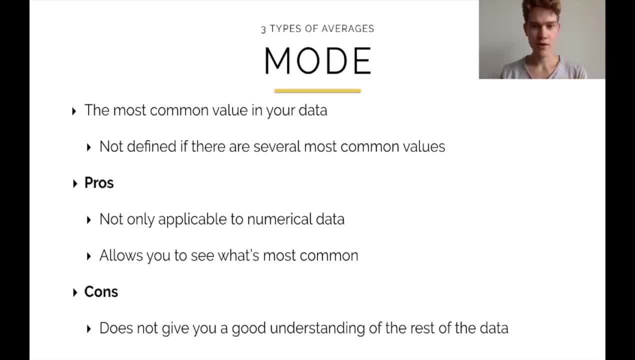 And it's not really defined if there are several most common values, but if there's only one most occurring value, then that's what your mode would be, And so we'll see an example of this in a second too. The pros of using the mode is that it's not only applicable to numerical data. 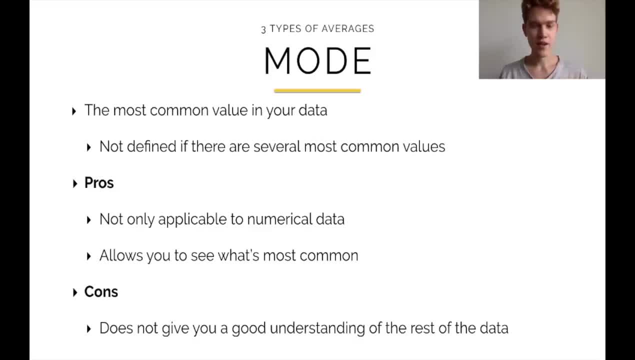 so if you look at categories, for example, then you can say: hey, we've got five people from the US, you know, and two from Canada and one from France, And you know that the mode is going to be the US. 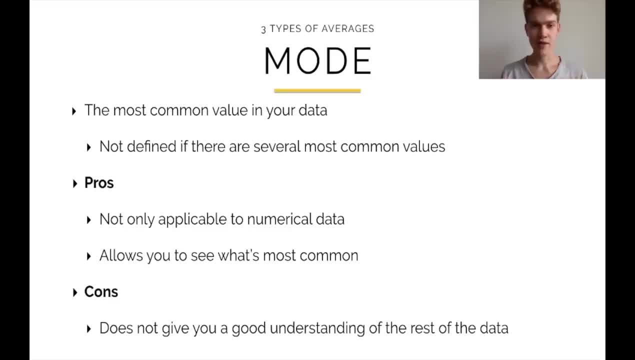 because there are five people from the US. So mode is the great average. that's not only applicable to numerical data in this sense, but you can technically also apply it to categories or to ordinal numbers if you wanted, so that you can say the most common country. 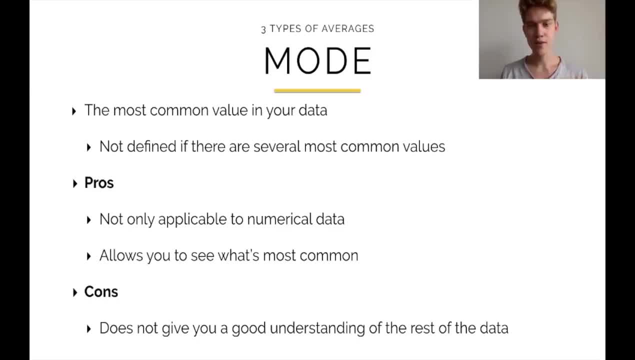 that we have, or the average kind of country that we would expect here, is the US. And sure, there are other countries, but the average or the most common one is going to be the US in this case. So yeah, and then, of course, 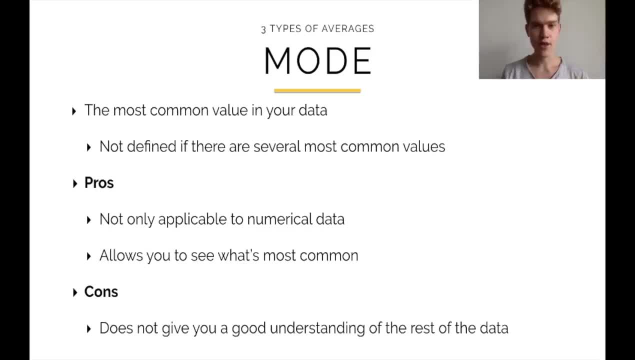 the other pro is that we allow to see what's most common, what pops up the most. So that's a great use of the mode if there are cases when you know recurring values happen a lot, which is the case for discrete numbers, for example. 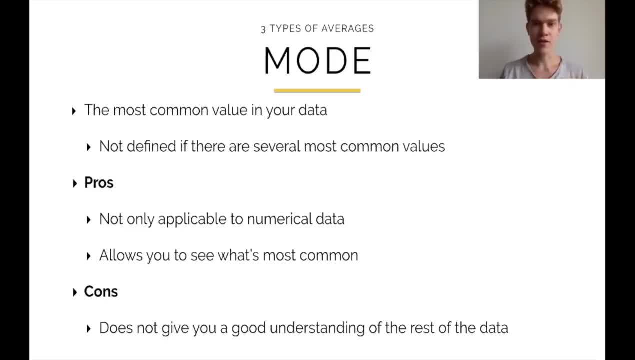 So in discrete numbers, values reoccur often, and so it's good to use the mode. A con of the mode is going to be that it doesn't really again give you a good understanding of the rest of the data, similar to what we had for the median. 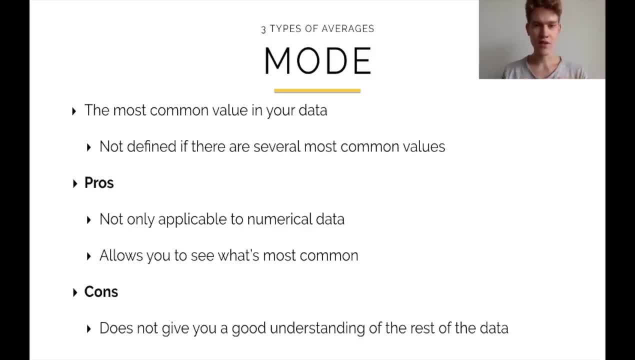 But also it's not really applicable. if you just have a bunch of different types of data, then there isn't really going to be a mode. If there's not enough of each data, it's not really good to use the mode. You don't want to. you know, have thousands of data points. 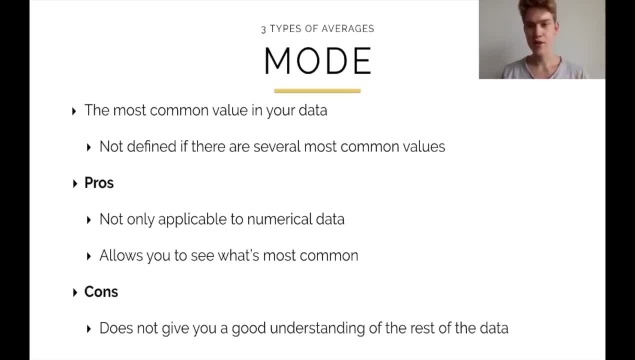 and the most reoccurring value reoccurs like three times. That's not good. You want to use the mode for situations where data reoccurs often, So, like we saw the country example, But let's actually see a worked example. 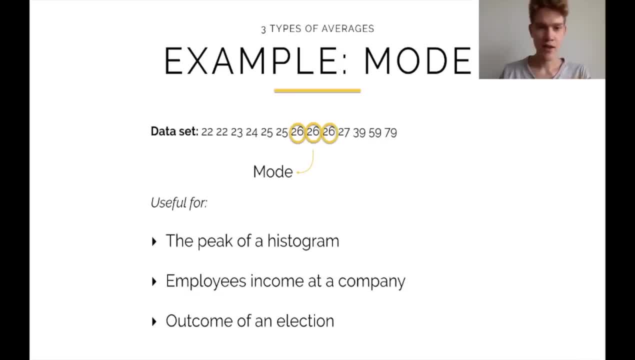 but also some other examples for the mode. So the worked example here would be: again, we take our data set and we can count how many times different numbers appear, And so if we go through the numbers, we'll see that 26 occurs the most. 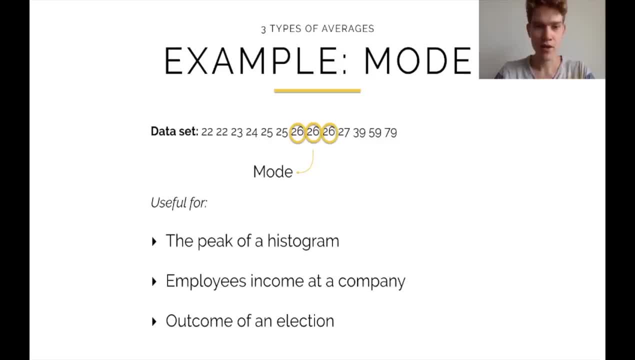 And so that's going to be our mode here. So we've got 22 and 25 that both occur twice, but 26 occurs three times, And so 26 is going to be our mode, It's going to be our most occurring value. 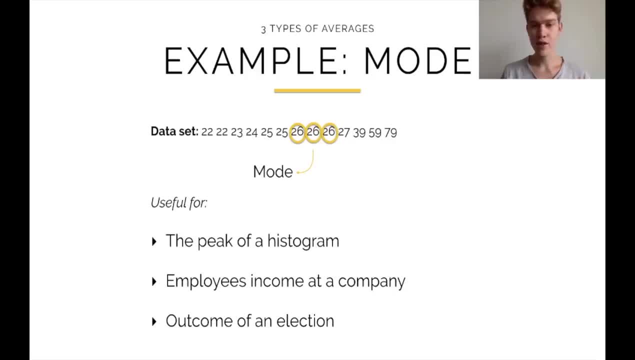 Now the mode is going to be useful for things like the peak of a histogram. So if you draw this histogram and if you don't know what a histogram is, don't worry, We'll cover that in a later lecture too. 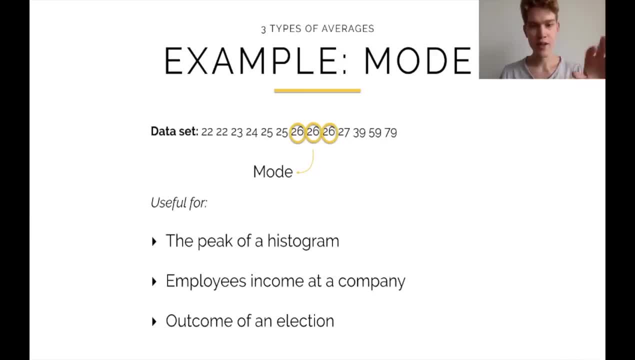 when we go into data visualization, But the peak of a histogram that's going to show you the mode of the data, The most occurring data. Another use of the mode would be if you look at employee income at a company, Because at a company, you can again have the boss, which takes off the mean, and you can have higher level employees too, which would kind of shift the median. But if one third of your employees earn minimum wage, then that's going to be the best average. 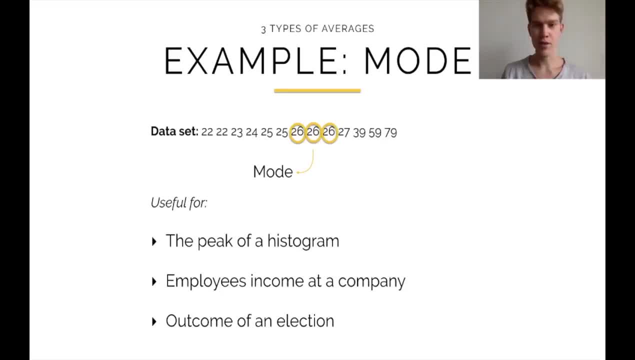 Or say, if 40% of your employees earn minimum wage- or probably not your employees, because that wouldn't be a very good system to have- but if 40% of the employees at the company that you're looking at earn minimum wage. 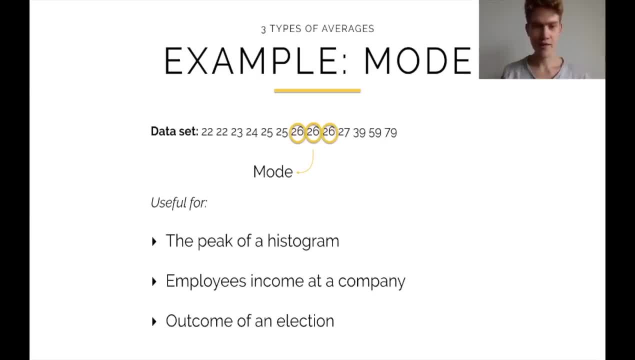 that's not a really good thing to have, And if you look at the mode, you'll easily see that the average in this case would be to earn minimum wage, because that's what most people earn, And sure the boss or the CEO or something. 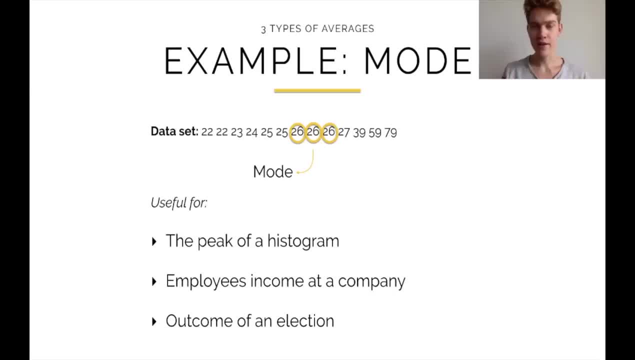 he may shift the mean up heavily. and then the fact that you have higher ups. if you look at the median value, you may even well be too far to the right that you really don't consider these employees that all earn the same amount. 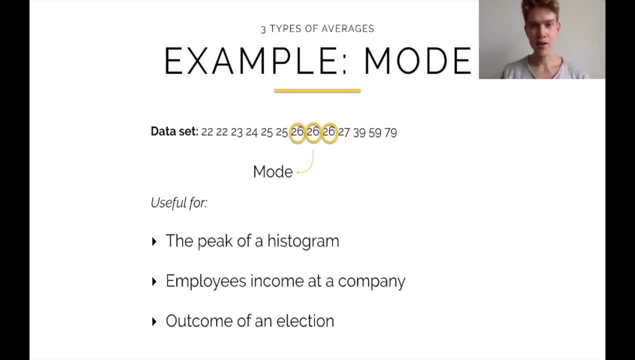 But you really want to get that description, which is what you get here from the mode, And then also the outcome of an election is where you use the mode for and sure. sometimes you may only have two values, sometimes you may have three. 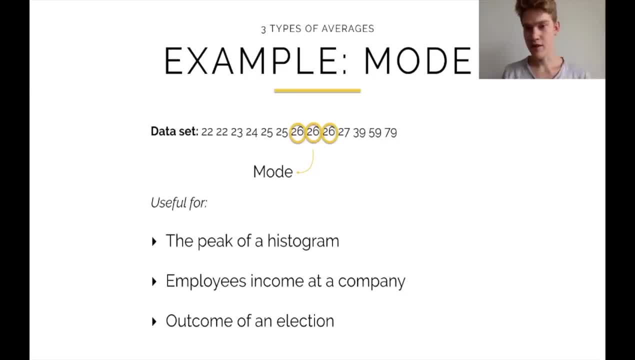 but if you have different candidates, and say you have five different candidates, then the person with the most votes is going to win the election because they have the most. So there again you'll use the mode. In this lecture we're going to look at spread of data. 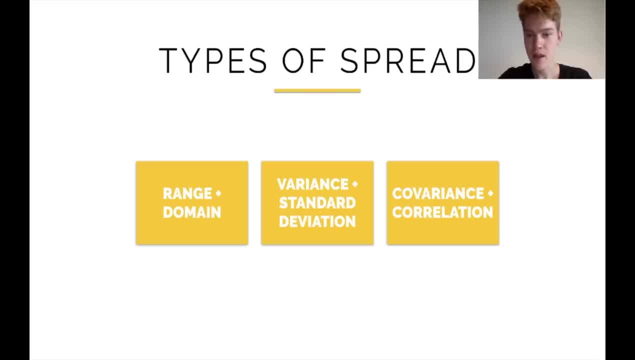 And we're going to start off with looking at the terms range and domain, then we're going to move on to understanding what variance and standard deviation means and then, finally, we'll look at covariance as well as correlation. Alright, so let's start off with the range and domain. 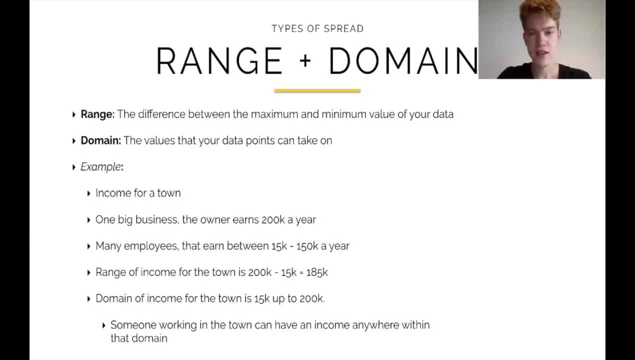 Now let's start off with the range. So the range is basically the difference between the maximum and the minimum value in our data set. It's kind of simple to think about, So let's just kind of go through this with a worked example. 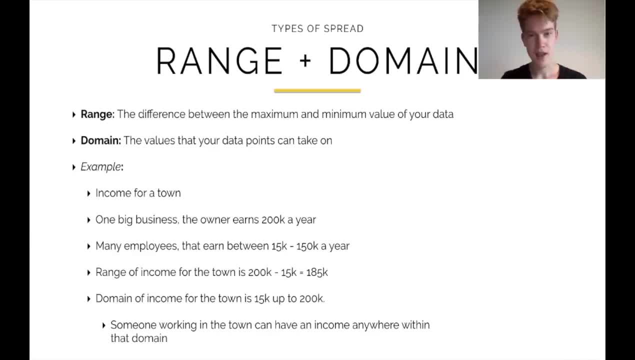 Let's set up a company in a town and this is the only company in the town and the owner of the company earns a salary of 200k a year. and then the employees. you know they all have different salaries, but the lowest employees. 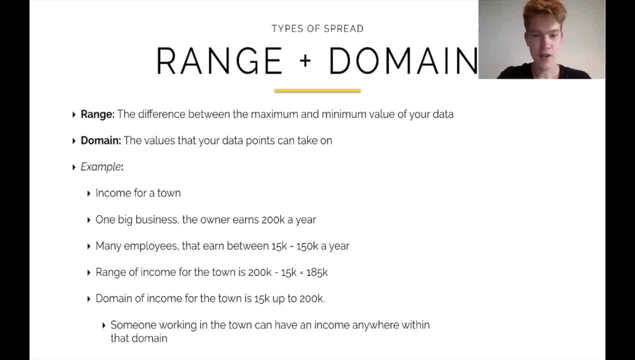 or maybe the part-time workers. they earn something like 50k a year. So we've got data kind of ranging from 15k up to 200k, And so our range is the difference between the maximum and the minimum value in our data. 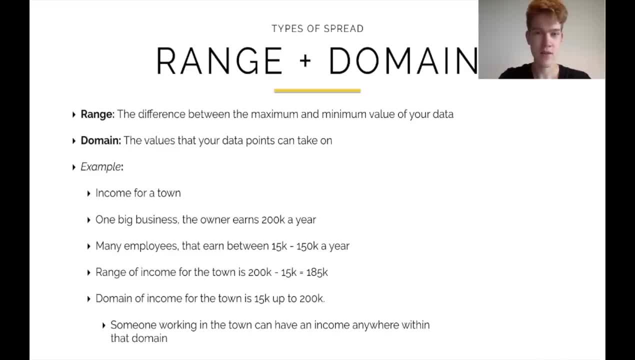 So we take 200k and we subtract 15k from it and we've got a range of 185k in salary. So that's how big our salary can change. So if we start at 15k it can go all the way up to 200k. 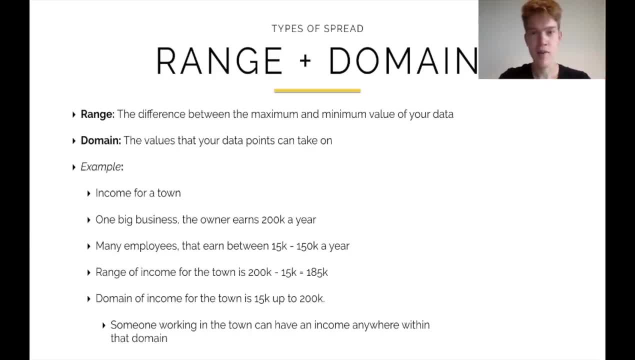 So that's a 185k range of salary that people in this company can have, Alright, and the domain is going to be the values that our data points can take on or the region that our data points lie in. So if we look at this example again, 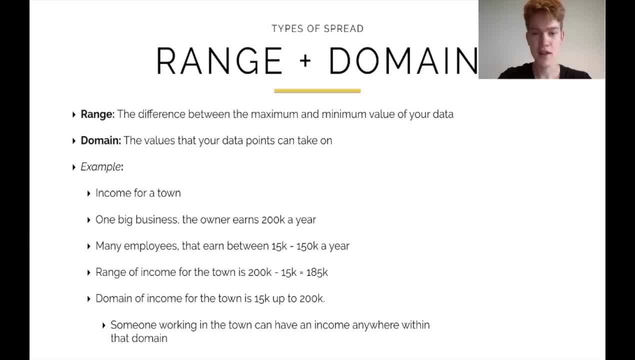 our domain is going to start at 15k and go up to 200k. So what the domain defines is it defines kind of starting and ending points, or it defines a section in our data, And so in this case the domain would define: you know, 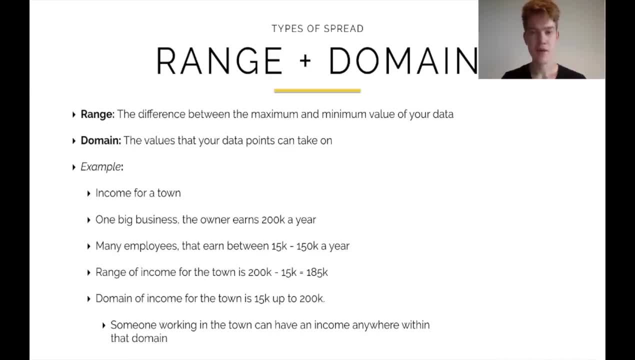 it would start at 15k and it would end at 200k, And what the domain tells us is that everything or all salaries within you know between 15k and 200k, that they're possible, but within this domain. 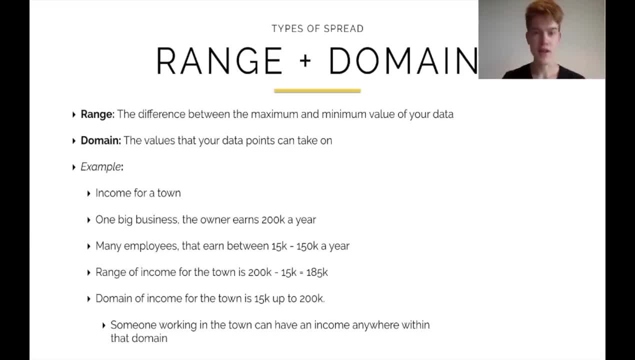 or within this company. it's not possible to have salaries outside of this domain. So if our domain again is 15k to 200k, then we can't have a salary of 14k because that's outside of our domain, And we also can't have a salary of 205k. 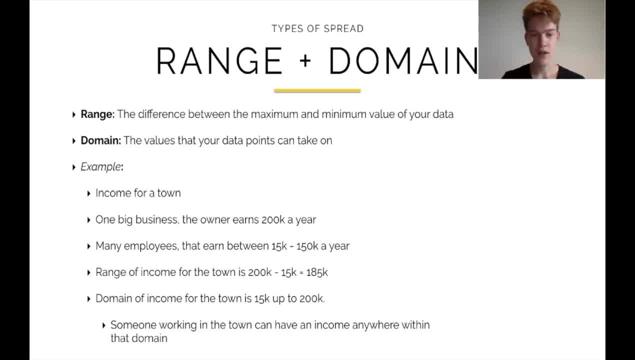 because, again, that's outside of our domain. So pretty much all salaries within 15 to 200k are possible. Anything outside of the domain is not possible because that's no longer in our domain. All right, so let's move on. 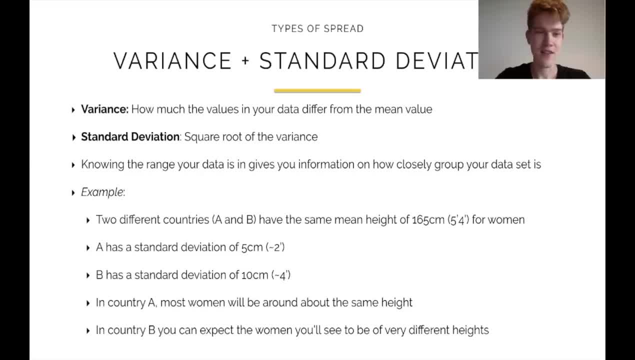 and look at the variance and standard deviation, And we'll talk about the variance first And what the variance tells us. it pretty much tells us how much our data differs from the mean value And it looks at each mean value and it looks at how different each value is. 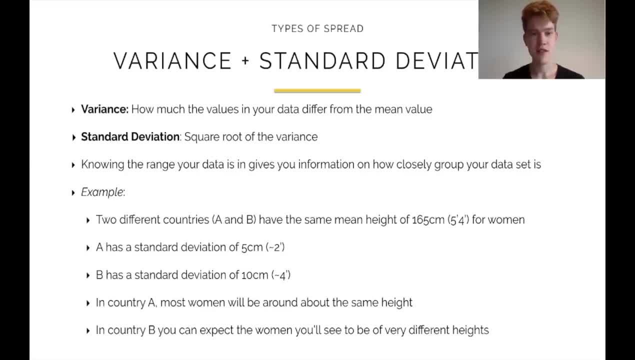 from the mean value And then it gives us the variance. It does some calculation and we don't really need to know the formula. It's more important right now just to understand the concept of variance. And so what variance really tells us is it tells us how much our data can fluctuate. 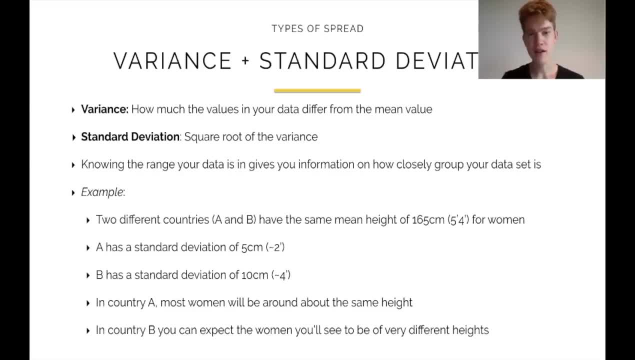 So if we have a high variance, that means a lot of our values differ greatly from the mean value and that will make our variance bigger. If we have a low variance, that means a lot of our values are very close to the mean value. 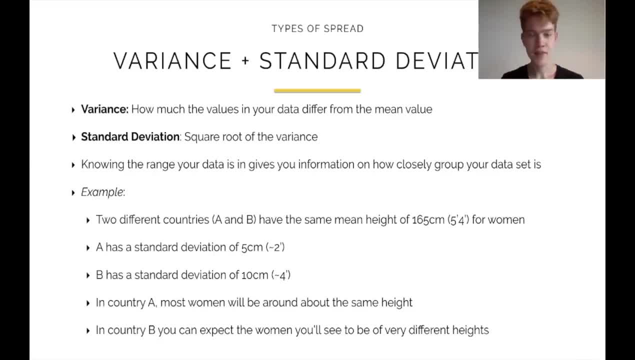 And so that will make our variance lower. And now, if we turn to the standard deviation, the standard deviation is literally just the square root of the variance. So if you understand one, then you also understand the other, And now we can combine this. 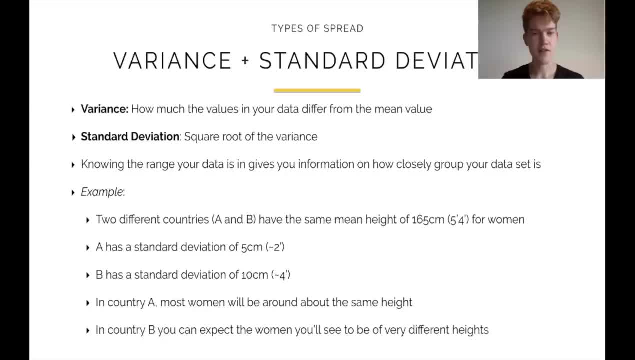 if we know the range of our data, to kind of get a better feel for our data. And so let's use an example where we have two different countries, just countries A and B, and they have the same mean height for women, which in this case we'll say: 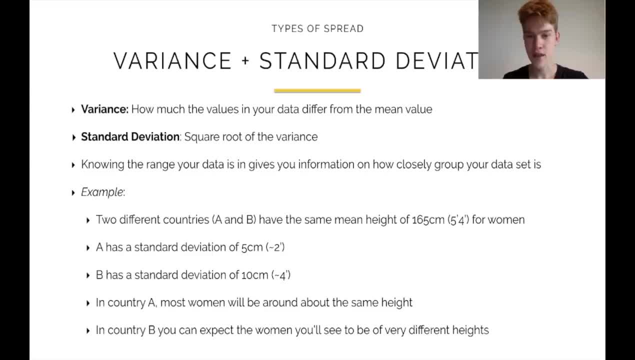 is 165 centimeters or 5 feet 4.. And we'll say that the range of heights for them could be identical. So let's say they can range. you know the range. let's say could be like 30 centimeters or something. 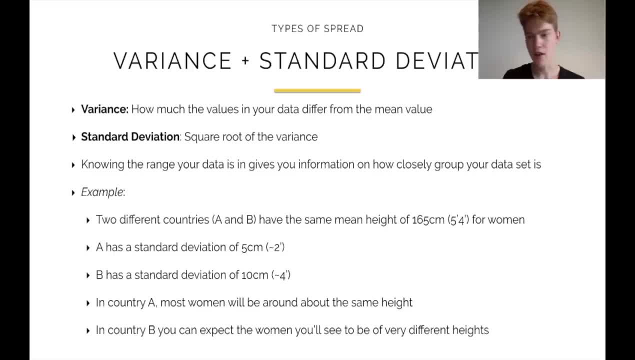 It can go anywhere from, say, 150 all the way up to 80, or we can even increase that and say, like, anywhere from as low as 140 up to like 2 meters or something like that. But let's just keep the range. 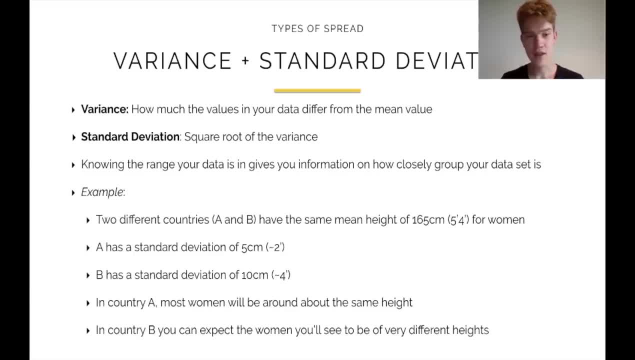 for these the same And they both have the mean height. So if country A has a standard deviation of 5 centimeters, which is approximately 2 inches, and country B has a standard deviation of 10 centimeters, which is approximately 4 inches, 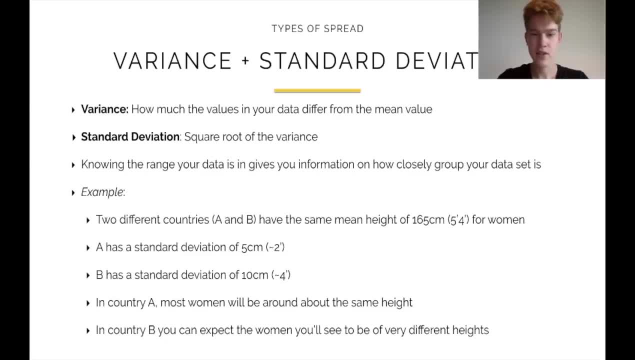 then what you can expect, knowing these values, is that if you go into country A, the people that you're going to see are going to be much more similar in height. So our standard deviation is lower. That means our values differ lower from the mean. 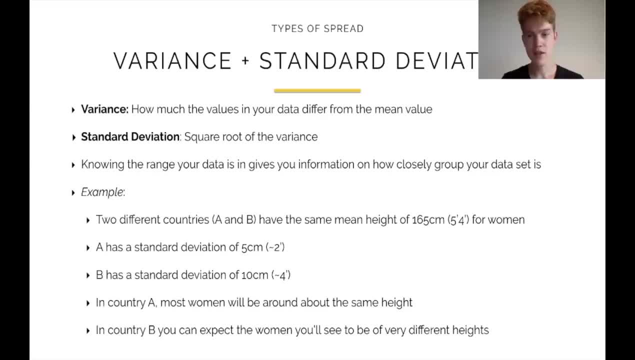 And so that means a lot of the women that you're going to see are going to be very close to 165 centimeters, or 5 feet 4 plus minus 2 inches. So what you can expect when you go to this country is that everyone is going to be. 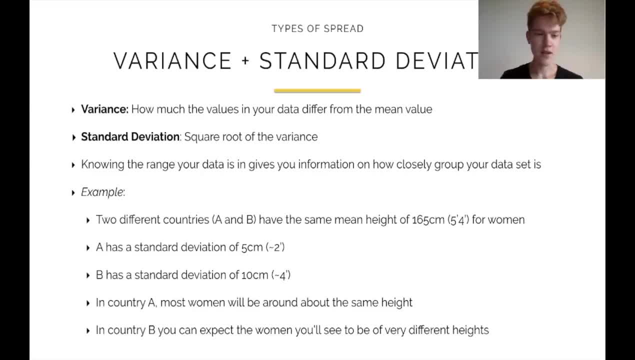 or a lot of the women, are going to be about that height, Whereas if you go to country B, they have a much larger standard deviation, And so you can't really expect everyone to be about 5'4", because it fluctuates a lot more. 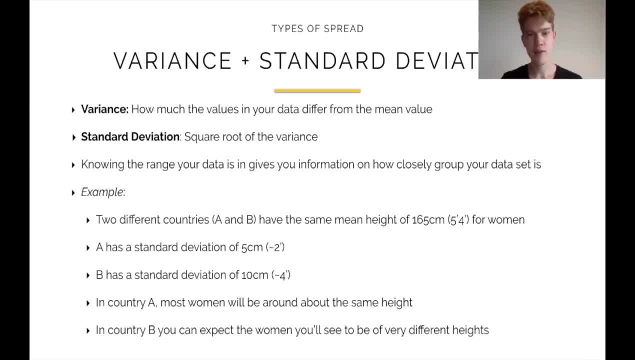 And so if you go to that country, you can expect to see a lot more women of different heights, both taller and shorter than 5'4". All right, And so that's how we can kind of use the variance and the standard deviation. 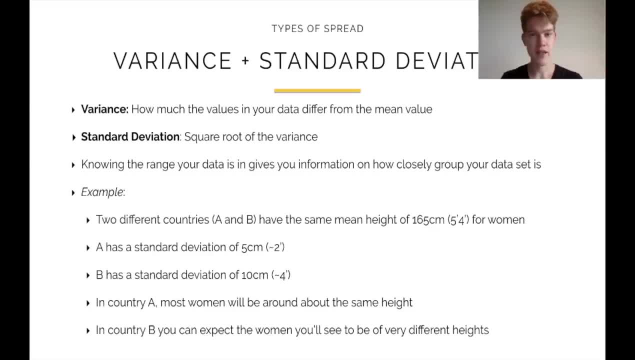 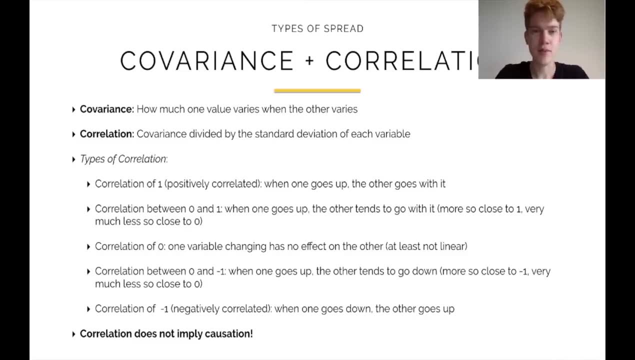 or the standard deviation, to give us a little bit more perspective on our data and kind of allow us to infer some stuff about our data. All right, So let's talk about covariance and correlation. So covariance will or already has the name variance in it. 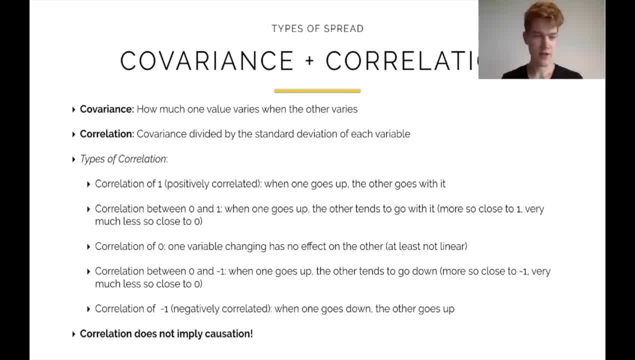 but covariance is measured between two different variables And it pretty much measures if you have two variables. So let's say we've got me drinking coffee in the morning and my general tiredness. So if I use these two values and get data points, 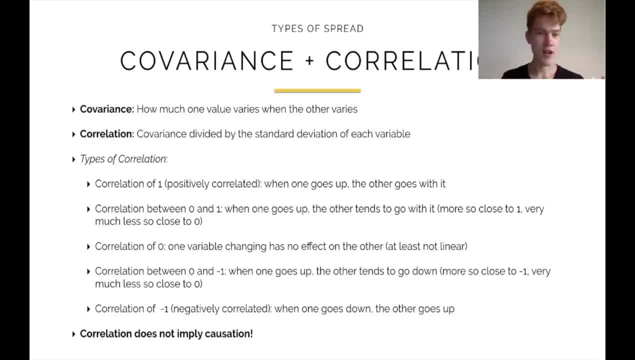 oh, this is how much coffee I drank in the morning And this is how tired I feel this morning, or something like that. And so what the covariance does is it looks at how much one of these values differs or changes when I change the other one. 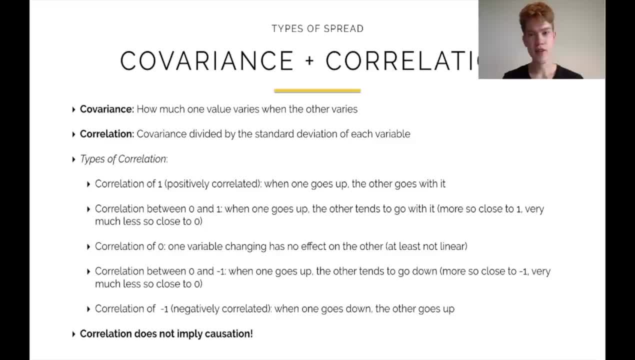 So what does that mean, for example, Well, if I drink more coffee, what the covariance would look at is how much does my tiredness change? So that's what you do with covariance. You see, you say I change one, How much does that affect? 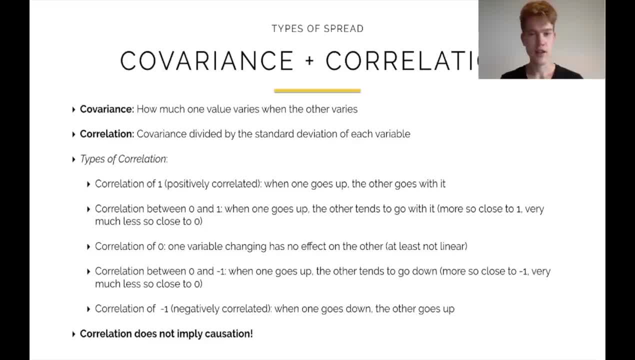 the other thing that I look at And our correlation is very similar to covariance. So we kind of normalize the covariance by dividing by the standard deviation of each variable. So what that means is we get the covariance for my drinking coffee versus feeling tired. 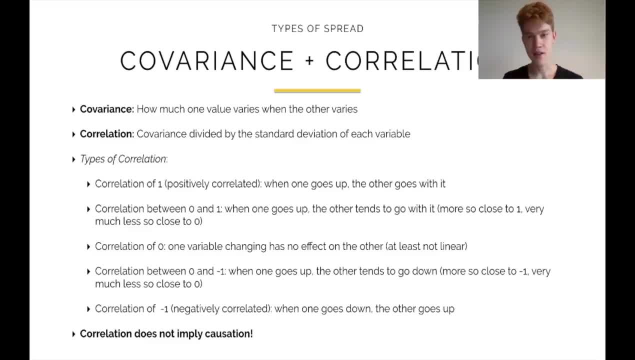 And then we would just divide by the standard deviation of me drinking coffee and the standard deviation of me feeling tired. And so really, what we're doing with the correlation is we're just kind of bringing it down to relative terms that would fit our data better. 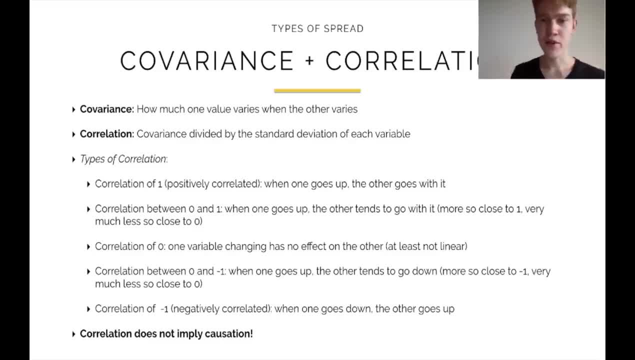 So that's kind of the abstract idea. The important thing to just keep in mind is that we're looking at one and we're seeing how much that changes, And we're seeing how much that change affects the other one. All right, So there are different types of correlation values. 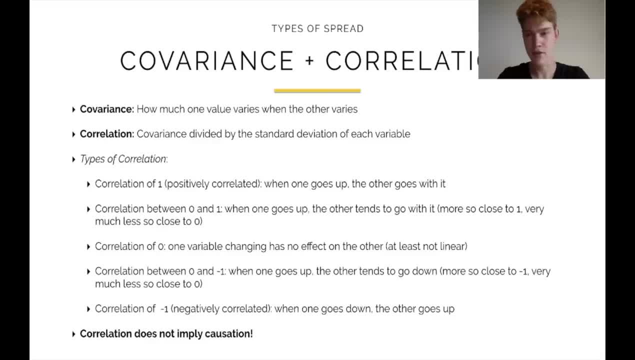 that we can have, and they can range anywhere between negative one and one Or so. their domain is between negative one and one, And a correlation of one means a perfect positive correlation. So that means when one variable goes up, the other goes up. 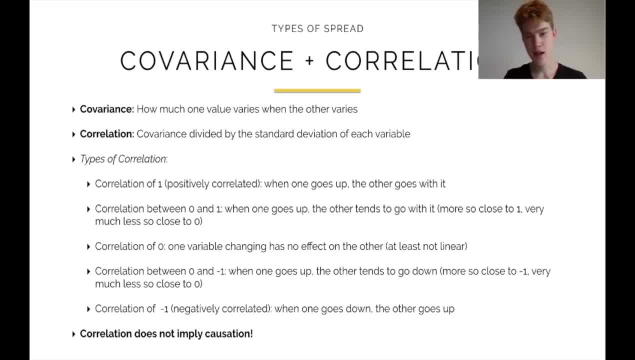 So for my coffee example that would be: if I have coffee in the morning, then I also feel more happy. So the more coffee I have, the more happy I feel, And of course there's going to be a limit. But let's say I only drink up to two cups of coffee. 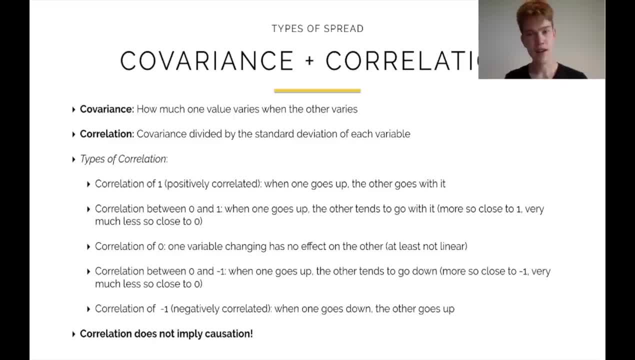 or something like that, and I can drink anything in between, And the more I have, the more happy I am about it. So that would be a positive correlation. The more I have of coffee, the more I have of happiness, And so they would kind of go up together. 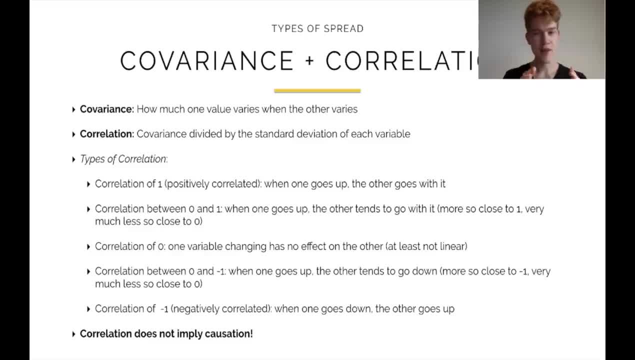 And then when we get closer to zero, the zero point is going to mean no correlation to us. So anything between zero and one is going to be a kind of slightly positive correlation. It's not going to be a super strong And we'll actually see some examples on the next slide. 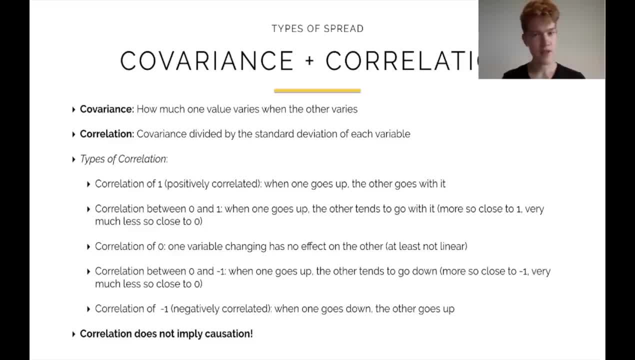 But yeah. so anything between zero and one is going to be a kind of slight positive correlation, not super strong, And the closer you get to zero, the more it means no correlation. So an example for the zero case would be that it doesn't matter how much coffee I drink in the morning. it's not going to affect the weather. They're unrelated. One does not affect the other. So I could drink, you know, one cup of coffee during a sunny day and one cup of coffee during a rainy day, and it's not going to change the weather. 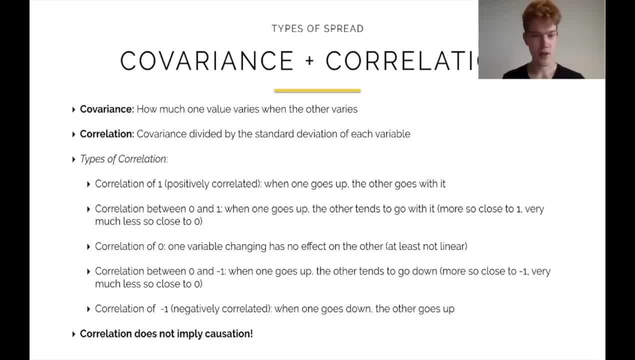 It's not going to affect the weather, So they're pretty much uncorrelated. And then we can also go down into the negative range, And so the closer we get to negative one, or, if we reach exactly negative one, a correlation of negative one. 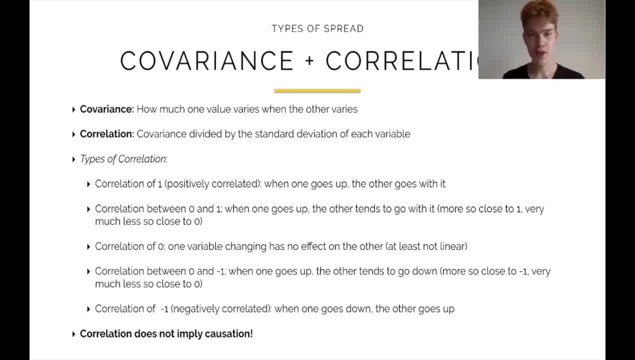 means a perfectly negative correlation. And so here we can take our example of coffee versus tiredness. And so the more coffee I have, the less tired I'm going to be. So coffee goes up and tiredness goes down. So that's how we can kind of understand this correlation. 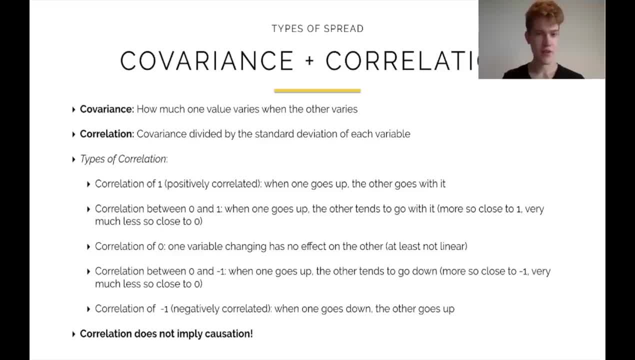 And it comes from the covariance. So it was important to understand the covariance. We usually use the correlation, because the correlation, because we divided by the standard deviation of each, is much better fit to our data. Now there is one thing that's very important to remember. 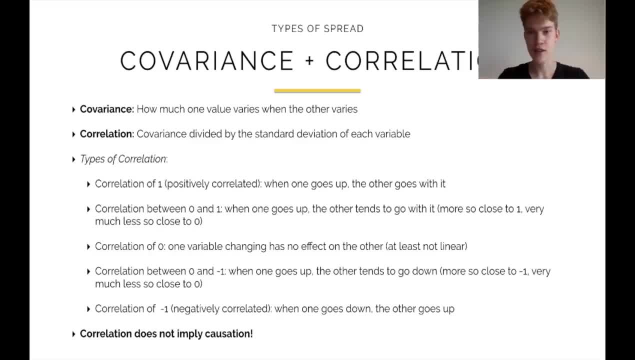 and that's that correlation does not imply causation. So just because two things are correlated, that does not mean that one causes the other. So a good example of this would be if I live in a climate where it's usually cloudy in the morning. 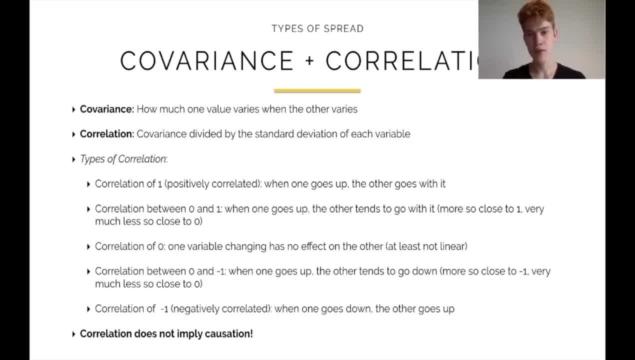 and I know it to be sunny in the afternoon. but every morning, when it's cloudy, I drink coffee and then it becomes sunny in the afternoon. That's not even though they may be correlated: me drinking coffee and it becoming sunny, me drinking coffee does not cause it to be sunny. 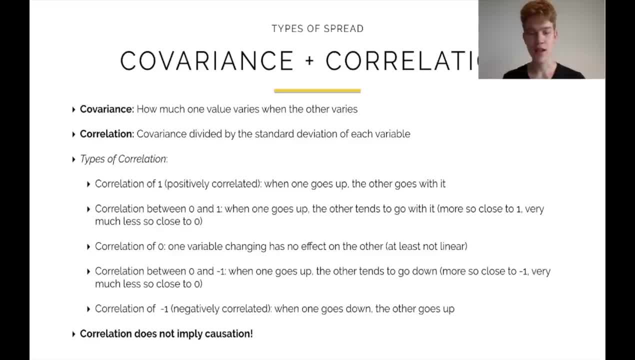 That's just, you know, by chance, It's just because it happens every day And by chance there's this kind of correlation that appears. But that does not mean that me drinking coffee, you know, results in the weather getting better. 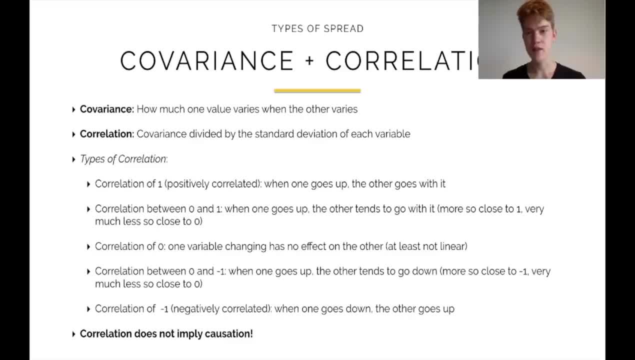 A causation would be me drinking coffee and me feeling less tired, Or me drinking coffee and me feeling happy about it because I like the taste. Those would be causations. So that's an important thing to keep in mind, Just because things are correlated. 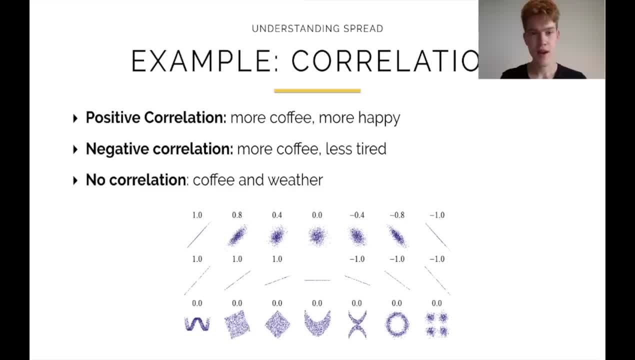 does not mean that one causes the other. All right, So let's see these things on a graph, And so here we have the examples again that we've talked about, But we can kind of see how the data would look like for different types of correlations. 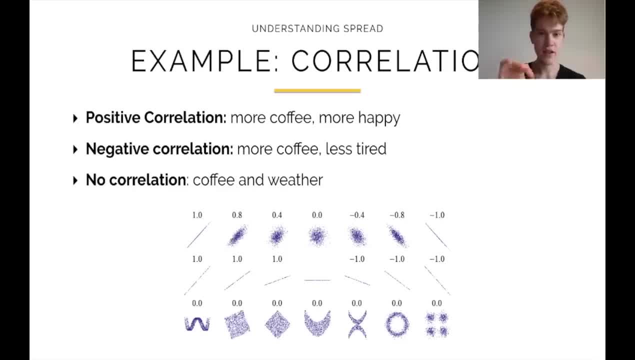 And so we can see a perfect correlation of one. So one goes up, the other goes up. We can see on the left side and we pretty much get this really nice straight line. So one value goes up, the other value goes up with it. 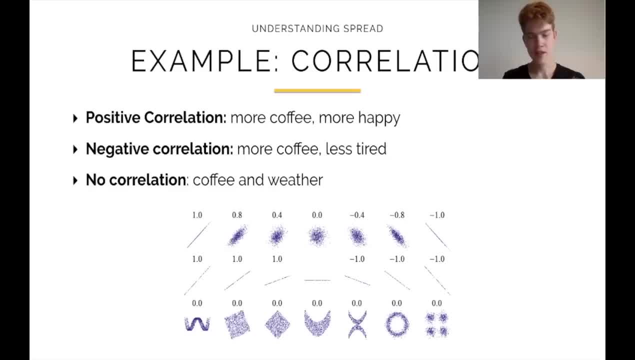 And then the closer we reach zero, the less related or the less correlation there is between them, And then the more kind of variance we have in data. So we'll notice, for the case of perfect correlation, which is the one, or the case of perfect anti-correlation. 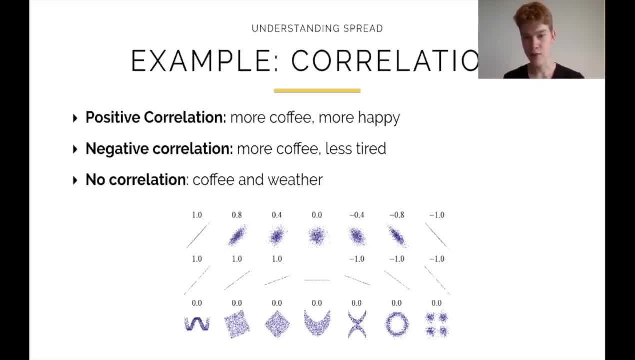 which is the minus one, which again we have the example of more coffee, less tired. In those cases, you know, we have a very nice thin line and our data doesn't jump around a lot, But the closer we get to zero, 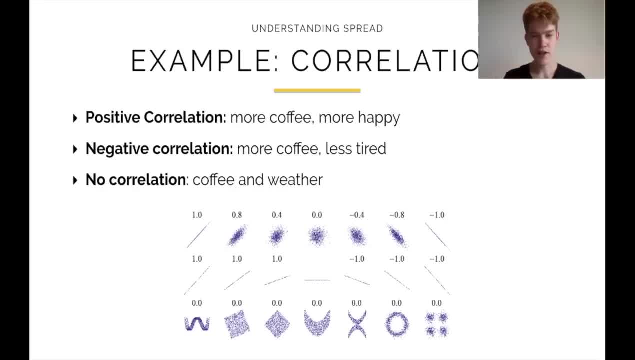 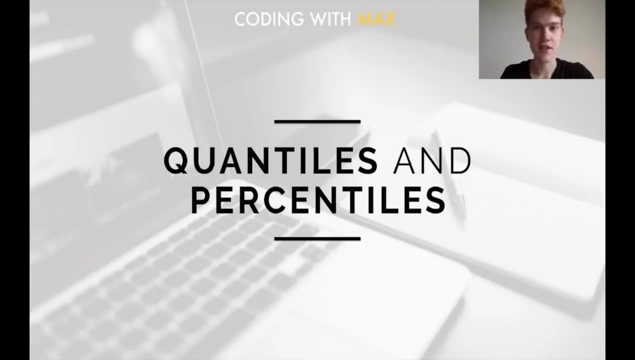 the less we can see you know one causing the other, and the more we can see our data kind of spread out, And so that's what correlation would look like in terms of graphics. In this tutorial we're going to go through quantiles and percentiles. 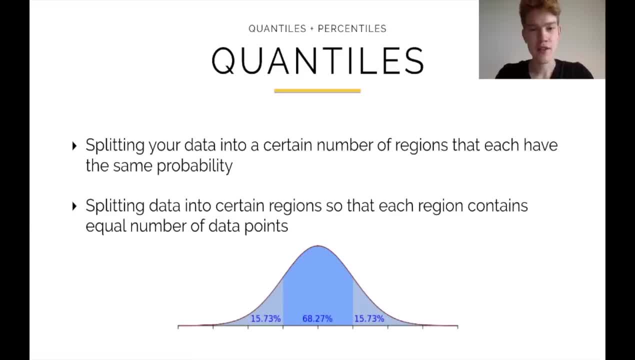 All right, so let's get started. So what are quantiles? Well, quantiles allow us to split our data into certain regions that, if we're dealing with probability, they all have the same probability, or if we're just dealing with, you know, sizes of data. 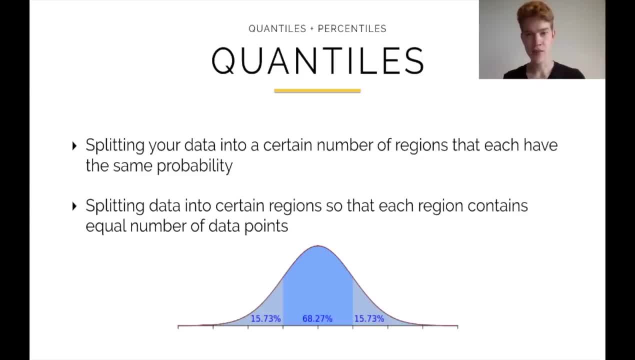 we want to split our data into equal regions. So that's what we can do with quantiles is just splitting everything up so that every time we split it, you know we have equal amounts of data. All right, and so an example of a quantile: 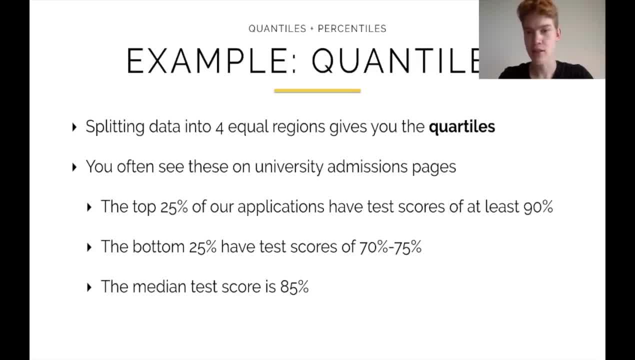 would be something known as a quartile, And so that's when we split our data into four equal regions, hence the name quartile. So a quantile is the general name for doing this splitting procedure. And then if we say quartile, 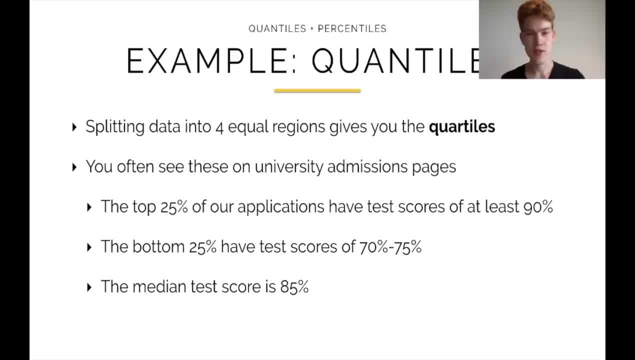 that means we're doing quantiles, but for four equal regions, And so this is something that you'd probably often see on like university admissions pages or something like that, And they say: the top 25% of our applicants have at least a test score of like 90% or something you know. 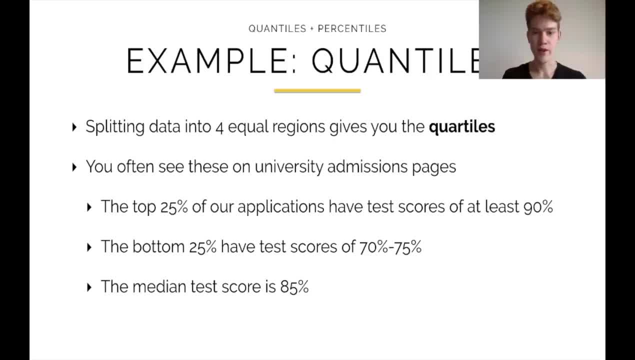 And then they would say: the bottom 25% of our applicants or our admitted students, or something like that, have a test score that is, I don't know, 70% or 75% or something like that, And then the median test score is 85%. 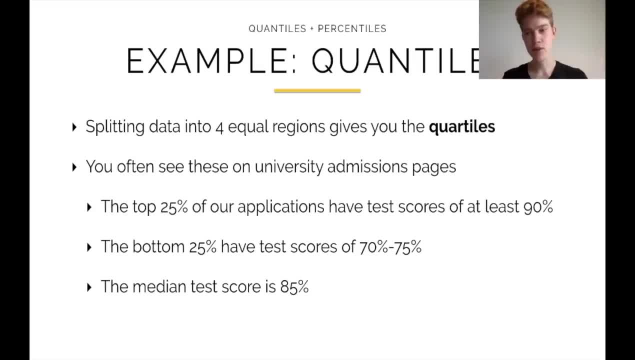 So that's how you would go about quartiles is that you would have, you know, the lower 25%, the middle 25 to 50, then you've got the 50 to 75, and then you've got the top 25%, so the 75% to 100. 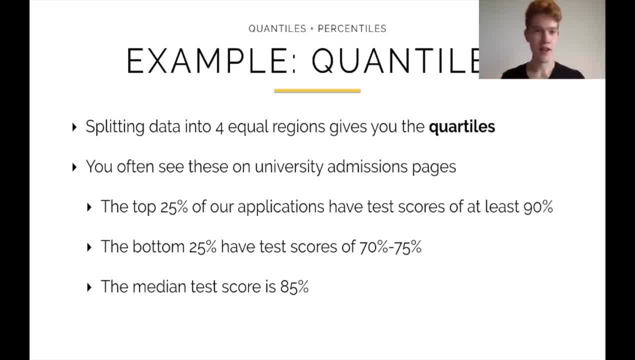 And so you've got these four equal regions, which also include your minimum value at the very bottom, your maximum at the very top and in the middle you've got your median value. So that's the value directly in the middle. That's because you're splitting it up into four equal regions. 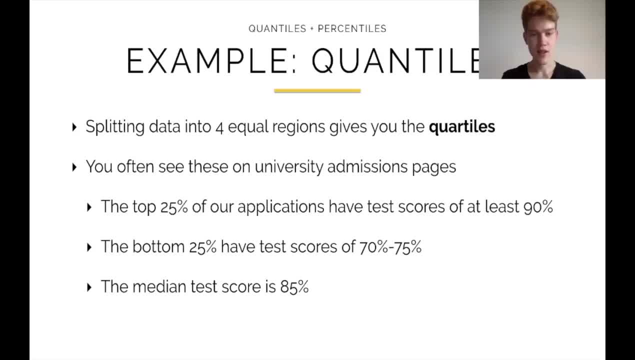 And so the value that separates the second quantile, which would be the 25 to 50, from the third quartile, which would be from 50 to 75, that value there would be the median value. All right, And so, if we go into percentiles, 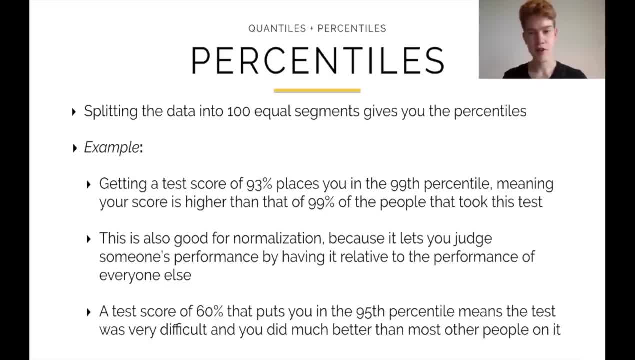 so percentiles? that may have been a name that you've probably heard before. Percentile is again an example of a quantile, but instead of saying you know, like a quartile, we do it for four. a percentile means splitting it into 100 equal segments. 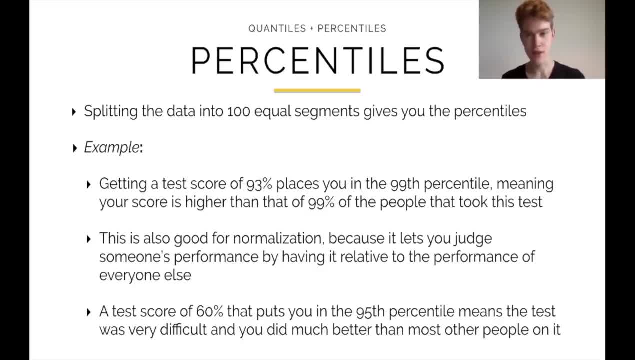 Hence the percentiles, the perks name at the beginning, though that's kind of where the percent you may have noticed. percent means out of 100. So that's, if you are familiar with percent, then that's also the same. 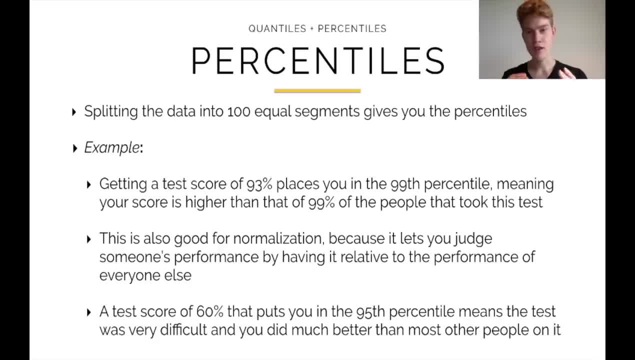 kind of reasoning where this comes from. And so we've got percentiles, which means splitting into 100 equal segments, And so an example of this is often used in test scores. So if you've ever taken something like the SATs or something like that, 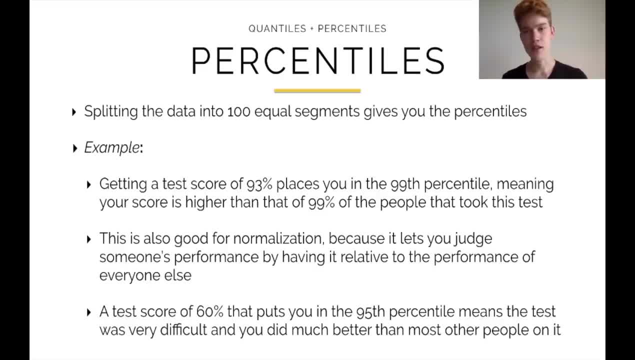 then you get a test score, but you also get a percentile, And the reason that's done that is it's to judge not you versus the test, but you versus everyone else, And so if it's a difficult test, then something like getting a test score of 60%. 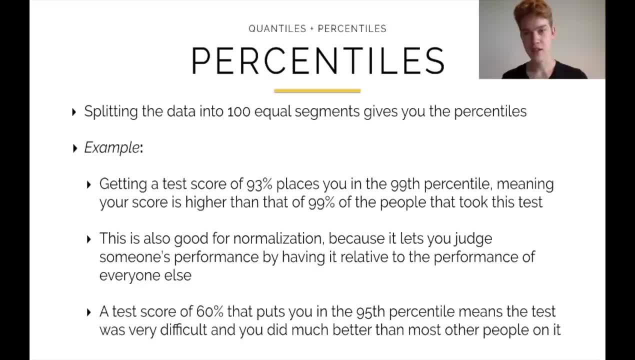 but you're in the 95th percentile means your score is actually a lot better, And so what you can say, with percentiles, for example, is that every percentile that you're in means you're better than you know that many other people. 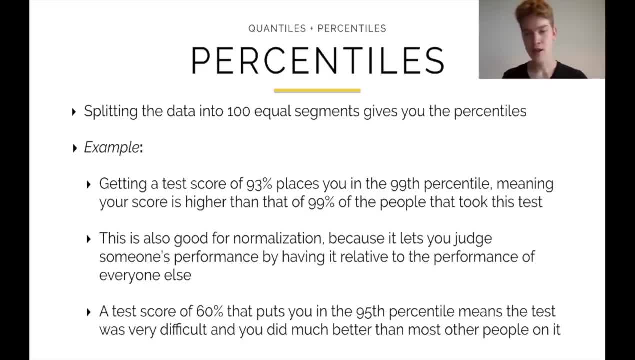 So, for example, if you reach the 99th percentile, that means you're better than 99% of the people that took the test. The 95th percentile would be: you're better than 95% of the people that took the test. 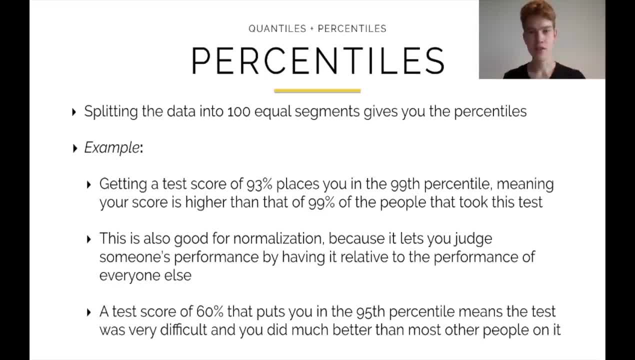 or something like that, And so that's why percentiles are often used for tests, and they're often used for normalization, because they allow you to take into consideration, you know, these factors of like. is it a difficult test? Is it an easier test? 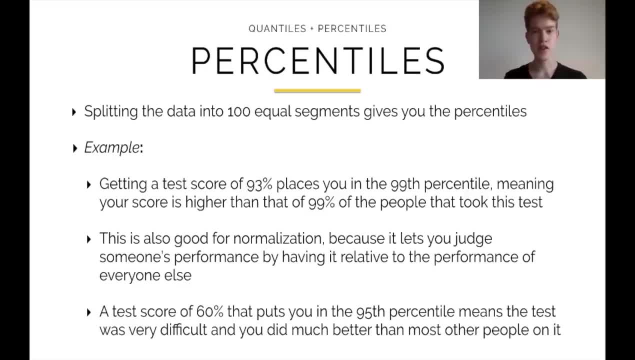 Maybe more people are scoring higher So they don't really judge you directly versus the test, but they normalize you against everyone else that took the test. So you take the test, you get a score and then the percentile checks where that score lies. 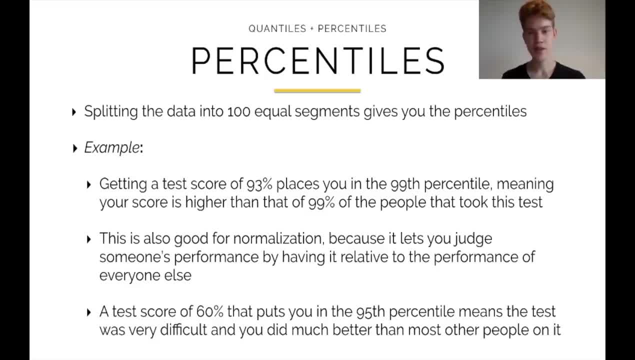 relative to everyone else. And so these percentiles, they allow you to give a good normalization and they allow you to do great comparisons, because they allow you to kind of eliminate some of these factors of test difficulty. And of course you know there can always be luck involved and stuff. 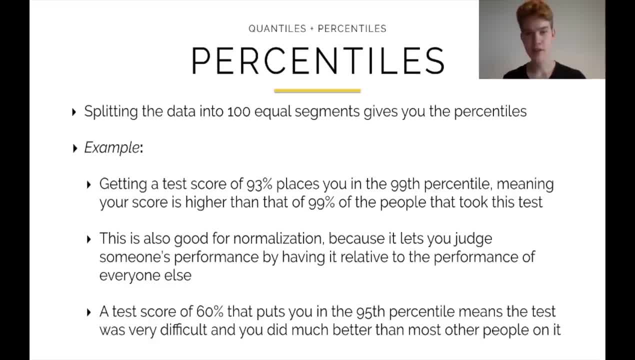 and that may not get filtered out on an individual basis. But if you do this, for a lot of students- and that's also why it's done in these kind of big standardized tests- is that you get a percentile along with your score, so that you understand if. 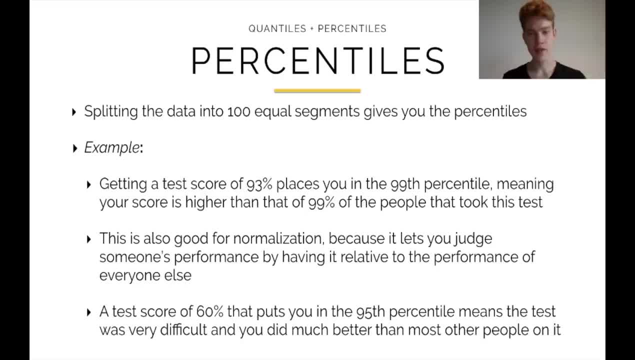 you know, maybe if your score is lower, but the test was really hard, you can still see. you know, I did really well, because people found this test really hard and it was even harder for them than it was for me In this tutorial. 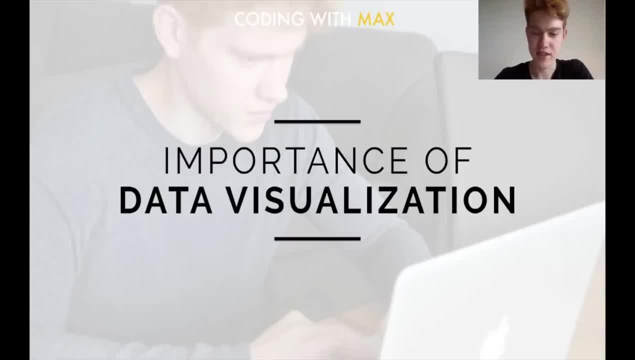 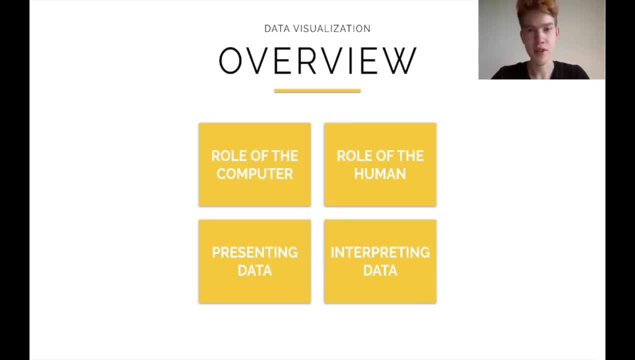 we're going to talk about the importance of data visualization, All right. So what we're going to talk about is, first, we're going to look at the role that the computer plays Kind of for us, and what role the computer is actually made for. 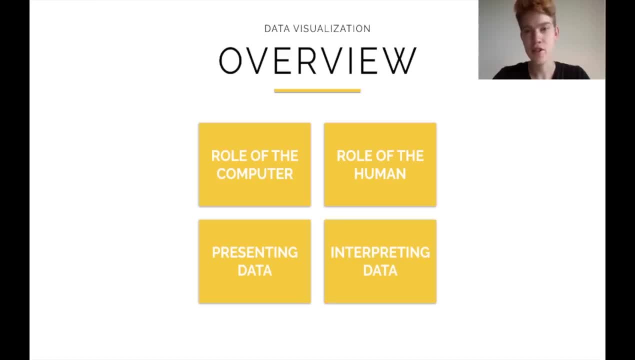 Then we're going to look at what role the human should play in terms of data science, Then we're going to look at presenting data And finally, we'll talk about interpreting data. All right, So let's get started and talk about the role that the computer plays. 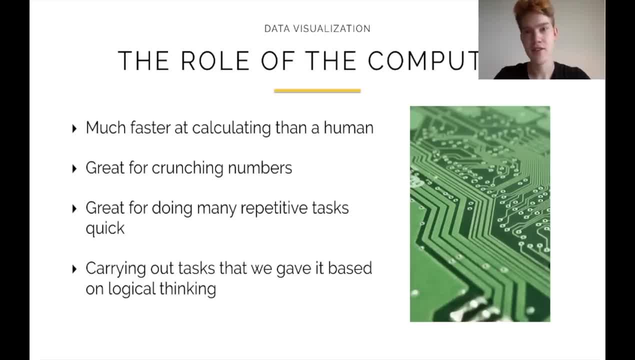 Now, computer is much, much faster at calculating than human, because that's what it's made for. It's made for crunching numbers, It's made for doing fast calculations. You know, if you think about how fast our computers are, they're in the gigahertz range. 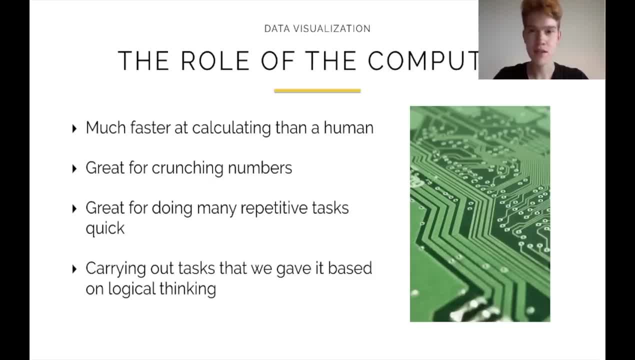 So giga means billions, So they just do billions of things every second, And so they're really good for doing repetitive things because they can do them so fast. And then we can give them these logical tasks in terms of programming And we give them a structure and they just do it. 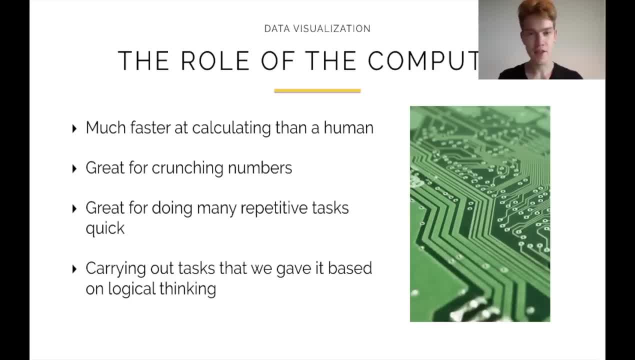 And they can do it over and over and over again. They're not going to mess up. They can just repeat the same thing. They won't get tired of it And they're really good and they're really fast at doing these things. 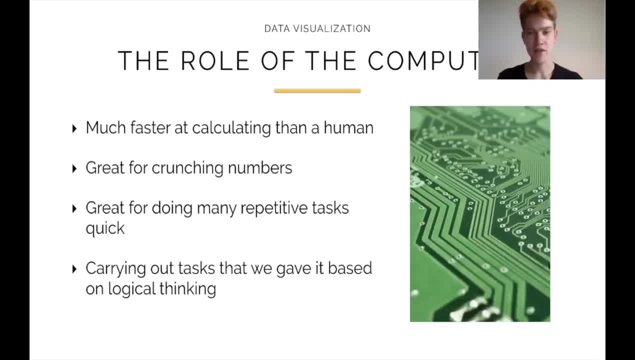 So that's the role that the computer should play for you. It should be kind of a means to get these hard number crunching and all of these things done. So there's really no need for you to kind of work out all this complicated math. 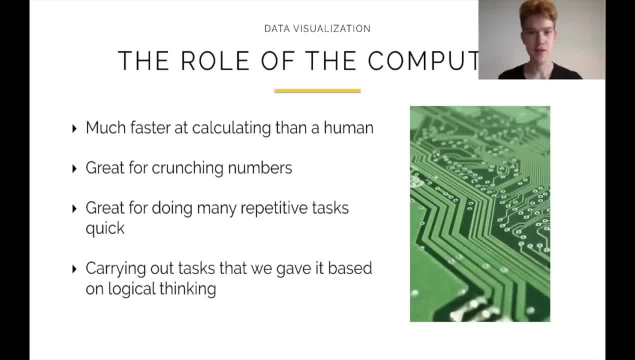 because your computer can do it much better and much faster than you, And it's also less prone to error if you code it correctly. So that's kind of the only part where you come in. It's only going to mess up if you mess up. 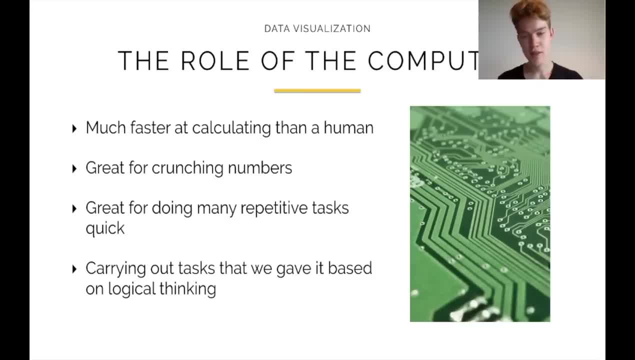 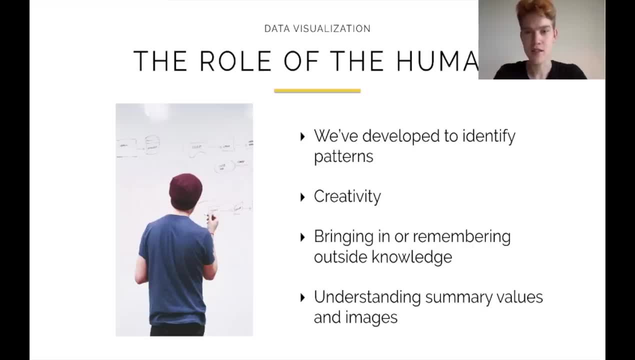 But generally, our computer does exactly what we tell it to do, And it's really good and it's really fast at it. Now, what role should a human play in terms of data science? Well, humans have naturally developed to identify patterns. 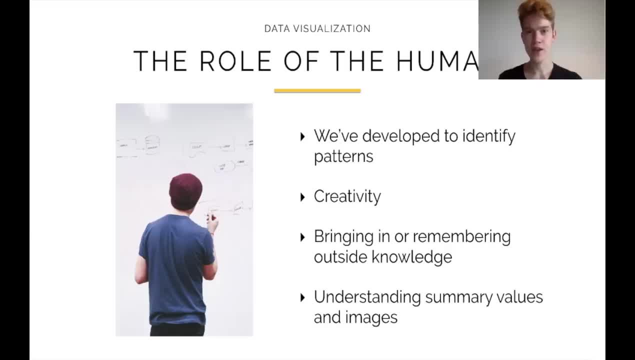 And we've done this first for survival, So that if we're walking around somewhere and we see a- I don't know a big predator hiding, that, we can identify that pattern of the predator and we can kind of pick it out, even though it's trying to camouflage itself. 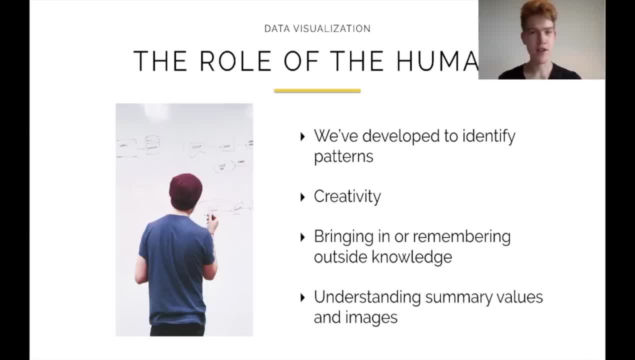 So humans, by nature, have become very, very good at identifying patterns. And you can also see this if you look at the clouds and you see things, or you see animal shapes in the clouds or other things. So those patterns aren't actually there, But humans have become so good at identifying patterns. 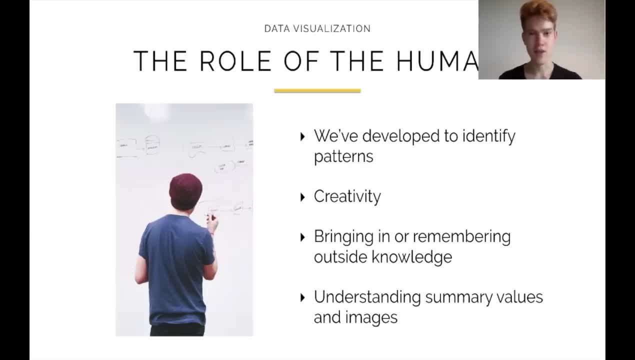 we can see things in many, many places, And so that's what humans are really really good at: We're able to look at things and we're able to pick out patterns. Now, another thing that's really good for humans is we are very creative. 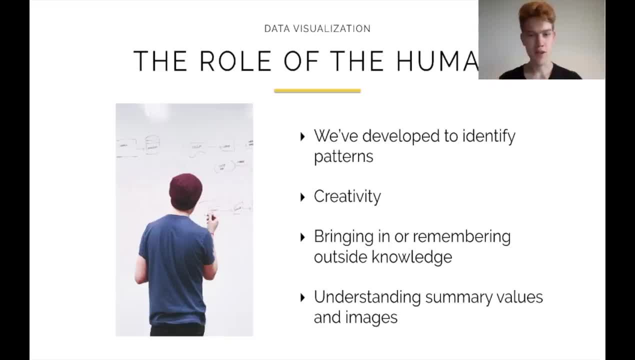 And through that creativity we can also use memory and bring in outside knowledge, And we can also use a general understanding, And so these are all things that computers can't do. So computers are kind of a means of getting stuff to us, But once it's actually there, it's our job to use our pattern recognition abilities. 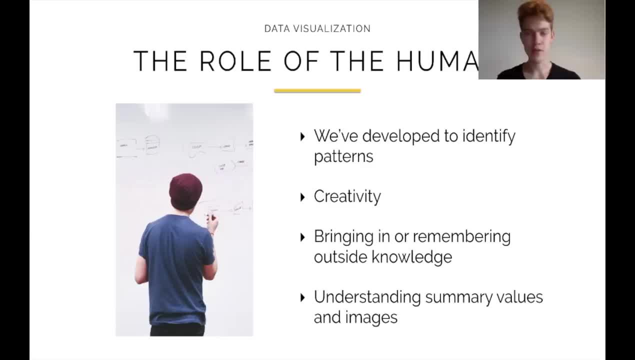 And of course you can train machine learning algorithms for specific patterns later on or specific cases and make them really good at that. But generally, if you don't know exactly what's going to come, then our or your first step as a data scientist would be to try to identify these patterns. 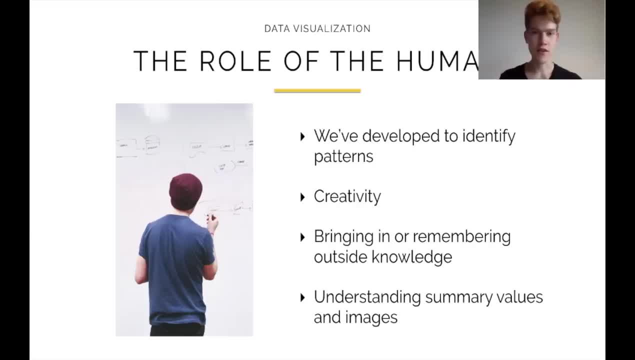 Use your creativity, use your memory, you know, bring in all of these different things, Use all of these different things that make you human, and use all of that on the data, All of these things that a computer just doesn't have any access to. 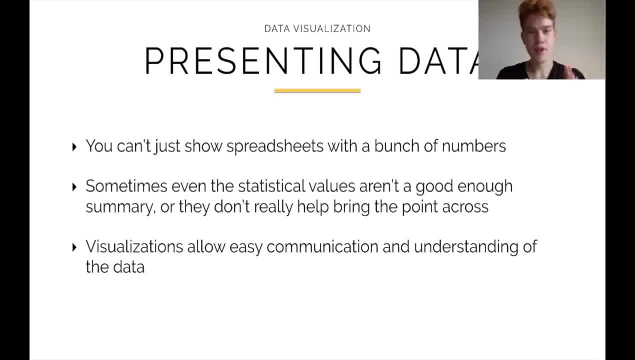 Okay, So You know you're considering all of this. The best way to do all of this would be in terms of data visualization, So you can't just show spreadsheets with a bunch of numbers. That won't really help you, because looking at numbers, it's really hard to pick out patterns. 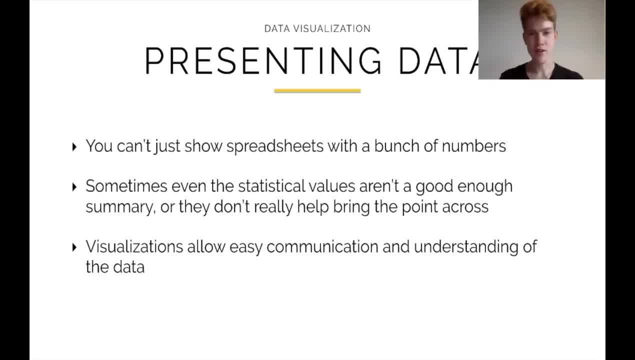 The best way to do it would just be to plot values And then if we have these visuals in front of us, then you know we can really identify patterns. We can see things go up and down and you know we can see them fluctuating and we can see them make very thin lines. 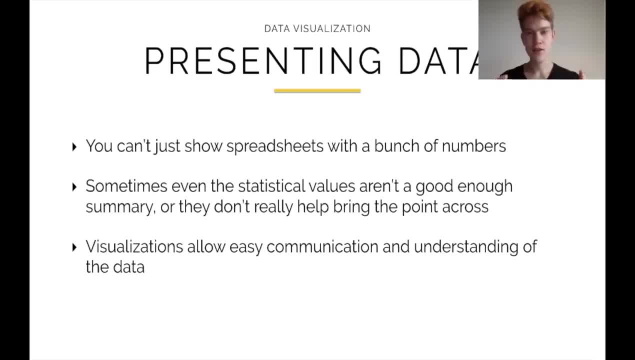 We can just look at a graph and we can just see things. And of course you know we need a little bit of practice to understand what that graph is trying to tell us. But once we understand the graph in general, then you know we can look at new graphs and we can just see things. 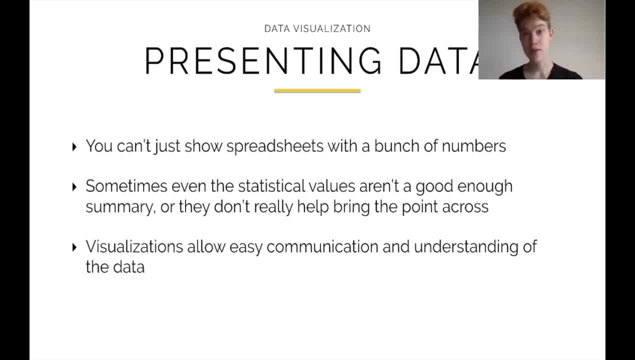 We can start to see patterns, and they may not always be true, But that doesn't mean, you know, we can't pick them out, And then that's later on. You would also do some testing, trying to see if those patterns are true, if they make sense. 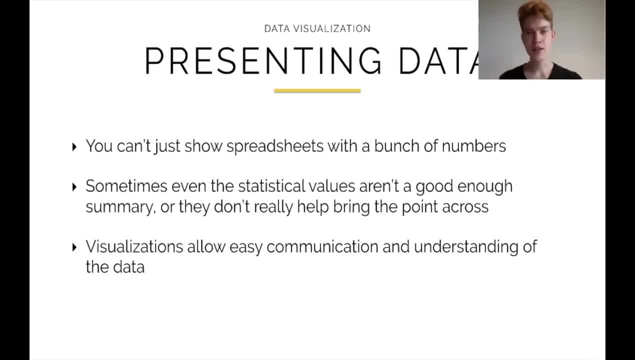 But generally, data visualization is very good for this, because it allows you to invoke all of your human characteristics, the things that are really good, that you know make us human, The things that we talked about in the last slide, all the things like the computer can't do. 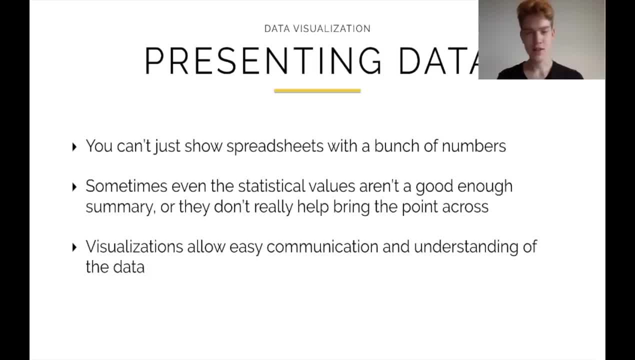 And sometimes you know, if you deal with just these numbers, data visualization is for you in one sense, so that you can see these things and try to pick them out and use them later on, But also if you're trying to show these things to other people. so maybe you have to do a presentation, a kind of summary. 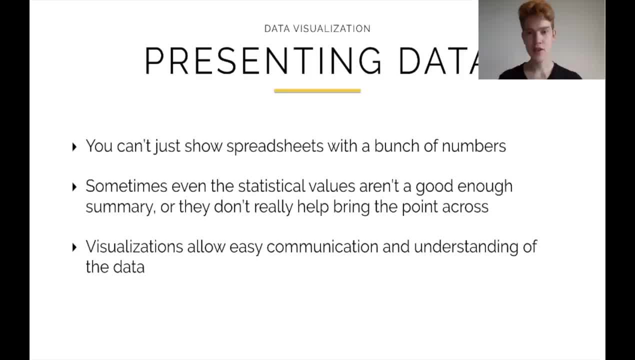 then you want to make sure that your data visualizations are good, because the people that are going to be looking at it are much, much less trained at looking at data and analyzing data than you are, And so if you try to convey them a message and just show them a big spreadsheet with numbers and just point out like 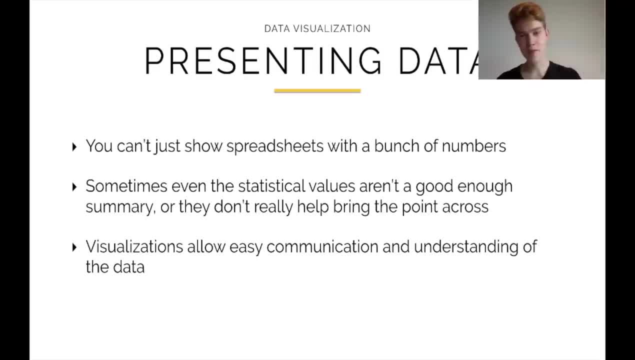 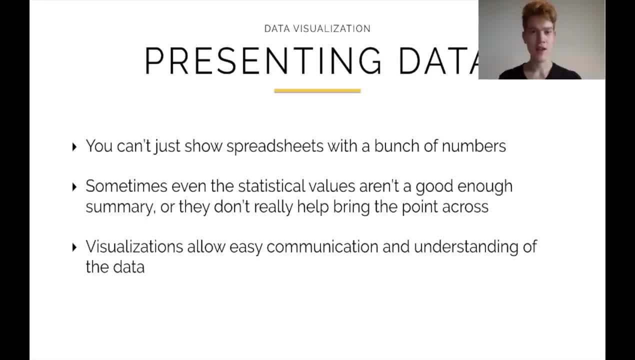 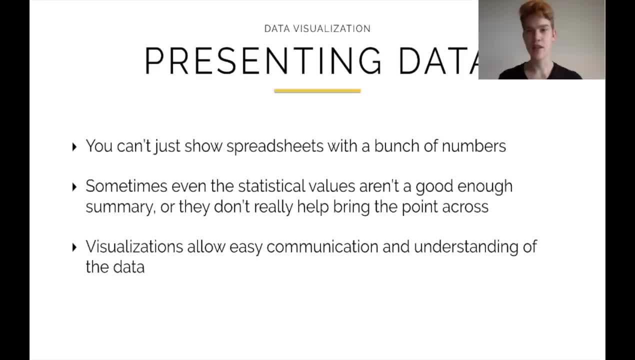 But the other part of it is to show it to other people and to kind of help you convey information to them. You know, of course, we talked about statistical values, and statistical values are very important and they can give us a good idea about the data and what's going on inside of the data. 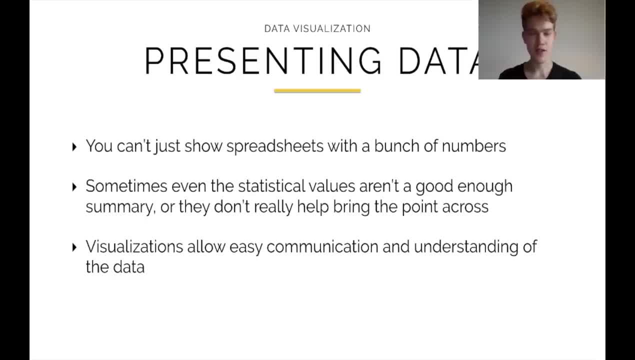 But visualizing data is just taking it to the next level and statistical values aren't enough there. they can give us, you know, they can help us, they can support us, they can give us ideas, but if we really want to understand what's going on, sometimes we just have to take a look at what's going on. 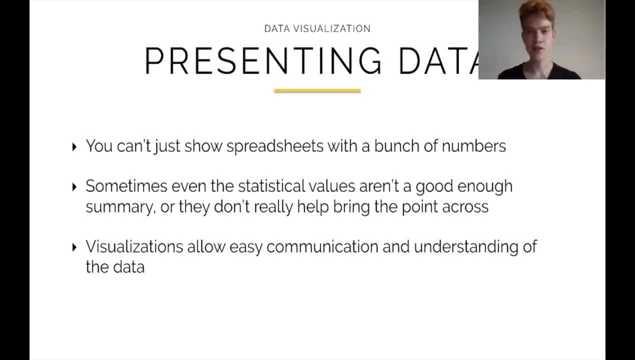 and, of course, there it's also important to make sure you choose the right visualizations and everything, because other times, you know, it may just look extremely weird, but just this skill of being able to present data both for yourself as well as for other people, is very, very important. 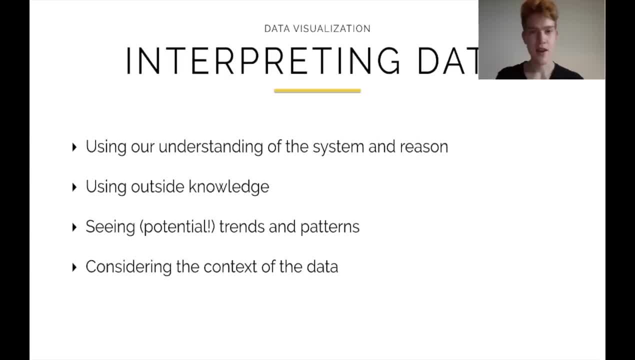 for a data scientist, and then we go over to interpreting data, and we've kind of touched on this in the last section already. but really, with data visualization, it just allows you to see this data and it allows you to apply some reasoning to the system, and so you can. 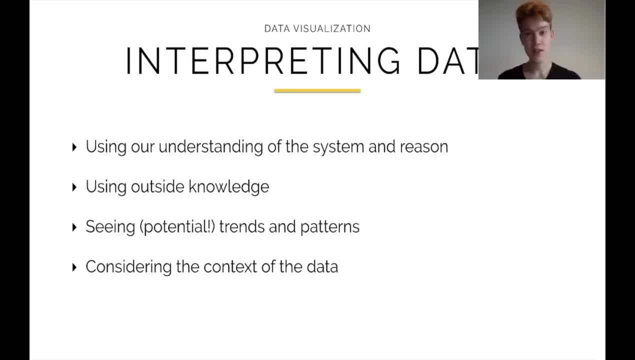 if you look at data, either you see something which is great, you know. that means you can try to test something, see if it's actually there- or you don't see anything, and that also tells you something that you aren't really able to pick up, and it's not something that you can pick up and it's not 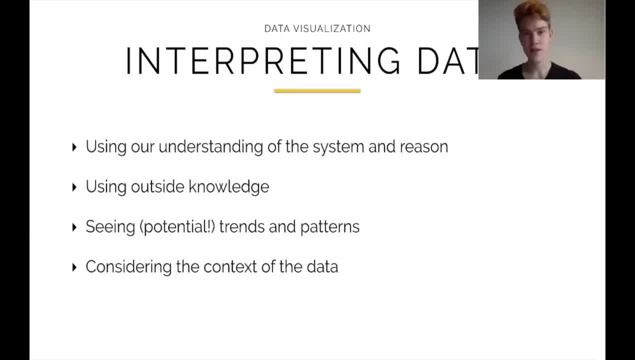 a pattern, so that there isn't. there isn't anything obvious that's going on. there may be something underlying that's more complicated, but obvious to the user. you know it's not there and so all of these things allow you to, you know, kind of easily, or much more easily, analyze your data and kind of 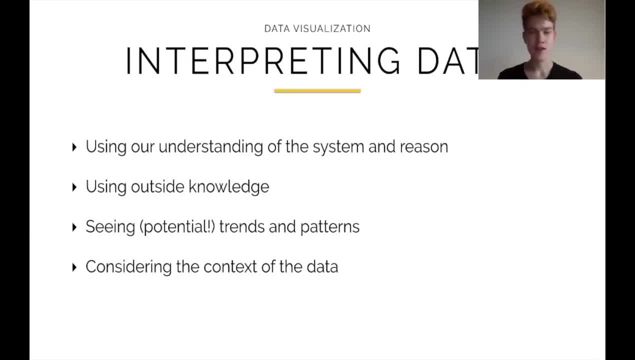 prepare what you're going to do after that. so this data visualization: it really gives you a deep, deep understanding of what's going on with your data and then, when we interpret this data and we look at these visualizations, we're going to be able to see what's going on with your data and then 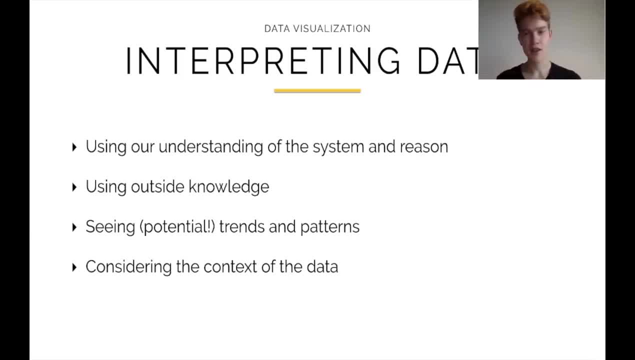 maybe you see dips and you know, maybe you see some hills somewhere. we can try to understand all of this by bringing in our outside knowledge. so, again, what the human is really good at, we can, you know, bring in the context of things. you know. maybe people are going out to lunch here and so that's. 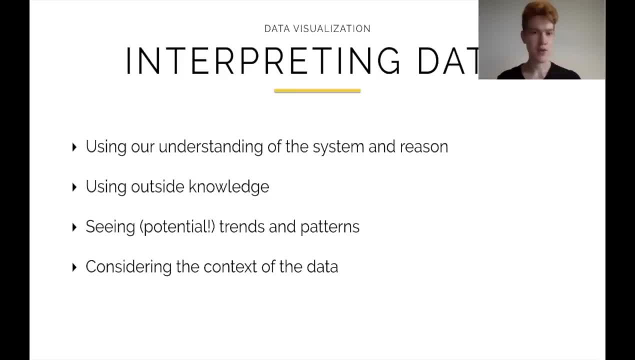 why activity decreases. or maybe everyone is coming to work in the morning and so that's why activity increases compared to, you know, 6 am. so all of these things, we can bring in all of this context, we can bring in all of this understanding, and so that's why activity increases compared to you know. 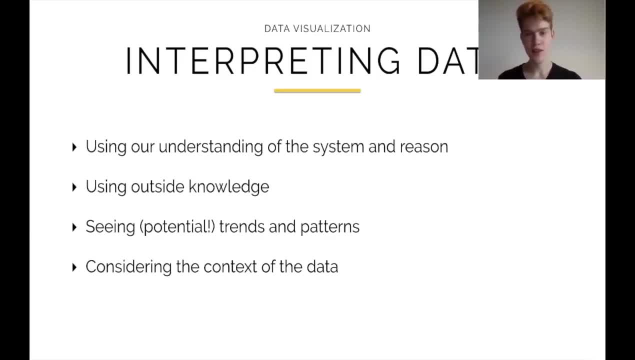 we can bring in all of this context. we can bring in all of this context, we can bring in all of this understanding to try to interpret the data, to try to better understand what's going on. and then, of course, we're gonna see, hopefully, some trends or patterns. of course, like I said, these may not always. 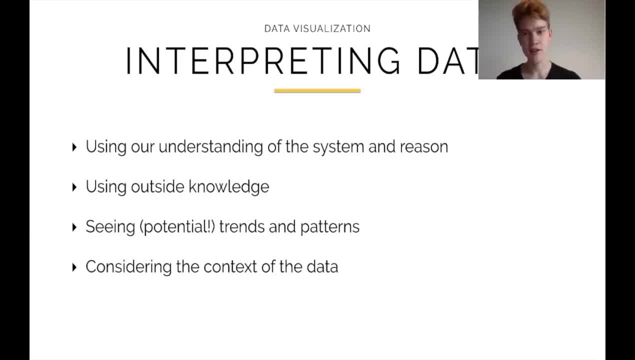 be there. so we're actually so good at pattern recognition that we can see, sometimes, patterns that aren't really there, and so a good example again of this would be just looking at the clouds in the sky and you can see animal patterns maybe, but that's really not there. that's just our mind. 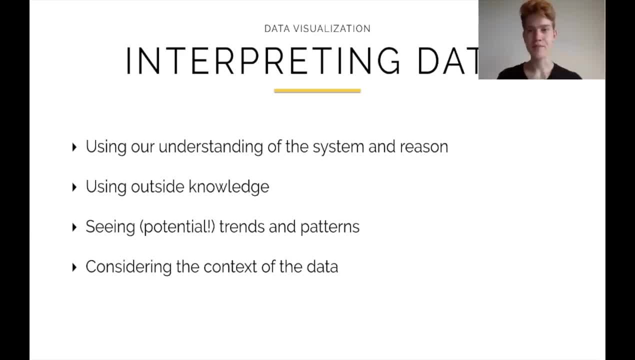 you know, identifying all of these patterns and so, yeah, that's. that's pretty much why data visualization is so important to a data scientist. it's because this whole human aspect is it's just key in data science, it's key in data analytics to be able to understand what's in front of you. 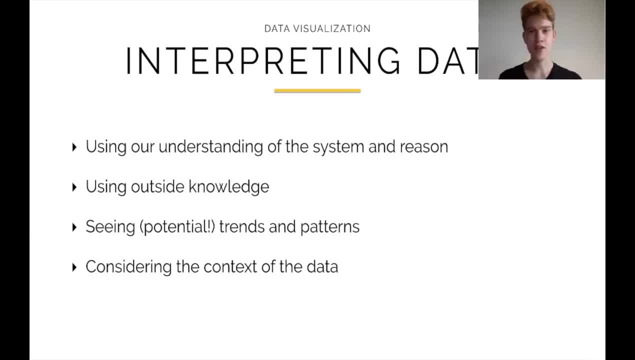 to be able to understand, to bring in these, this outside knowledge, to be able to contextualize this creativity. that's really key to a good data scientist, and a computer can help you with all of this. the computer can help you. you know, do the number crunching a computer? 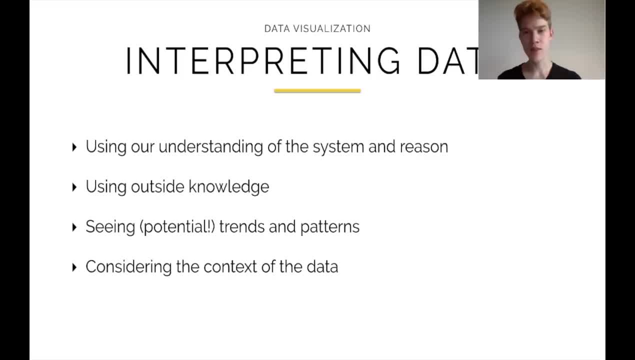 can help you set up the visualizations, and it can plot whatever you want for it, but ultimately it's up to you to choose the right visualizations to do, to look at the data, to be able to communicate the visualization as well- all of those things are up to you, and so that's why the human is so. 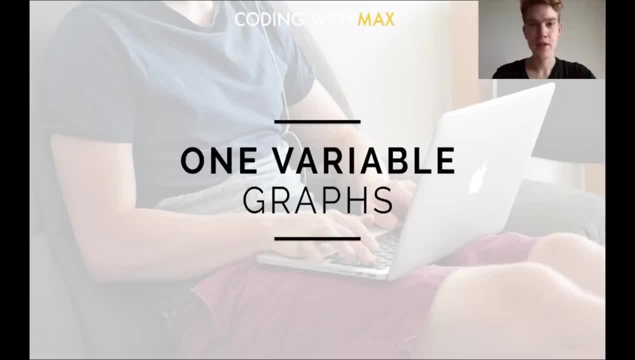 so important in data science. in this tutorial we're gonna look at one variable graph, so we're actually going to see some of the types of graphs that we can do. you know that we talked about in our last tutorial, where we just looked at the importance of data. 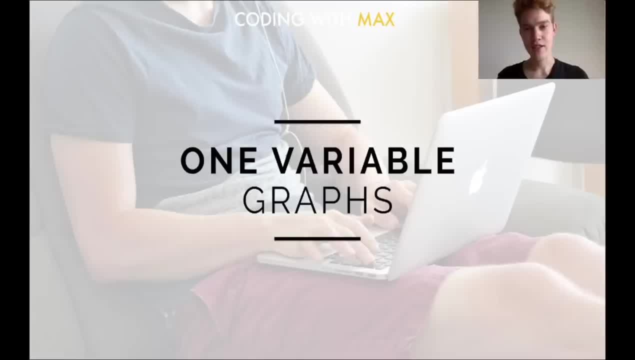 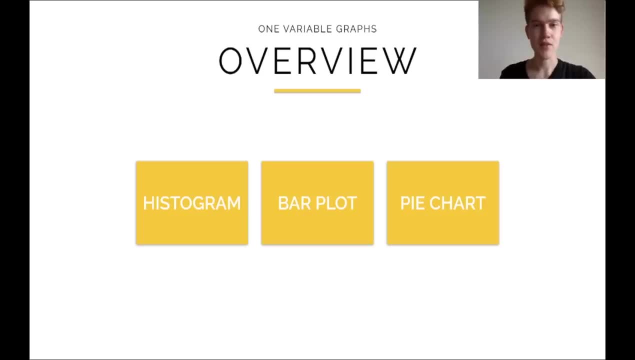 visualization. so now we're gonna go into data visualization and look at the types of graphs that you may want to use or that you may want to choose from, all right, and so the graphs that we're gonna look at in terms of one variable graphs are going to be histograms, bar plots and pie charts. so 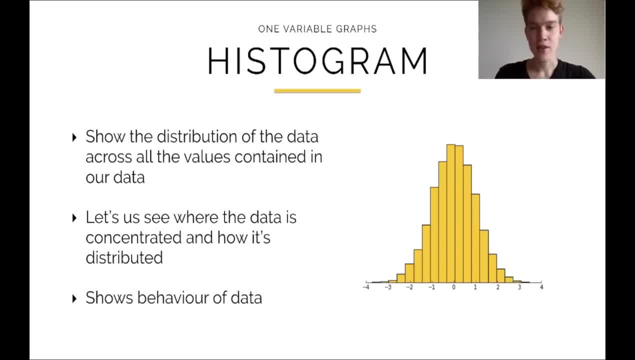 let's get started with histograms. now we can see an example of a histogram on the rights, but what's really cool about this is that if you look at the histogram, you're going to see a bunch of histograms. histograms is that it shows us the distribution of the data and it shows us the distribution. 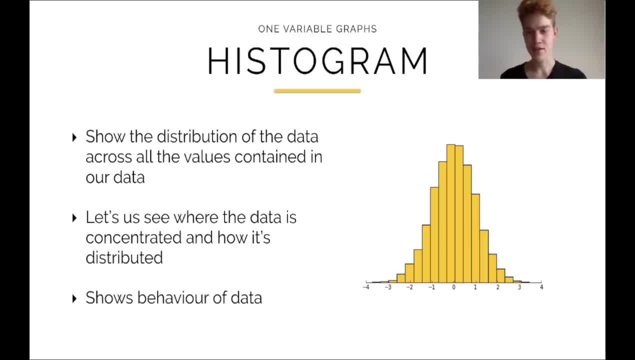 across all the values in our data, and so it shows us what happens the least and it also shows us what happens the most. and histograms, they let us see where our data is concentrated and they also let us see how it's distributed, and so through this it kind of shows a general behavior. 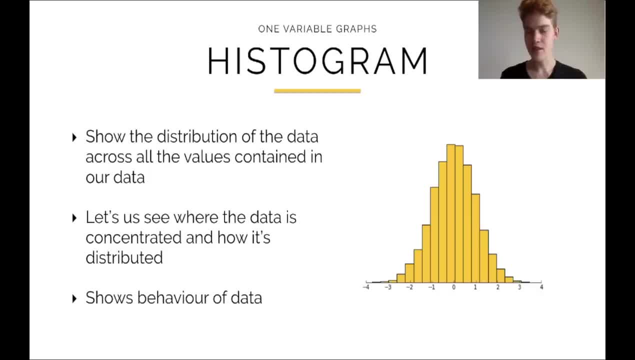 and so, really, what a histogram is is it looks at each value and it just looks at how often the value has occurred, and so what we see here, for example, is that around zero, you know, we have the most occurrence of whatever value we're looking at, and as we move to the left and as we move to, 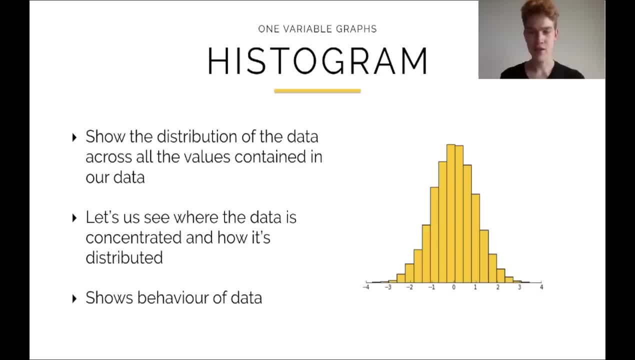 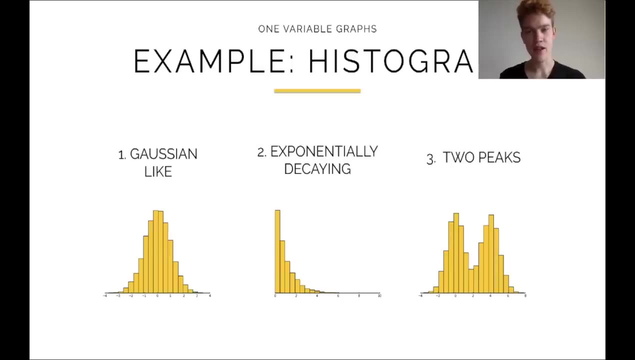 the right, these values start to drop off, so they start to become less frequent, and so that's what histogram shows us. the histogram shows us a kind of frequency, how often these things occur, and so there are different types of histograms that you can encounter, or i mean generally a histogram. 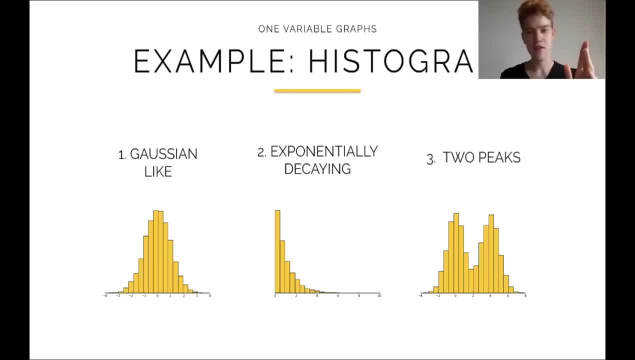 is just this plotting of frequency versus your value, and so there are different ways that this histogram can look like. one of them is the one that we've just seen, which is a normal distribution, or it's called gaussian like histogram because it follows this gaussian distribution or this normal distribution. 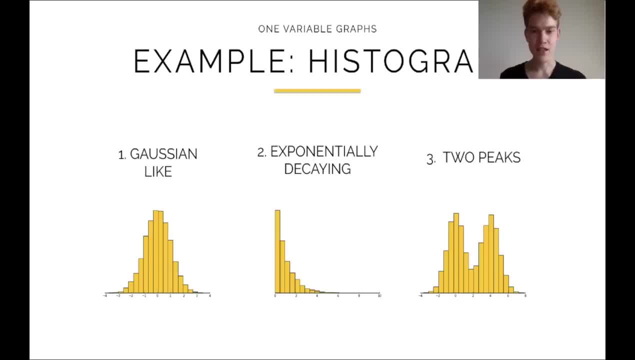 that you know. but we can also have like an exponentially decaying value. so we start off very high and the further we get away from that initial value, the quicker it's going to decrease to the gaussian like or to the normal distribution. so the normal distribution looks more of like a. 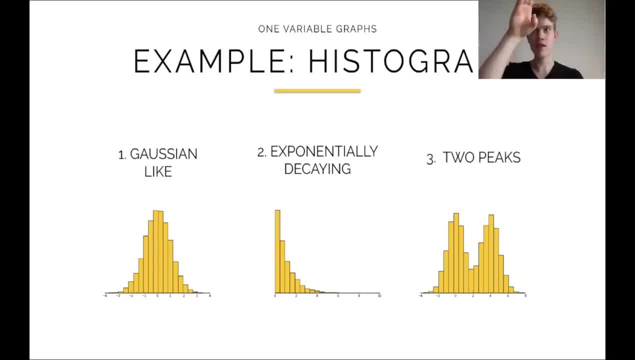 bell it kind of goes up and then curves down slowly, whereas the exponential it cuts off very fast and then kind of slows down later on. so they do have different behaviors. and then of course, you know, we can also get not just one peak, like we see in this first case and the gaussian, like 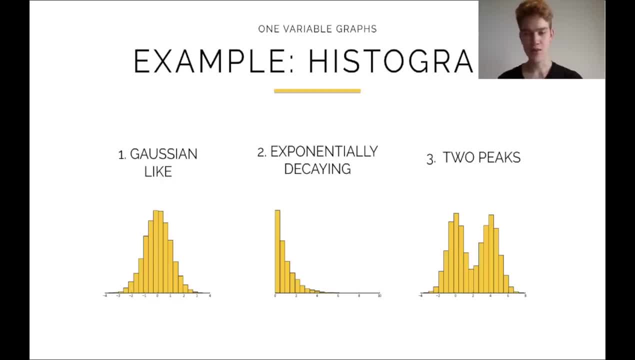 distribution. but we can also get things like two peaks, or we can even get three peaks or more. we can even get three peaks or more, and then we can even get three peaks or more, and then we can even have very large extended peaks. And so our histograms. there are means of showing us how. 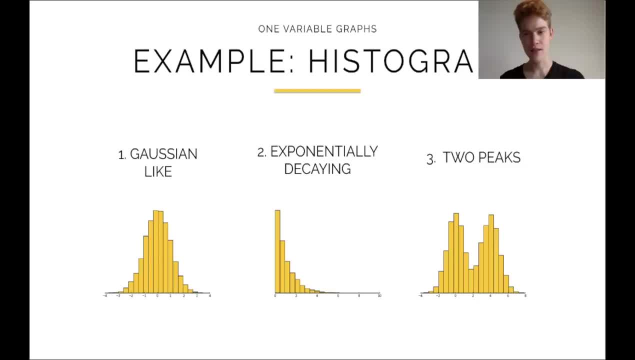 this data is distributed. there are means of showing us, you know, what things occur most frequently, where's our data concentrated? but that don't that doesn't mean that they're going to have to have a specific value, And so there are specific shapes, So there are many different. 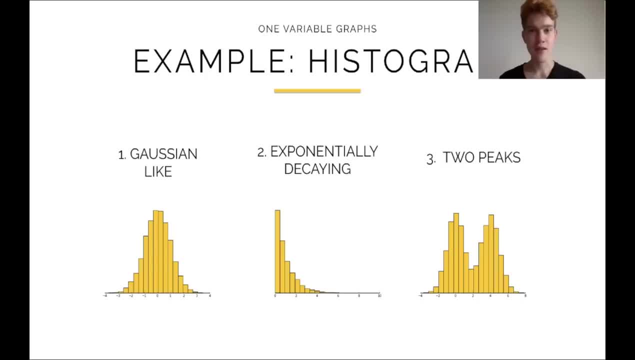 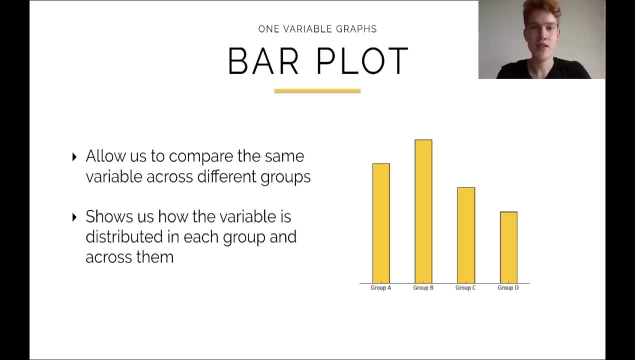 shapes that our histograms can take on, And, depending on what shape that you get, that also tells us something very different about our data. Alright, so the next one variable plot that we'll look at is going to be bar plots, And so what bar plots do is they may look a little bit similar to. 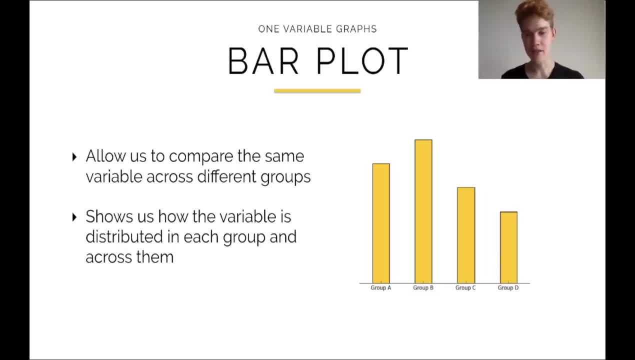 histograms at first, but they're very different in some sense because bar plots allow us to compare across different groups, And so that's what we see on the x axis. down there is: we look at different groups And so we use the same variable. 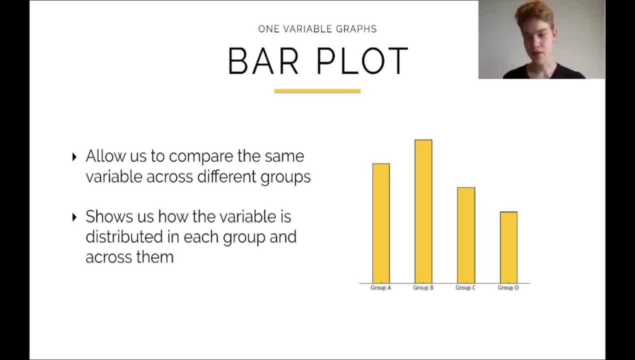 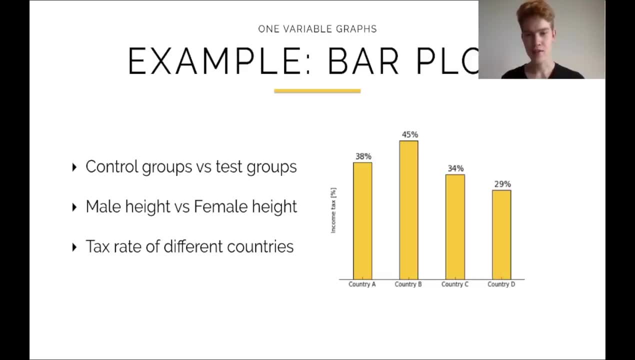 And. but we can compare that variable over different groups And so if we look at that in example, so what we see on the right here is we look at different countries And what we show is we show the average income tax And so we see that country B, for example, has the highest average. 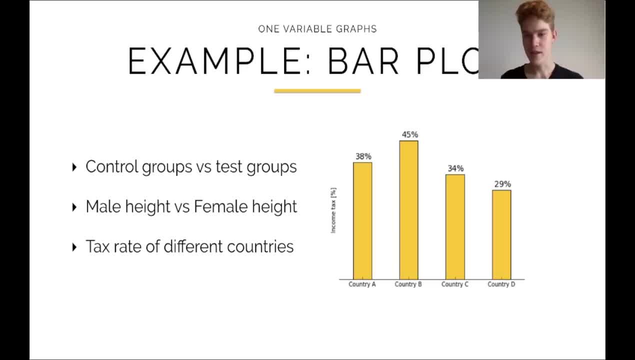 income tax, whereas country D has the lowest income tax. So through this, you know, we're still only looking at the income tax variable, but we are able to compare it over different groups, So we're different categories, if you will. So other examples would be, if you look at control groups and 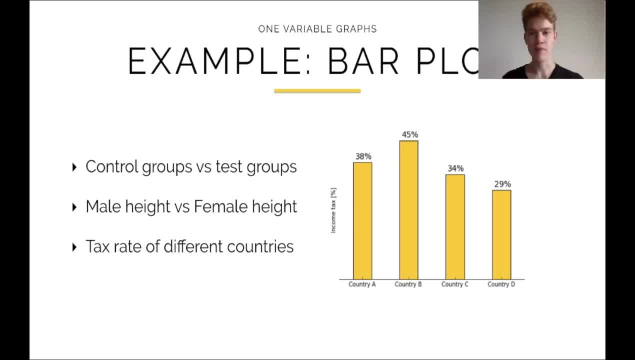 test groups. So if you're doing some like medical study or maybe some psychology study or something like that, you always want to have your control group And then you can have different types of test groups And then you can plot each of these groups as a bar plot And you can look at the same. 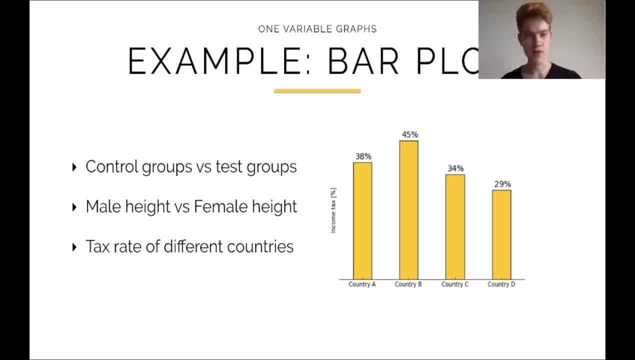 variable, But you can look how that changes over the different groups. Another example would be something like comparing male versus female heights. So you can plot one group that's male, the other group that's female and you can just plot their average height. 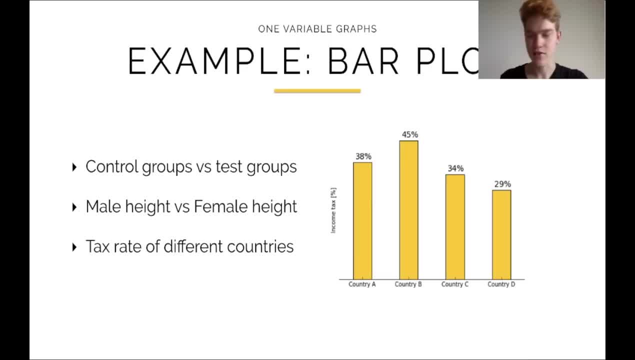 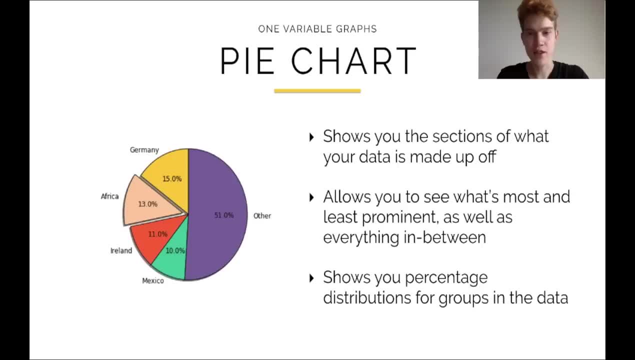 And then the tax, the income tax of different countries, which is what we've seen on the right over here. All right, And so the last one variable graph that we're going to look at is going to be pie charts, And what pi charts are allows to do is they allow us to section up our data and the, and then we can kind of 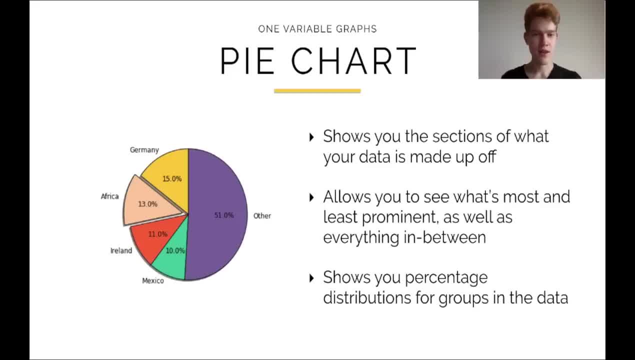 split it into percentiles And because of this we can see what our data is made up of. So the whole pi corresponds to 100%, and then we kind of cut it down into different slices and through that slicing and then hopefully also color coding, like we've done here, and maybe even labeling, or most definitely labeling, so that 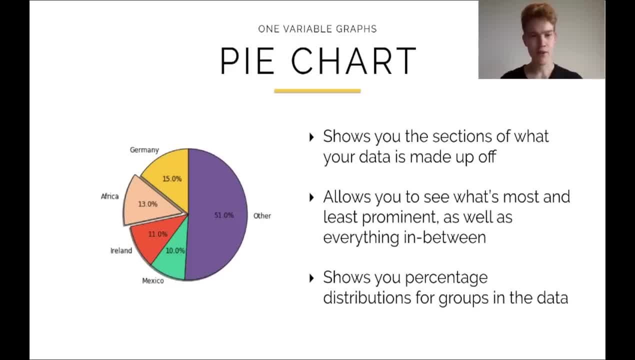 you know what slice corresponds to what value. we're able to see what categories you know, or what, what categories our data is made up of, and so we can see what is most prominent, but we can also see what is least prominent in all of these things, and then again, here we can see also. 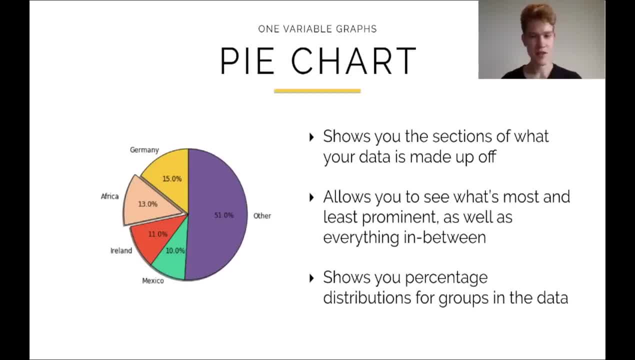 distributions, not as well as in the histogram, but we can still see distributions in terms of dominance, in terms of how many groups there are. is the data spread evenly? is it, you know, heavily concentrated in one part of the pie? all of these things in allow, you know, is that's what we're? 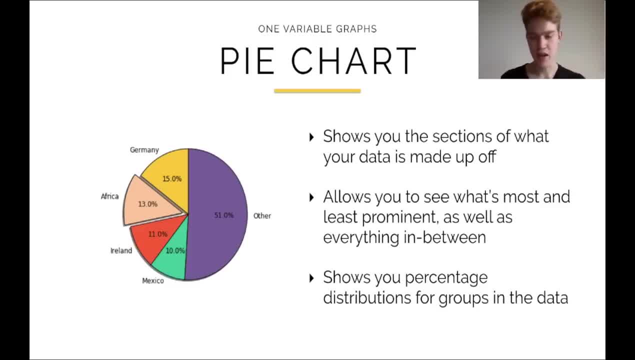 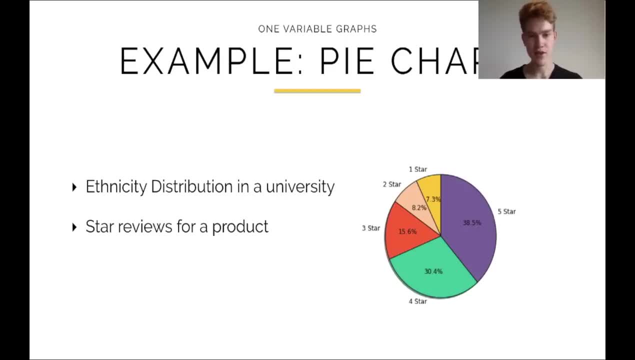 able to do with pie charts. we get this nice kind of group overview of one variable. so examples of this would be: you can look at ethnicity distribution in a university, and so you can have a pie chart, and just each slice of pie would just represent a different. 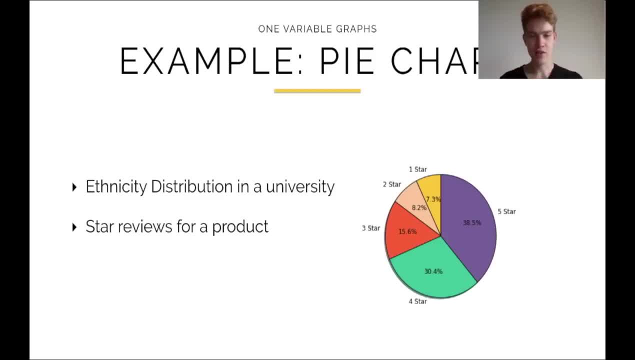 ethnicity and depending on you know how much of a percentage they make up the total university profile. that's how big the slice of pie would be, and so you can see dominance of some ethnicities as well as you know minorities. but you can also see just by how many slices there are. you can see. 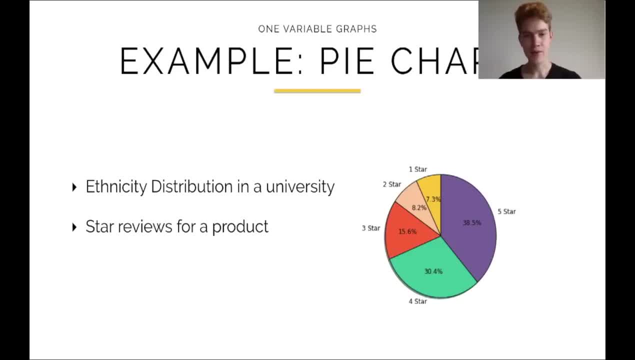 how many different ethnicity groups there are. and another example would be: you can split up star. so rather than you know looking at the average star review, you can also just use a pie chart and you can see how many of my reviews are five stars, how many of them were four stars, three, two and one. 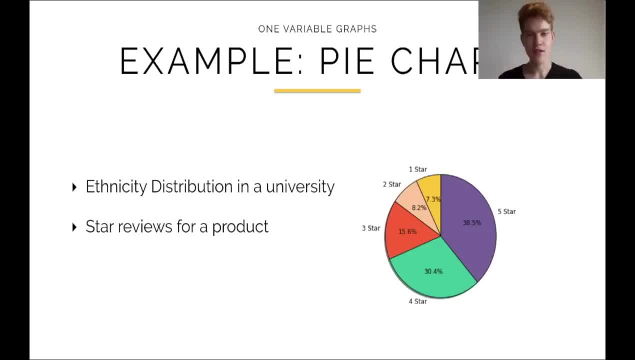 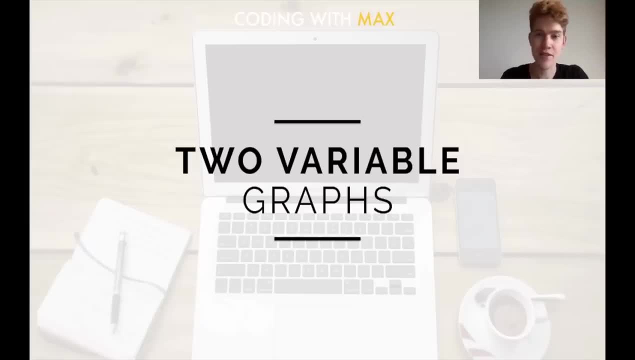 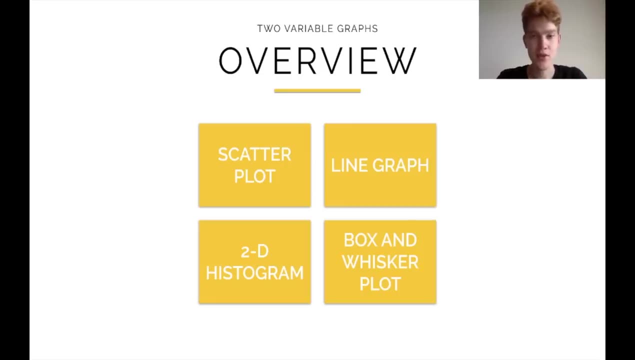 and so there you can again also get this nice, different overview of how the review system would work. now we're going to talk about two variable graphs, so the graphs that we're going to look at are going to be scatter plots, line graphs, 2d histograms or two-dimensional histograms. 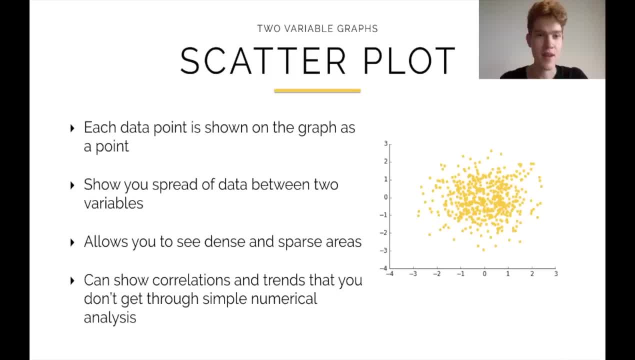 and box and whisker plots- all right. so let's start off with scatter plots. now for a scatter plot. what we're doing is we're really scattering all of our data points onto a graph, and so pretty much every data point that we have, we kind of put a little dot onto it on the graph and scatter plots are. 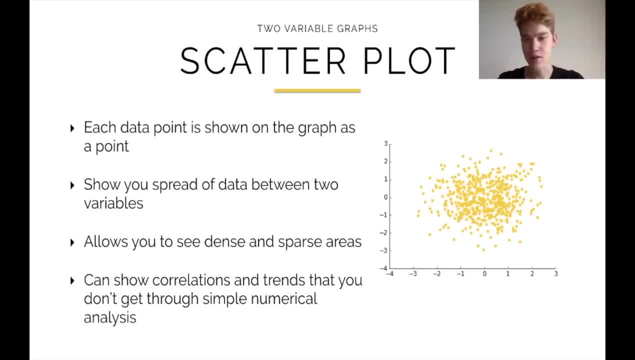 great because they allow us to see spread of data between two variables. so we're always plotting one variable on the x-axis and then another variable on the y-axis and then another variable on the y-axis, and it just pretty much allows us to see how the data is distributed for these two variables and 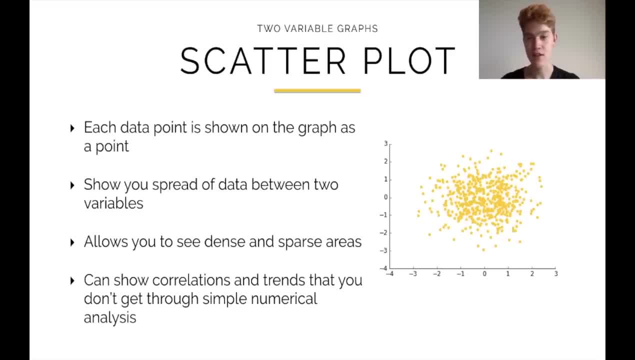 then through that we can also see more dense areas, we can also see some sparse areas and we can also look at correlations. so maybe you remember in the lecture we talked about correlations. we were able to see through scatter plots, where those correlations were or where there weren't. 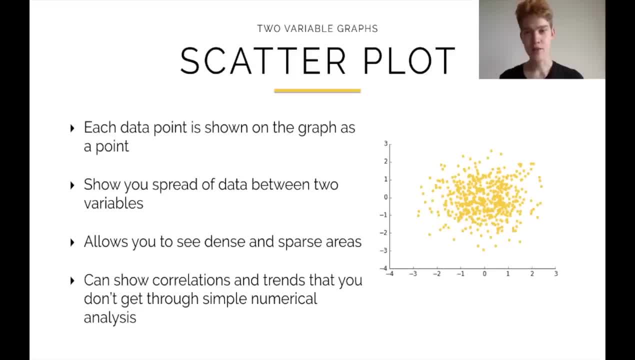 any correlations. so all of these things, that's what scatter plots are really, really nice for. and scatter plots, of course, we can also use them to have, like we see here, little clusters. so not everything needs to be connected by a line or a curve, maybe something is more like a circle, and 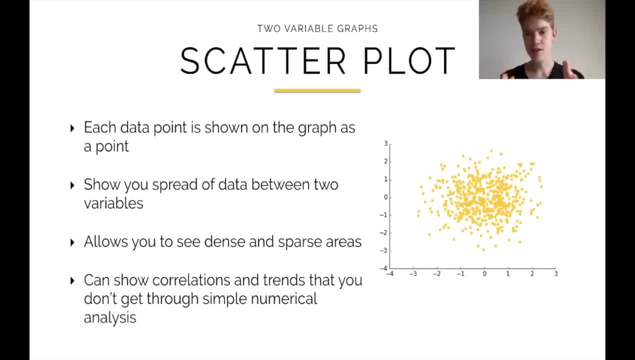 so that's what scatter plots can show us too. they can kind of show us these groupings and we see one cluster here, but maybe you know, you have bigger plots and then there would be smaller. you know like ten little different groupings for different things. so scatter plots are really great for that. 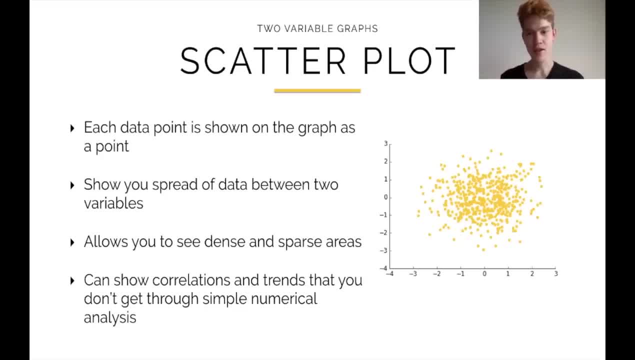 because they just show us where the data points are located and then you can kind of see how they are located for these two variables and then we can you ourselves see, you know like how, how do these look like? do does one variable affect the other? is there maybe certain groupings that we 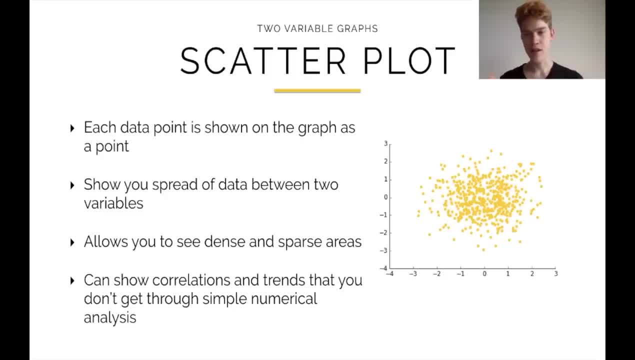 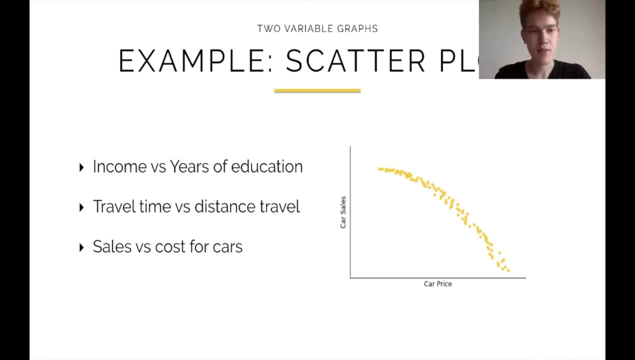 can see where are dense areas, where it's sparse, where are things concentrated, you know? is everything spread up all over the place? is it very, very narrow and only in a specific region? scatter plots allow us to see all of these things very easily, and so some examples where we could use scatter plots: 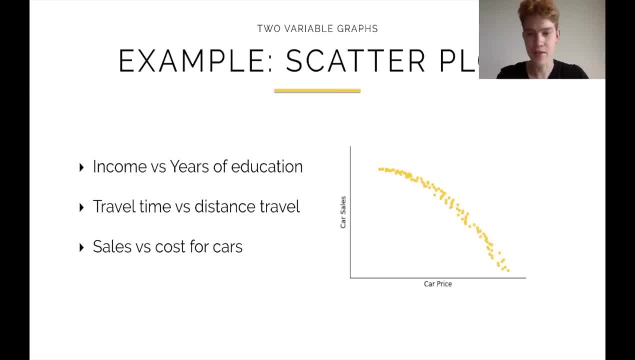 would be if we see a scatter plot and we could use a scatter plot and we could use a scatter plot and we can see. if we look at the graph on the right, we can look at something like a car price versus the number of cars sold. so each of these data points pretty much represents a car. that's. 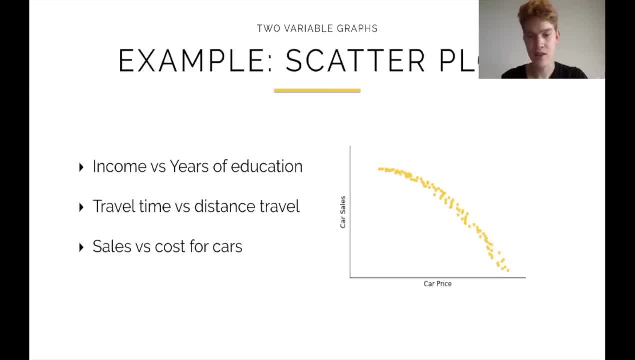 been sold, and then the x-axis tells us the price that the car has been sold at and the y-axis tells us the number of cars that the that have been sold at this price. and so what we see here, for example, very easily is that the more the car is priced, the less it gets sold. and then maybe you can think of: 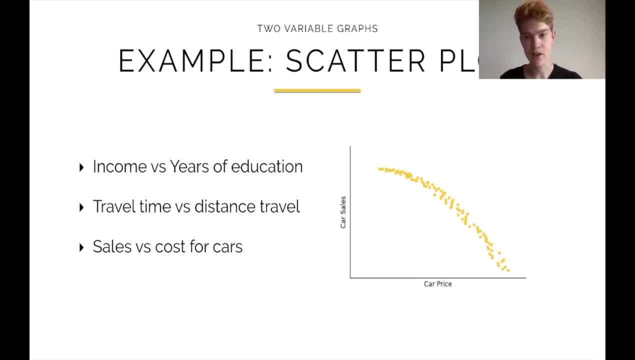 well, the more it's priced. maybe people don't want to buy such an expensive car. maybe they found a cheaper version of it, so maybe it's just a branding thing, which is why it's more expensive. maybe there's something just as good quality that's cheaper. maybe people just don't have. 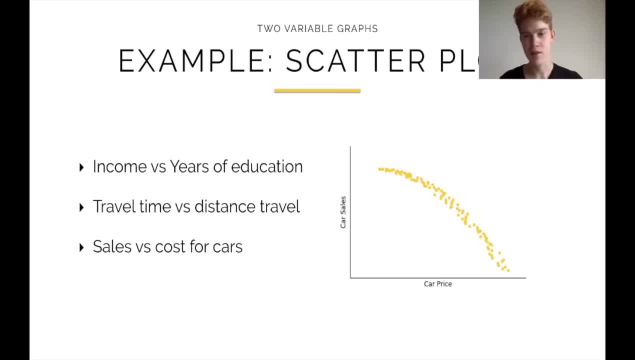 enough money. so that's probably a big factor too, that people just don't have enough money to buy these expensive cars, and so that's why they drop off, and so it may look a little bit different in terms of profits, but the higher the car is priced, the less we see it. 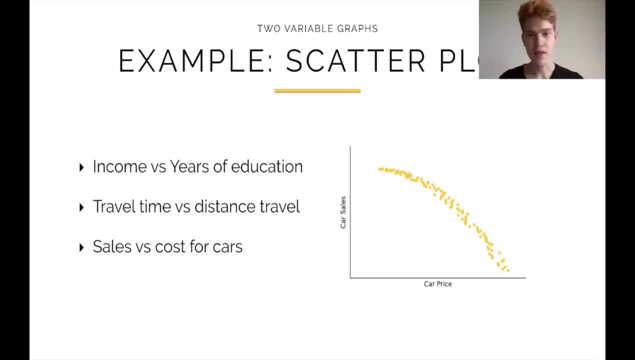 being sold. so that's one example of a scatter plot. then something else that we can look at is maybe the income versus years of education. so on the, we would look at on the x-axis how many years someone has been educated, and then we would look at the current income, and that would just be. 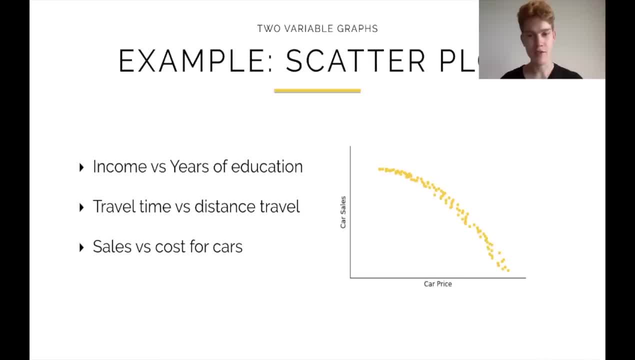 a point on the, on the graph, and we can do that for many, many different people, and then we can see how different education for different people, how that affects their current income. so that's another thing where we can do a scatter plot, for we can also go back to one of the earlier. 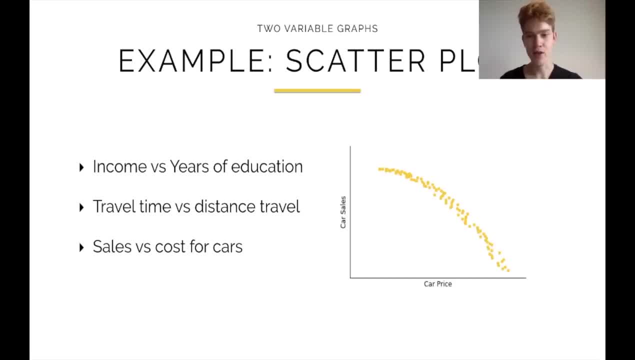 examples that we used very early on, where we talked about people traveling to work, and we can just plot the distance traveled versus the time it takes them to travel to work and then we can see. you know, maybe some people travel faster. it could be that some people travel the 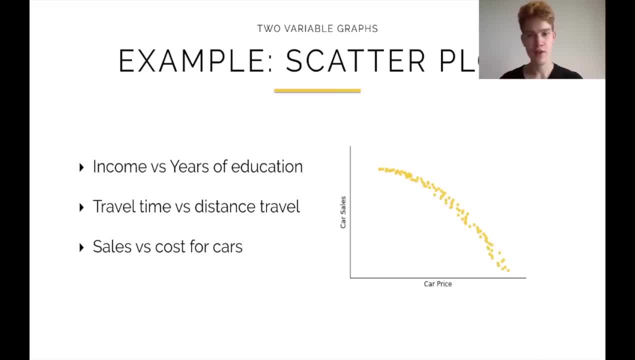 same distance but one takes longer than the other because one goes by car, the other one goes by bike, the other one takes public transport. all of that is a point on the graph. so that's another thing where we can do a lot more of this analysis. so when we look at our charts we can see that. 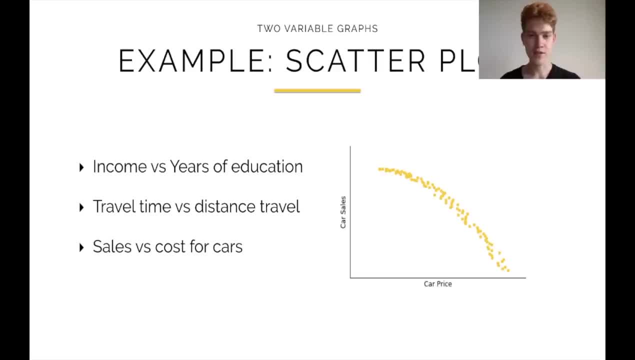 there's a lot of different reasons why people travel between different regions and that you can see, that's why we're using a lot of these things. so all of that we can see in these scatter plots and just kind of take into account these different situations and see how that all looks. 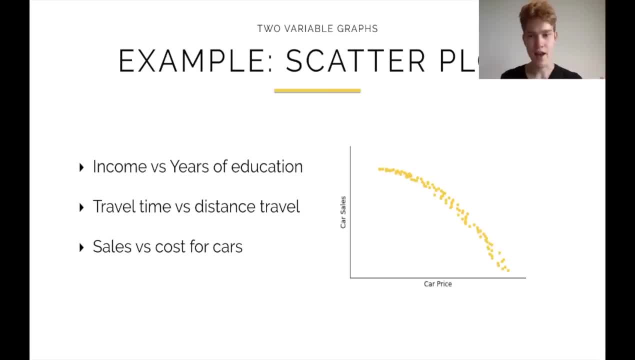 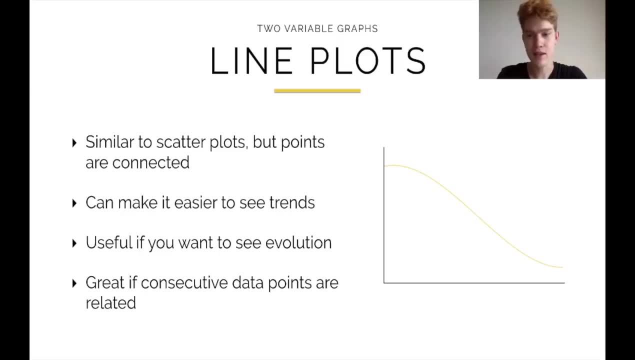 for the general population of our data or just generally for our data. so scatter plots are really really great as a kind of first go to just also identifying trends, identifying regions and just giving a good overview of your data, kind of similar to scatter plots. so we have the same basis of the X and the Y. 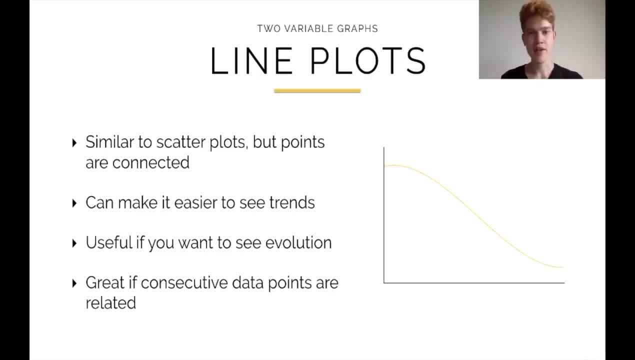 axis, but the points are connected and now it's very important to know when to choose line plots and when to choose scatter plots. so line plots can carry a lot of advantages with them, because this connectedness it makes it very easy for us to see trends, because we can see where these lines go, not just trying to. 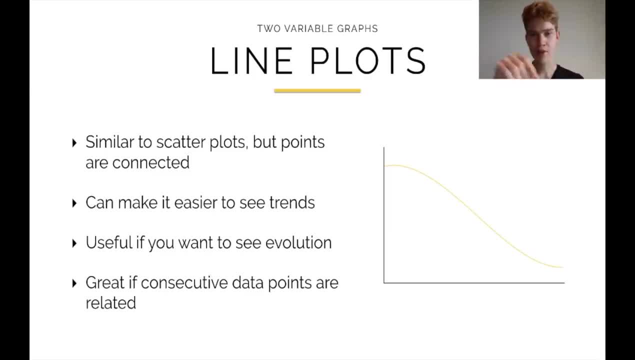 connect the points in our head, you know like kind of connect the dots. but that's exactly what a line plot does is it connects the dots for us and so we can see these lines. it's great if we want to see an evolution of something. so maybe we want to see an evolution over time, maybe we want to see an evolution. 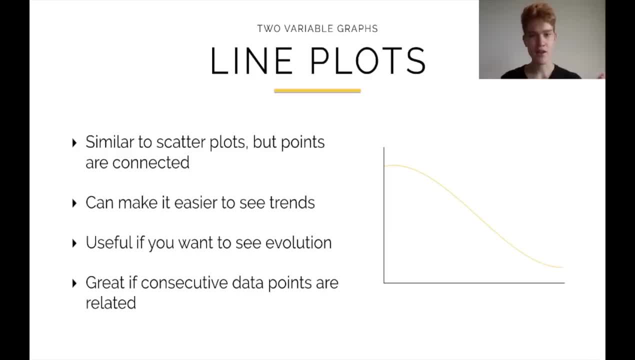 over space and evolution with people, something like that. just if our data points are connected, it's great to use a line plot. so if we know that whatever happened before is connected to what happens now, it's great to use line plots. because line plots show us how things evolve, because they're all connected as 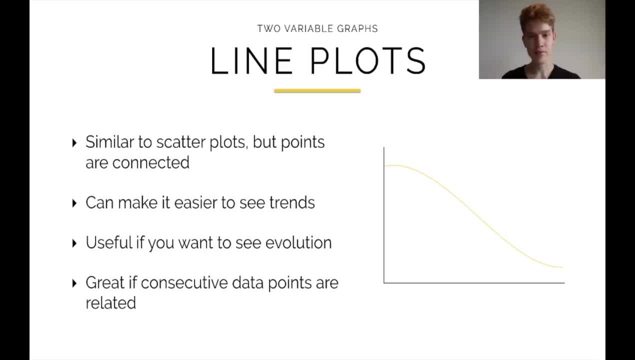 a line. but if we're to do scatter plots ��를 and we just kind of plot points randomly And just because, if we go back to our kind of car sold car price example, just because someone bought an expensive car, or if we look at the expensive car, 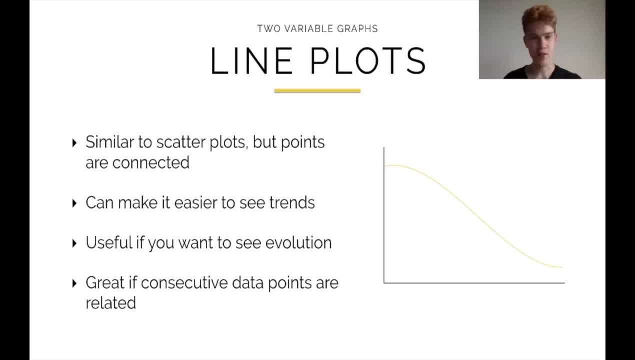 and it's been bought, say, like five times, and we look at a cheaper car, it's been bought 100 times. there isn't really a logical connection to make between the two, And so if we were to use line plots, where we should use scatter plots, 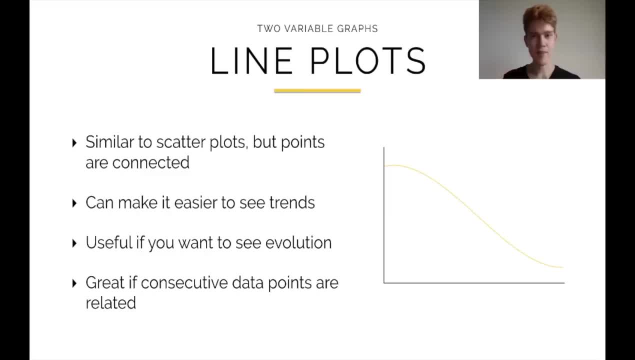 really what we'd see is just a bunch of lines all over the place, And so that's why it's important to kind of know when to use line plots and when to use scatter plots, because it can be very, very helpful If you use a scatter plot instead of a line plot. 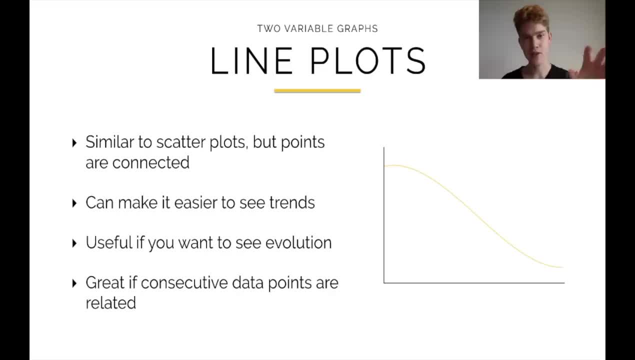 it's gonna be a bit more confusing because you have to try to connect the dots yourself in your head. But if you use a line plot instead of a scatter plot, it's gonna look really weird because there's just lines all over the place and you can't really see anything. 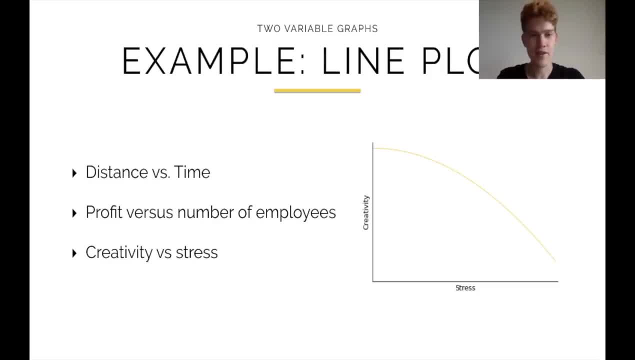 So an example where we could use line plots is we have the typical distance versus time, So you can look at how far someone or what time it is, and then how far someone has traveled- just a general curve of distance versus time. that's very, very common. 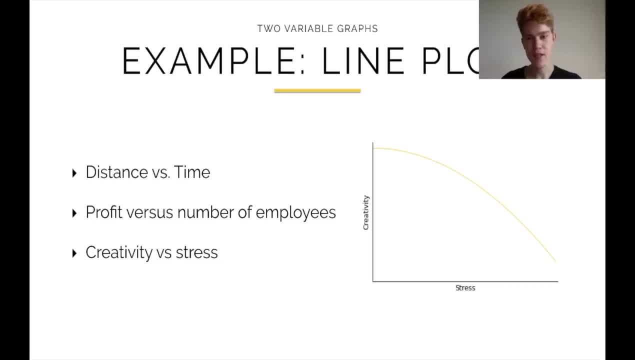 You can look at the profit of a company versus the number of employees. So the more employees they employ, how does that change their profits? So of course they have to pay the employees more. but maybe the employees can also do more work and hopefully that kind of cancels out what you pay them. 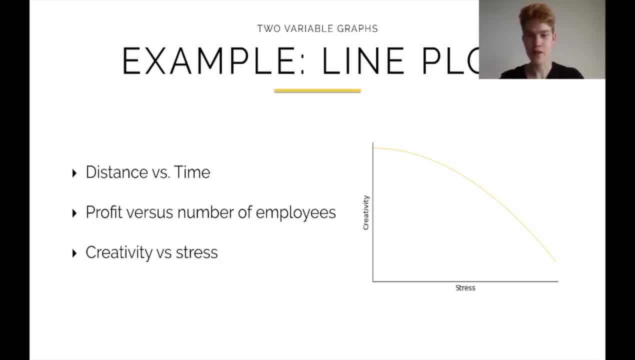 and then increases company profits. And then what we can see on the right here is we can look at your creativity and how that changes with stress. So we can see that the more stressed out you are, the less creative you are, And here it's also good to use a line plot. 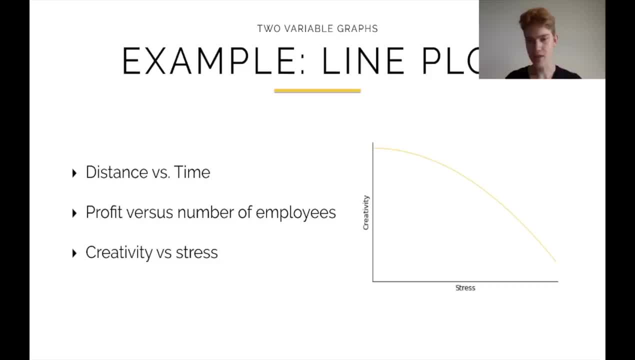 because you kind of gradually advance in stress, And so each point in stress is kind of related, and the higher you go up in stress, the lower you go down in creativity, And so there's this kind of relation where we can see this evolution. 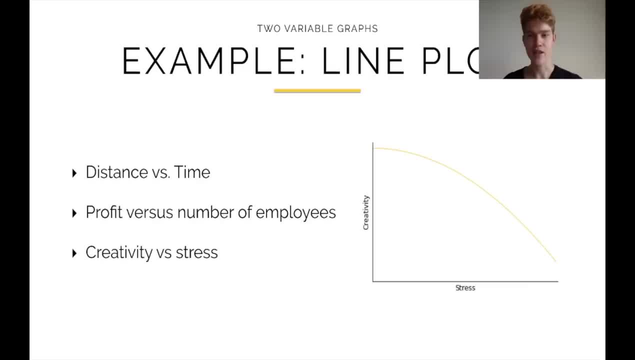 So the more you get stressed out, the less creative you become, And so line plots are really nice here, because there's not this chaotic movement everywhere. but it's very nice and it's very easy to see this line. It's very easy to follow. 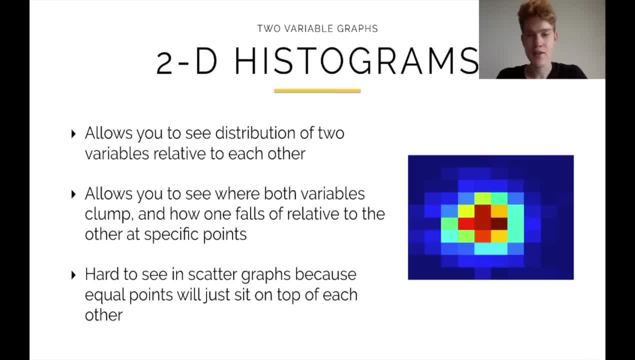 Okay, so the next graph that we can talk about is two-dimensional histograms. Now we've seen one-dimensional histograms in the last tutorial, where we looked at the spread of data and we looked at the peaks and how things were distributed to the right and to the left. 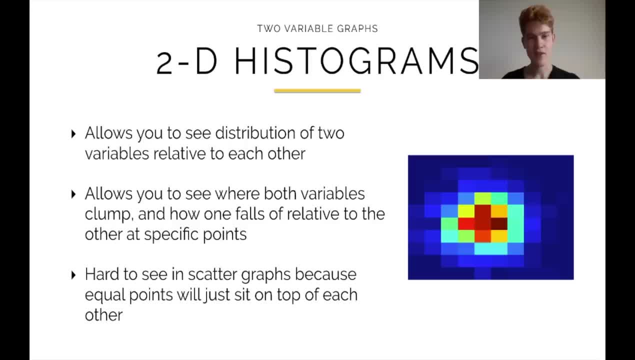 but we can also do a two-dimensional histogram, And so what a two-dimensional histogram is? it's a one-dimensional histogram, but it's a pretty much a histogram for every single point of the other variable that we're looking at. So, really, what these things allow us to see. 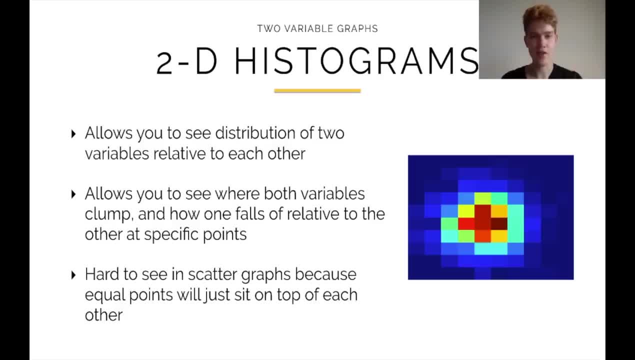 is they allow us to see how the different distributions of the two variables relative to another. So we can see here, for example in the red region, that for those specific values they happen a lot, So that combination of values happens a lot. 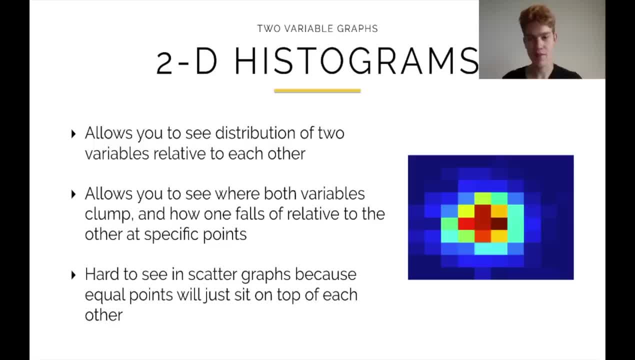 And so we're able to kind of pinpoint these frequency occurrences again and we're also able to look at drop-offs. but we're able to pinpoint that to two specific values now rather than just one, which is what we did to the 2D histogram. 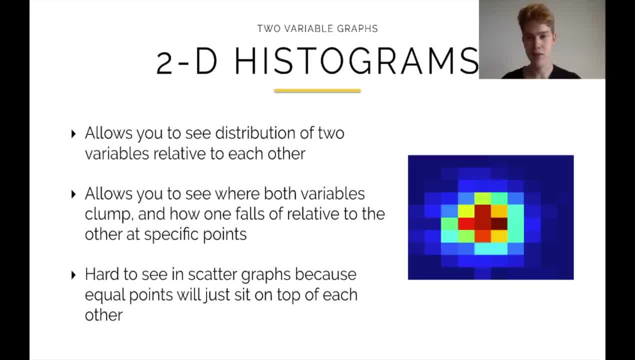 And these things are much harder to see in scatterplots, because in scatterplots, if we have a value occurring a hundred times, it would just be the same dot and the dot wouldn't get bigger. Now, of course, you can make the dot bigger yourself. 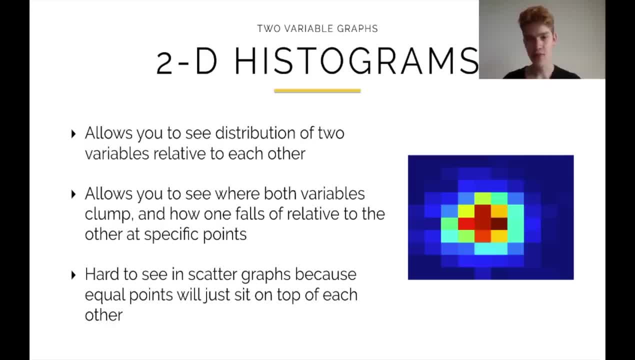 if you wanted to, Or you could change the color or something like that. But really, if you do a scatter plot and the same thing happens a hundred times, it's just gonna look like one dot, Whereas for two-dimensional histograms we can see that it's not just. 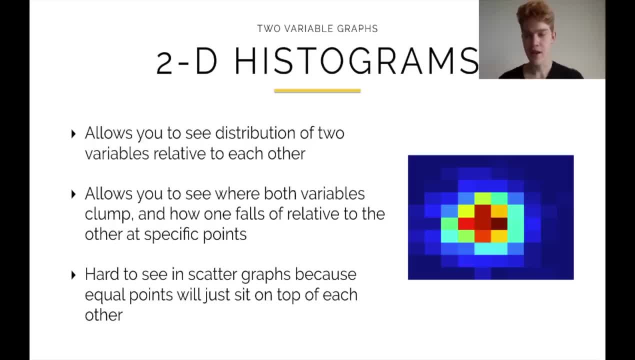 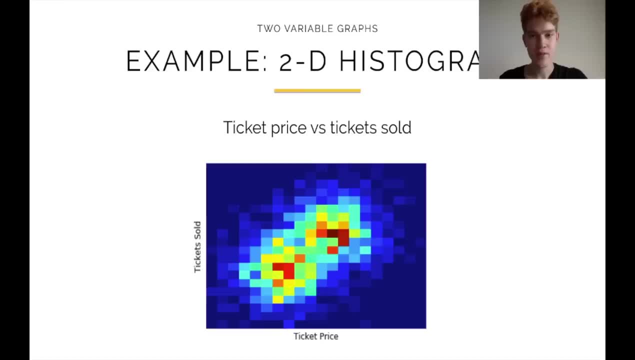 it's not just happening once, but we can actually see the frequency of those variables or those two variables together. So an example of a two-dimensional histogram would be if you look at ticket prices versus tickets sold. And so if you look at a ticket prices, I'm gonna add up two. 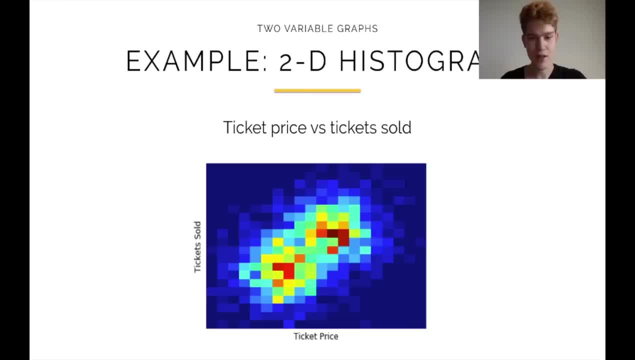 of those variables. I'm gonna multiply that by three. you look at the lower left corner and we can kind of see this red peak. so that's cheaper ticket prices. but the tickets are also sold often, so we know that tickets at that price are sold quite. 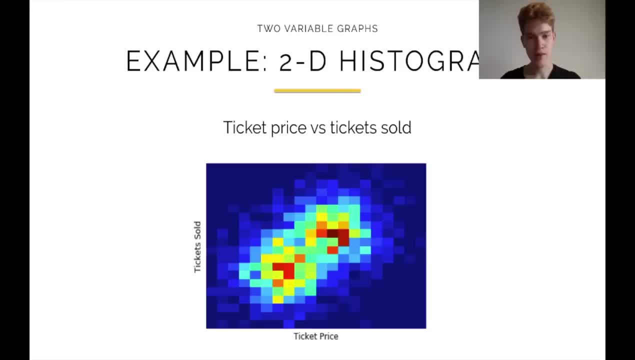 often, and these could be, you know, like new rising brand bands. these could be, like you know, you kind of standard bands that maybe you want to take someone on a day to but you don't want to spend too much money on a ticket. but still, a concert is a nice idea and so that's a good ticket price. 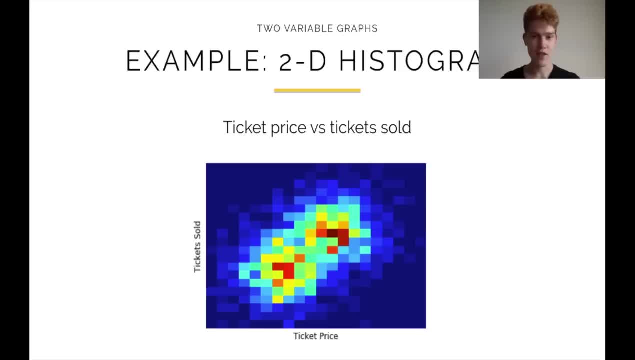 and that sells a lot of tickets because it gives you the pleasure of the event without making it too expensive. and then if you move more towards higher ticket prices and then if you move more towards more tickets sold, then you can see that for high tickets, high ticket. 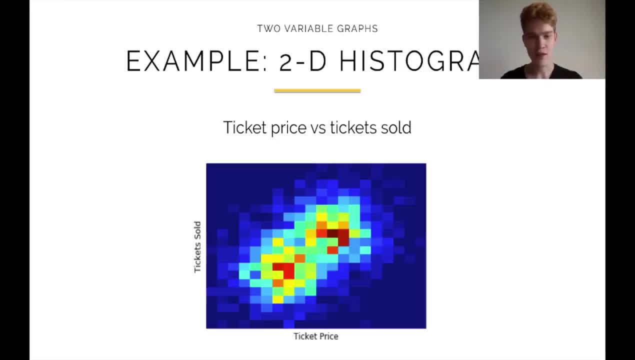 prices which would be, you know, like these big bands, then we can again see how many tickets we've sold. so we can see that for you know, a higher price and if we go up in tickets sold. so if you want to see like a higher ticket price, then you can see that for a higher price, and if we go up in 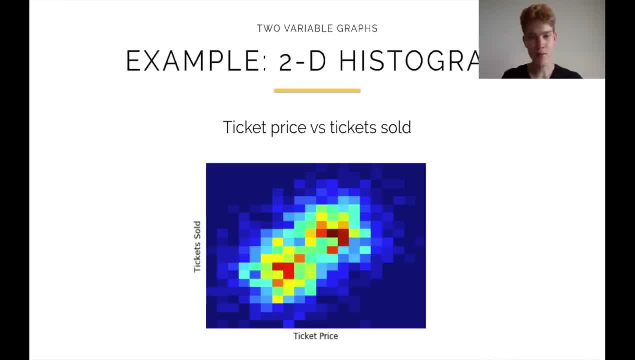 lots of tickets sold for a high price. then the red peaks are going to give us all of these more famous artists. so that's, you know, one kind of application, but of course there are many, many better ones. it's just these things, you know, if you're in the moment and you, you can kind of then. 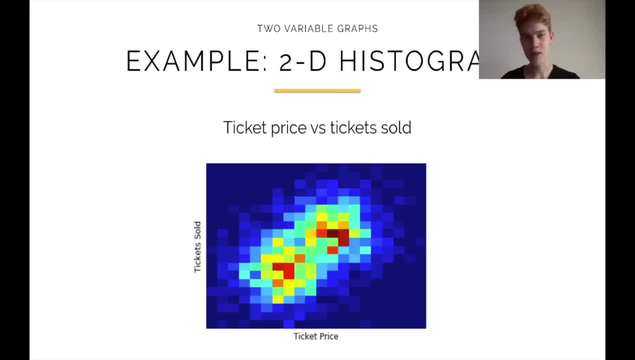 you would realize: oh, this is when a two-dimensional histogram would be a great thing for me to use, so a lot of these graphs. they're great to know, and once you're in the moment, then it's much easier for you to pick out which graph would be the best for you to use, and so that's a good thing for me. 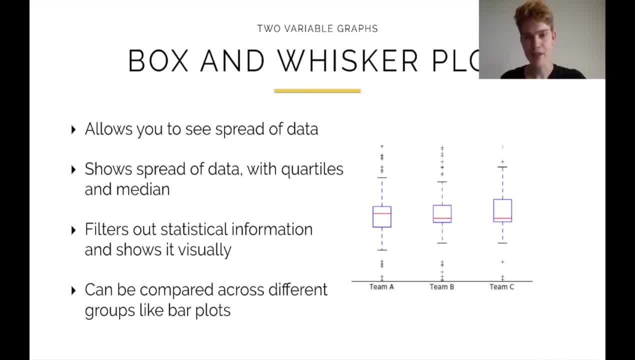 which graph would be best representative? finally, the last graph that we're going to look at is going to be a box and whisker plot. and now, what box and whisker plots allow us to do is they allow us to see the spread within our data. so it's not just like a bar plot, which just shows us one value, but 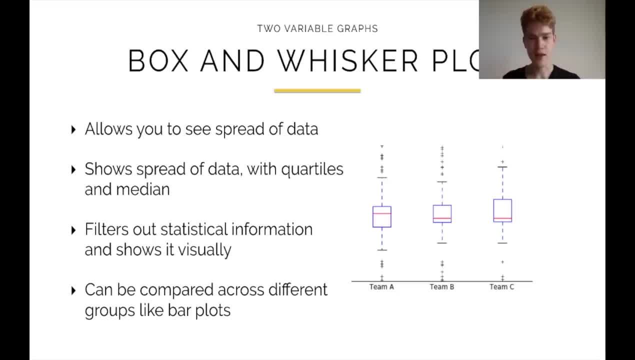 we can actually see the statistical spread, so we can see median values, which is what we see here. we can see quartiles. the little dots on the outside actually show us outliers, and so what box and whisker plots allow us to do is they allow us to see the statistical information, but they allow us. 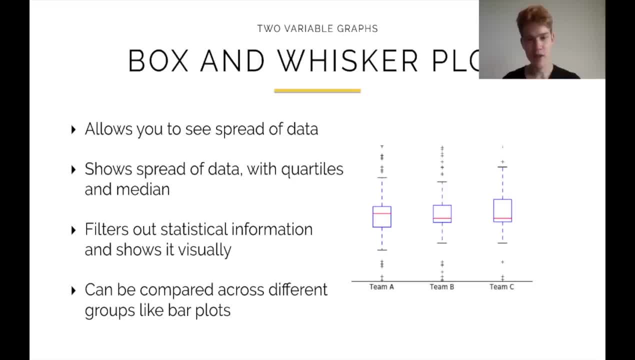 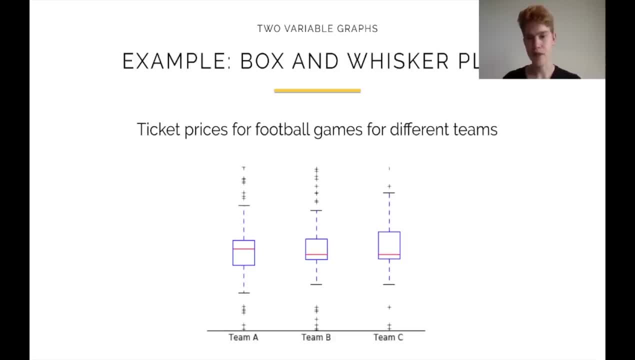 to see it visually, and that makes comparing across different groups, which is what we're doing here, much easier, and so a good example of that would be if we look at ticket prices for football games for different teams. so we have different teams and different teams, of course, use different stadiums. 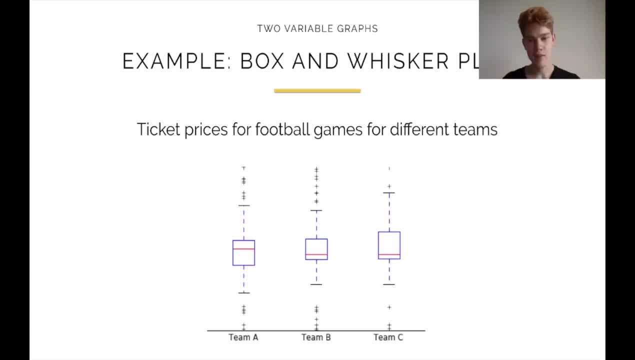 and their. they have different popularities and some teams may be much more expensive or the ticket prices may be much more expensive than other ones are in terms of interest, and that just sort of shows. and so we can compare these ticket prices using box and whisker plots and then we can see. you know, 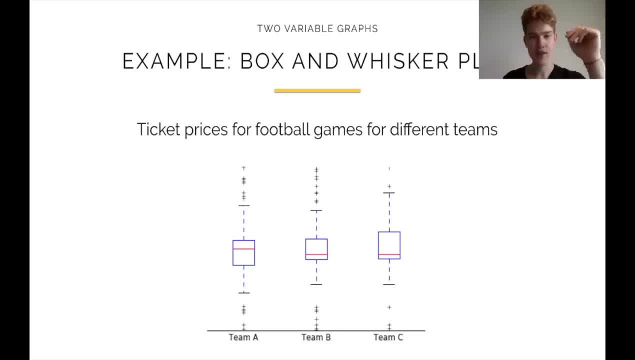 what is the higher end of these costs? so those are going to be the more luxurious seats. and then we go to the bottom and those are going to be the less luxurious seats, probably the ones where you stand, and then you have middle values depending on you know, the standard seats and where you are. 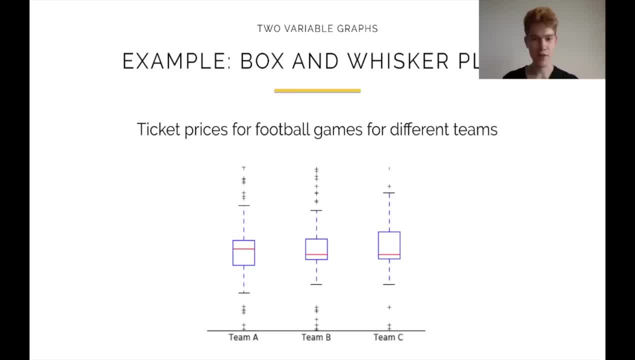 in the stadium, if you're close to the field, if you're further away from the field but you're still sitting. all of these things we can kind of see here and that's what gives us a spread. we can compare that across different teams and we can see the spread across different teams. we can 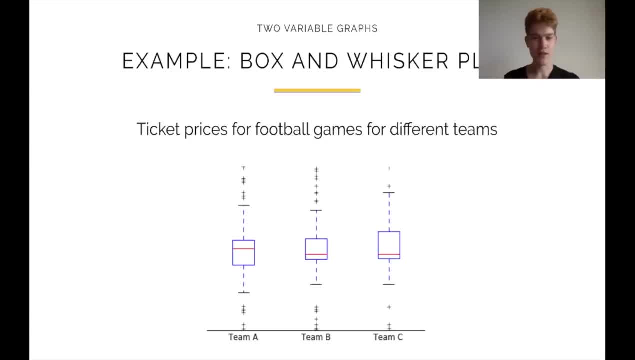 also see which teams are more expensive. you know, where do the prices vary the most for specific teams? so maybe some teams have a super launch and then they have your- you know- standing places that are just much cheaper, and so you would see a much more larger spread. or maybe some teams just have 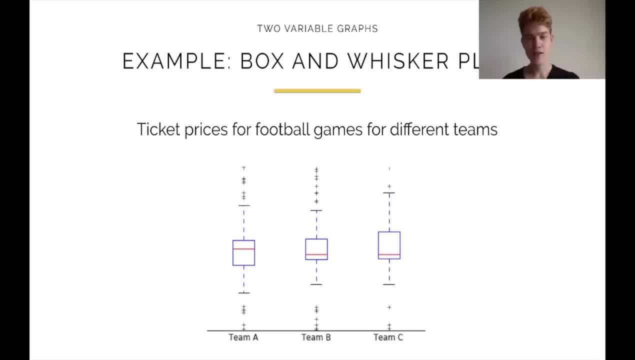 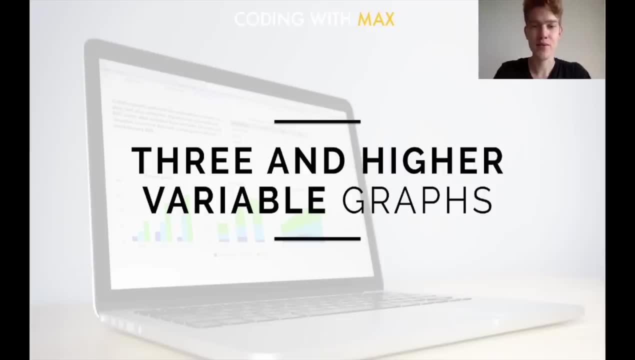 you know only seats, and so you'd see a much lower spread, and so all of these things we're able to compare using box and whisker plots, and then we can compare that across different teams and we can score plots over different groups. in this tutorial we're going to talk about three and higher. 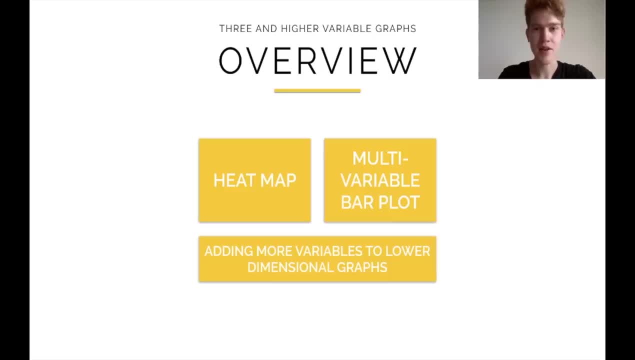 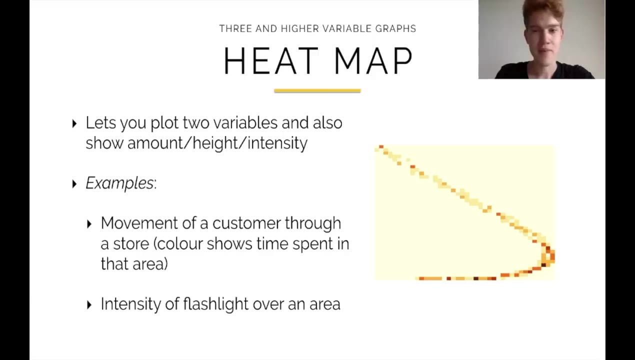 variable graphs. so the graphs that we're going to look at is going to be heat maps, and then we'll also look at multi variable bar plots, as well as how we can add more variables to some of the lower dimensional graphs that we've talked about earlier. alright, so let's start with heat maps. now what? 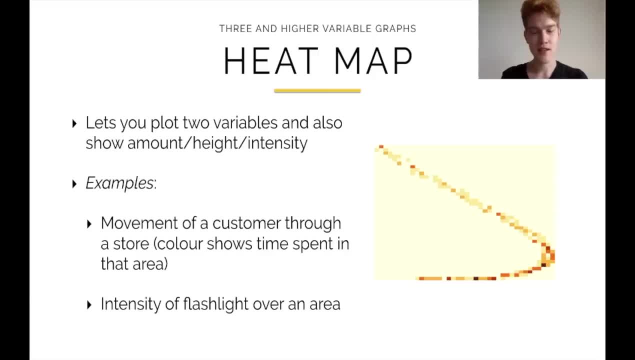 heat maps allow us to do is they allow us to plot two variables against each other, in the X and the Y, and they allow us to show an or a size or something like that in the Z direction or towards us. so an example of this, which is kind of what I've tried to illustrate on the right, is a customer. 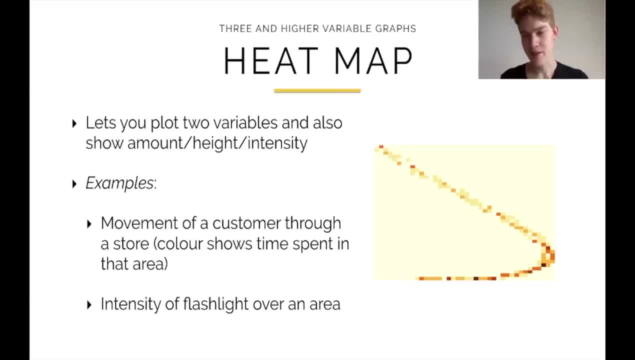 moving through a storm and so we can track the path of the customer in the X and Y direction of the store. so you can kind of get this bird's-eye view and see where they move to, and the darker spots actually tell us the positions where they spend more time at, so we can see that they spend a little bit of time you. 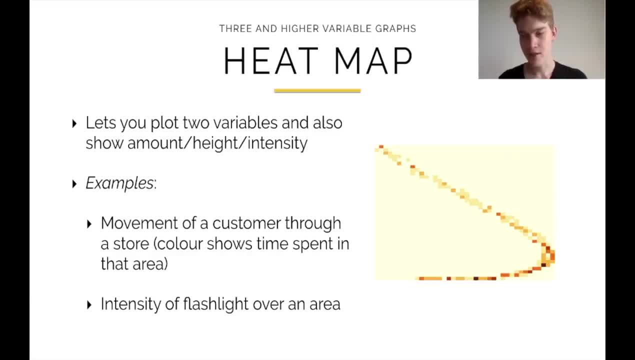 know, at the beginning they moved in and then they stopped. once was what we see the dark spot being. maybe they found, like the candy aisle or something, there was a specific piece of candy that they wanted, and then they moved on and then they started to go towards the corner, around the corner a little bit, and maybe 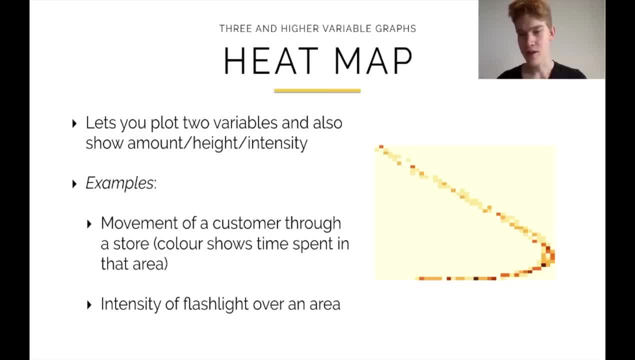 they reached the fruits and vegetables section there and picked out several things, and then they started to head towards the checkout counter, which happens at the very end, and they were moving at a more constant pace. sometimes they stopped to look a little bit, but they just kind of continued moving on. 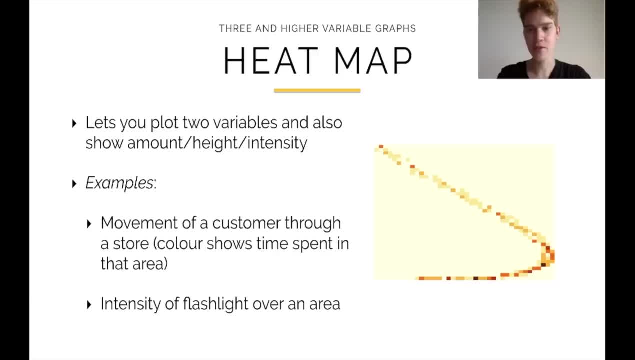 and so the three variables that we've shown here is: we've shown their X position in the store, we've shown their Y position in the store and to the color, we've also shown the time that they spend at each position. so that's what we can use: heat. 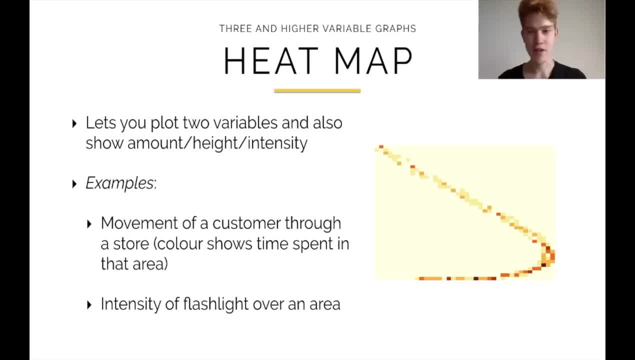 maps for. and then another example of a heat map would, for example, be if you take a flashlight and you move it over the screen and really what you're showing is the amount of time that you've shown the flashlight onto a specific region. so that's kind of another example of a heat map. but 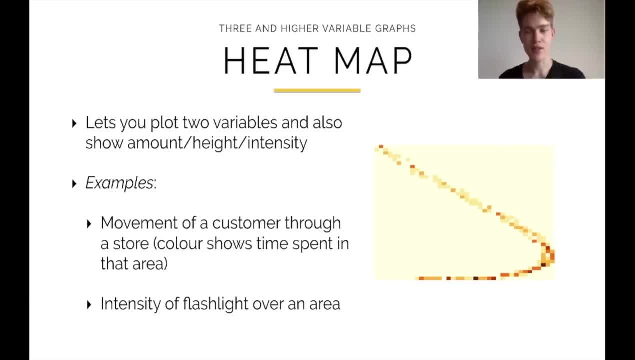 heat map. as the name implies, it allows you to track positions, and so it's very often used for things like tracking customers through stores or just tracking general popping people location where they like to spend their time, and the intensity that you see in terms of the color is usually the amount. 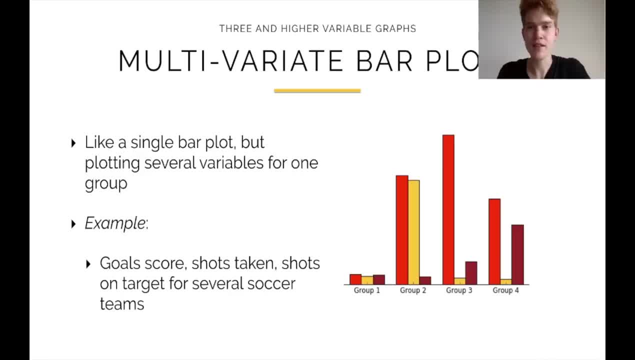 of time that they spent there. alright, so we can also do multi variable bar plot, some multivariate bar plot, and so it's very similar to a single bar plot, where we just pull it up to the left on the right side and then we can see if it just 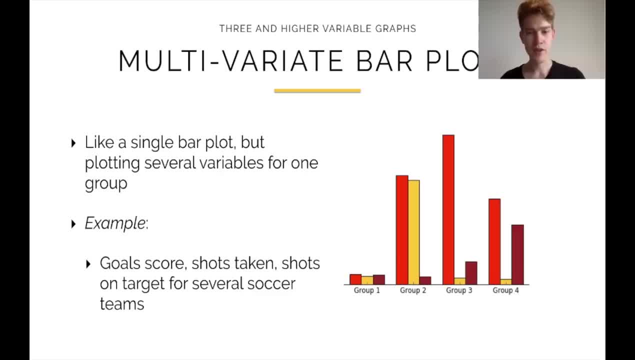 looks the same, so we just move it around and see if we've shown the same thing: one value over different groups. But rather than just plotting one, we kind of cramp them together and we plot several, And so an example of this would be that we plot, you know, goal scores. 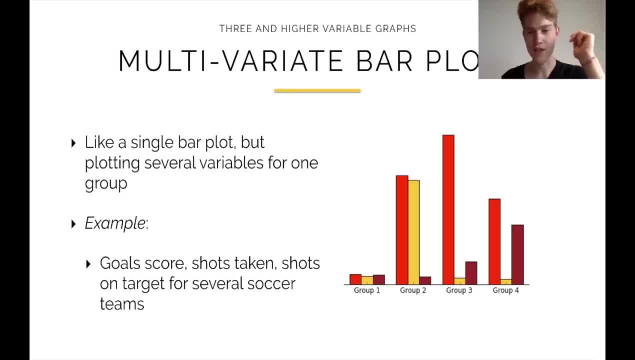 goal scored for team, the shots taken on goal as well as the shots on target, And so we can see: maybe there are teams that shoot less on goal or that score less, but that's because they also shoot less and therefore they also shoot less on target. Or maybe there are some teams that just 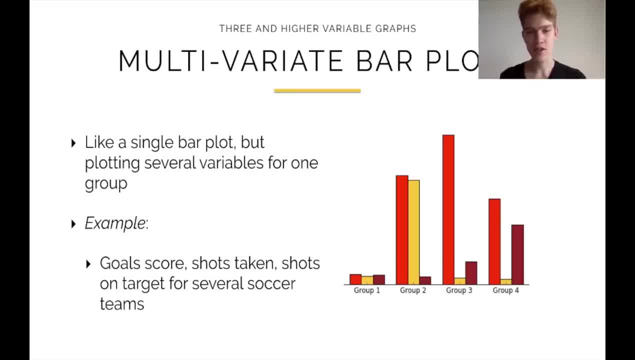 score a lot And that's because they shoot a bunch but they just don't hit the target that often. Or maybe there are really good teams that score a lot and they also shoot a lot on target, And so all of these things were able to then compare over different groups, And so that's. 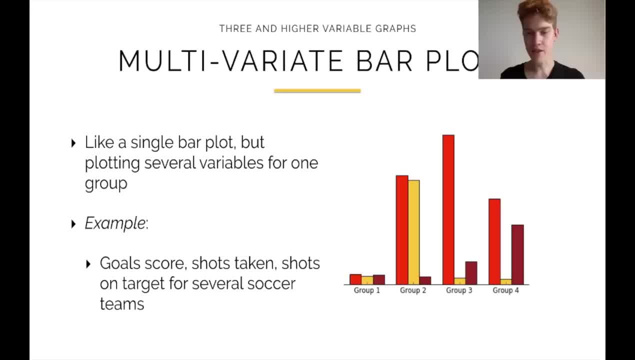 what we can use multivariable bar plots for. If there are several variables, that would give us a better understanding of the system than just looking at the variables one at a time. But it'd also be really cool if we could compare all of them. then we could, you know, we could just. 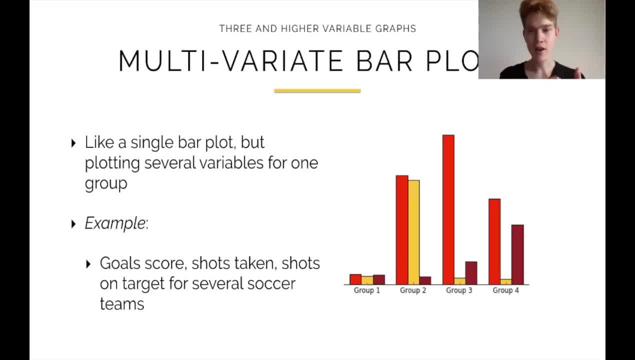 use multivariable bar plots for that and just plot them on the same bar plot And then we can see how they change, you know, within a group, but we can also see how they change over different groups. Okay, and something that we can do is we can also just add extra dimensions to lower. 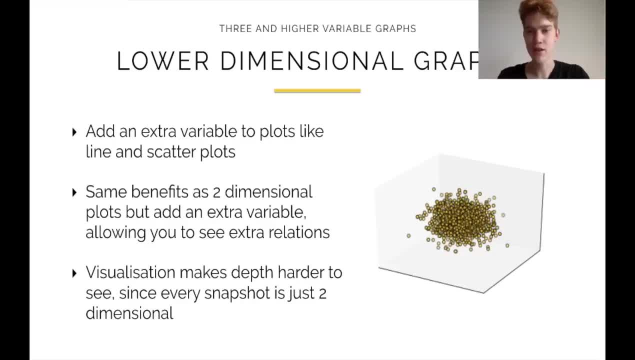 dimensional graphs that we've had And so we're kind of limited to three dimensions because that's the amount of space dimensions that we live in. But if we take the scatterplot, for example, where we started off with just the x and the y axis and points located, 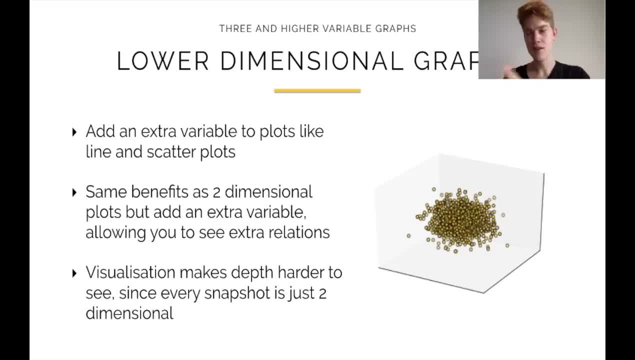 what we can do is we can actually add a third axis, So we can take the x and the y and then we can add a z, And that gives us an extra depth dimension, which is exactly what we see here. So, rather than just plotting on like a two dimensional field, on like a plane, we can actually plot it in. 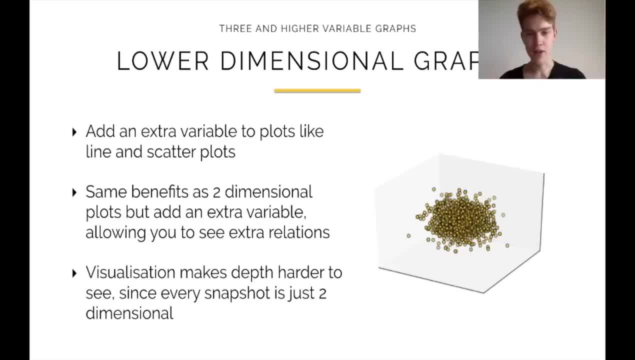 a volume, And so we can see this kind of scattered ball that we've done, kind of ball that we've done here, which is kind of located at the center of our plot, And so this can be really cool because it allows us this. 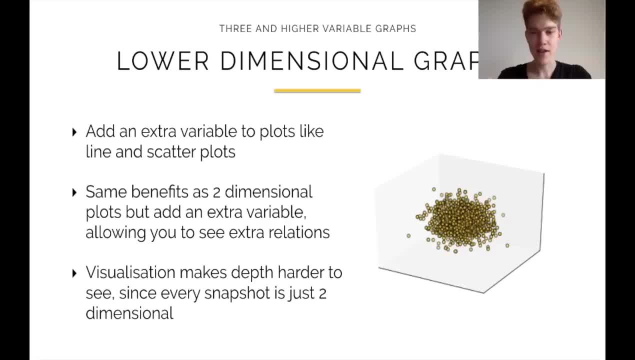 so, so, so. so see, depth to the problem with this is that we have snapshots every time, And so, really, we're looking at two dimensional snapshots, And so to get the best understanding of this, we need to rotate our scatter plots, or our plots as we do them, so that we can also add in our depth. 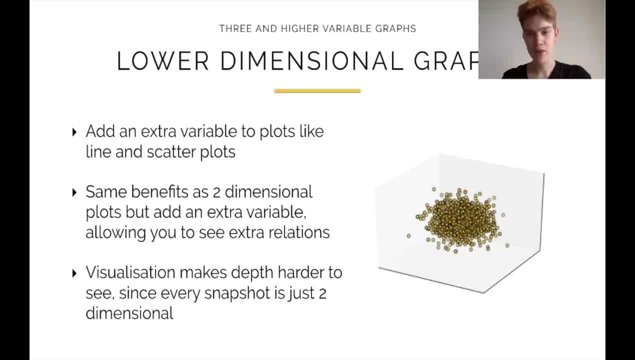 perception, Because right now, if we're looking at it, it may look three dimensional, but really it's just a two dimensional snapshot And, to get the best understanding, if our scatter plot is located more towards us and more towards the left or something like that, or maybe it's just- 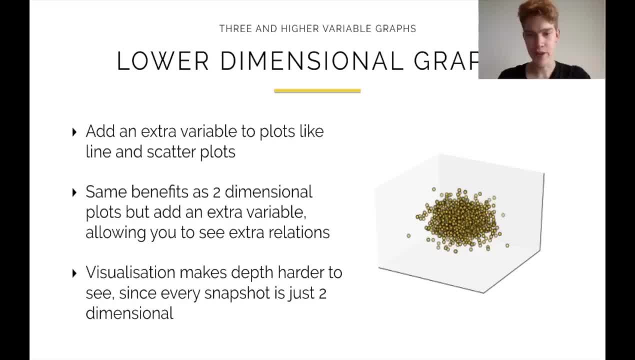 really high and close to us, or maybe it's really low and far away. To understand all of these things, we need to be able to rotate our scatter plot so that we can see it from different angles, which then gives us this depth perception, And we can do the same thing with 3d line graphs. So here, 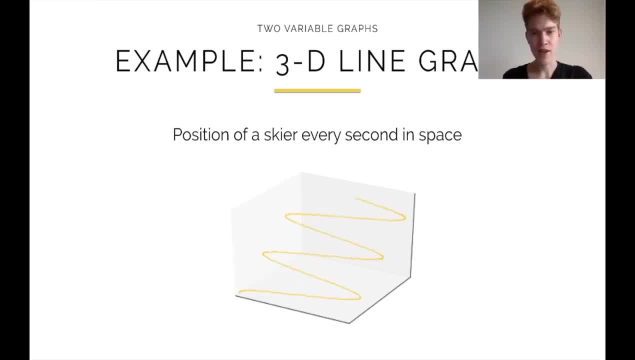 we see an example of, maybe, the position of a skier as they're skiing down a hill And then we can kind of trace that through time And we see that they're kind of they're going down the hill in this nice zigzag motion as you should and we can just track their. 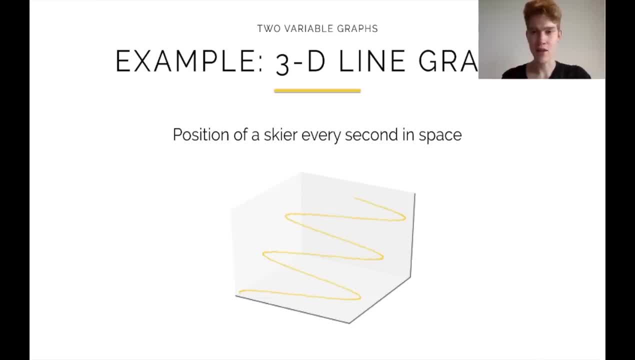 position over time. So here we've added this extra dimension to the 3d line graph. rather than just taking maybe a time and a position in a time or something like that, we've added a second positions or actually even a third position. So we've got the x, the y and the z position and then 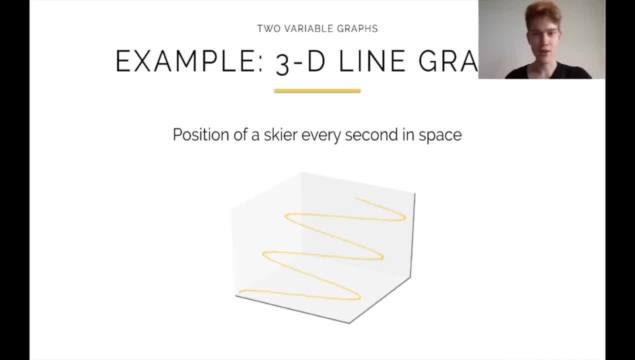 we just trace it over time, And so that gives us this whole line here, And so that's how we can take these lower dimensional plots that we've looked at before, And we can just add extra dimensions to them if we want, as long as it's still easy to see, as long as it makes sense what we're looking. 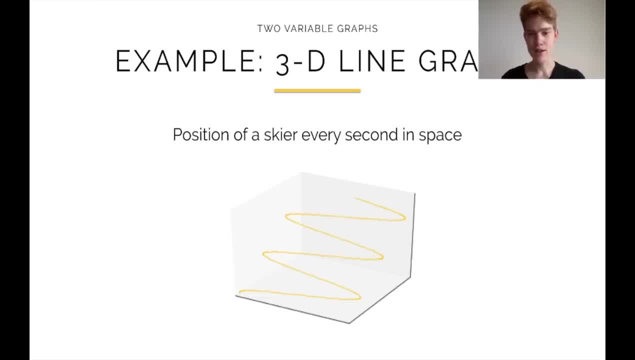 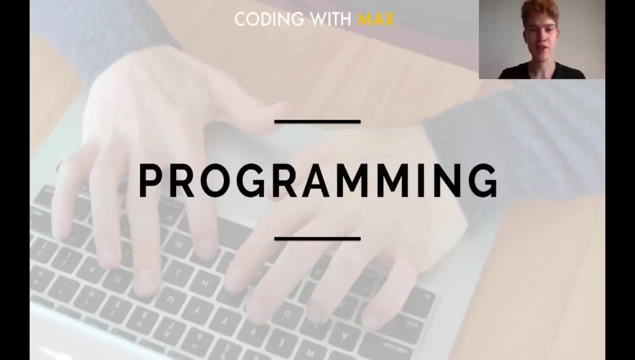 at. Yeah, we're really just able to maybe just slap on another direction there And, you know, compare another variable. In this tutorial we're going to touch on the third major section that is really great for data scientists- or that should be an essential data scientist- which is the. 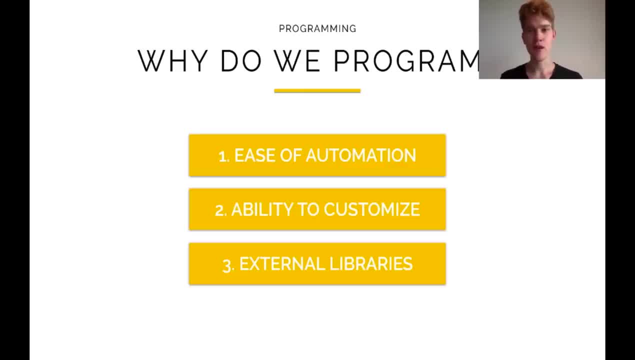 first one. So why do we program? Well, there are different reasons why we want to be able to program. The first one is going to be the ease of automation. The second will be the ability to customize And, finally, it's because there are many great external libraries for us to use. that. 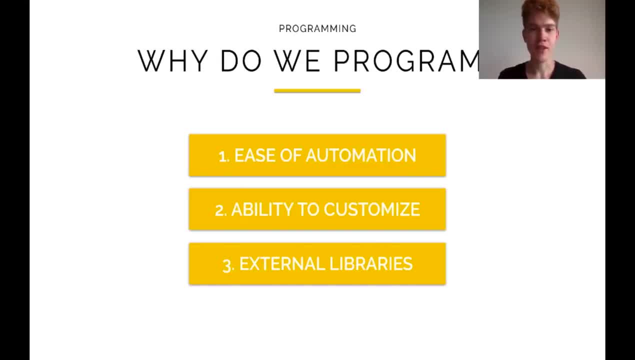 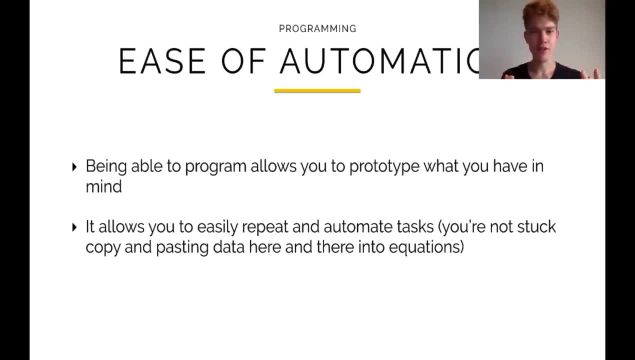 will just make our job so much easier. All right, but so let's get started. Let's talk about the ease of automation for us. What do I mean with that? Well, being able to program. it really allows you to prototype really fast, allows us to automate things. 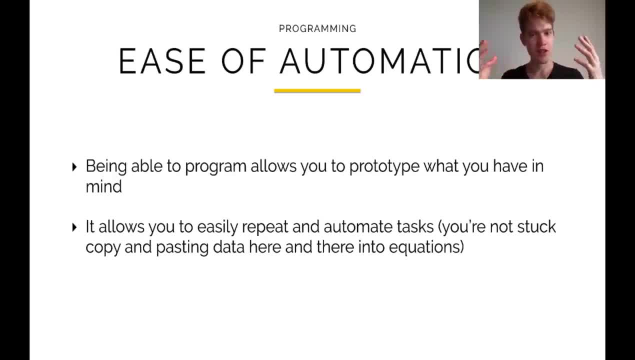 It also gives us the extra benefit of if we have something in our mind, we can just take that and kind of put it into the computer by programming it, And so we're able to automate everything very fast And we don't have to do these repetitive tasks. You know, maybe copy pasting stuff into or 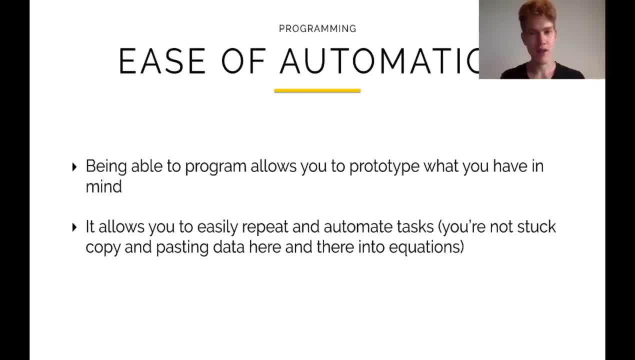 from Excel or all these things. If we just want to repeat something or we want to quickly change something up and just change a small thing, we don't have to do a lot of stuff. we can just change that in our code and then click play. 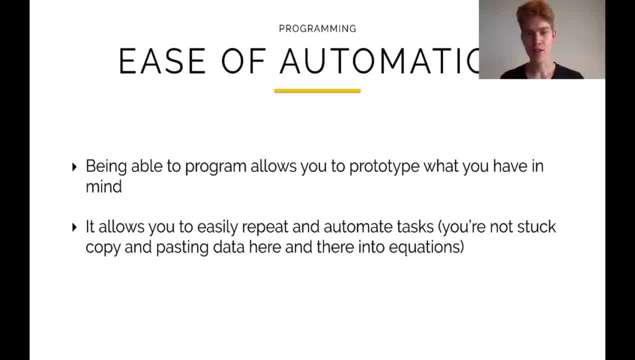 And let the computer take care of all of that for us, rather than us having to do everything manually. So it's very easy for us to automate things And also for doing reports. it's very easy to automatically create these reports. you know, all you have to do is set up your program to deal with. 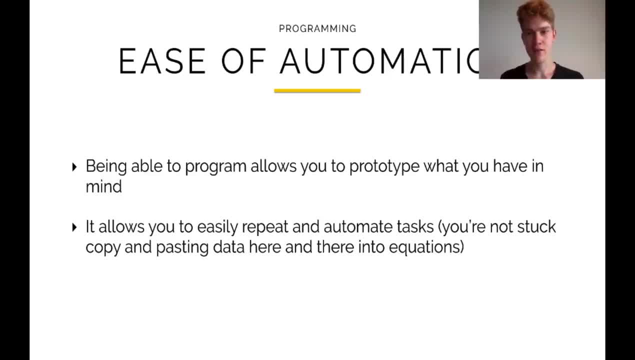 the data that you're going to give it And then it can automatically create reports every week And the reports can be different because you give it different data and it should still look the same, But the data, the values, can be different. 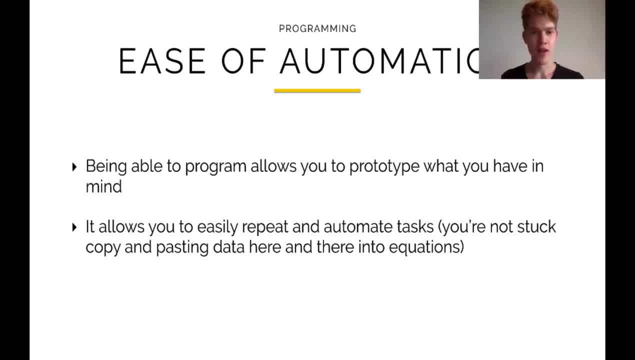 And so that will just be a little bit more complicated, but it's very easy for us to do that, So you can just automatically create all these reports for you And you don't have to do it all yourself. the program does it for you. But you've built the program and you're giving it this. 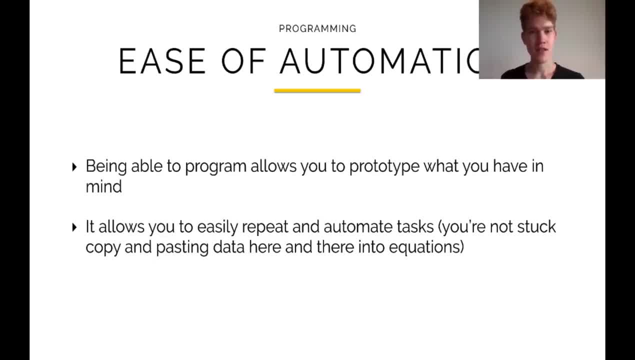 different data. So you're still doing all of the analysis. it's just you get to skip the part of copy pasting and like looking across and taking over the values and doing all the formatting, of just doing the same report over and over and over again. All of that is taken care of for you And 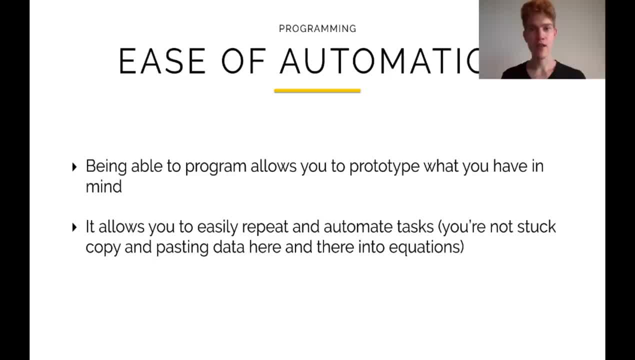 all you have to do is just put in the right data, you know, write out everything that you want to do and let the computer handle all of that for you, Because, remember, that's what the computer is doing good at doing, doing these repetitive tasks. Okay, we also want to be able to program, because it 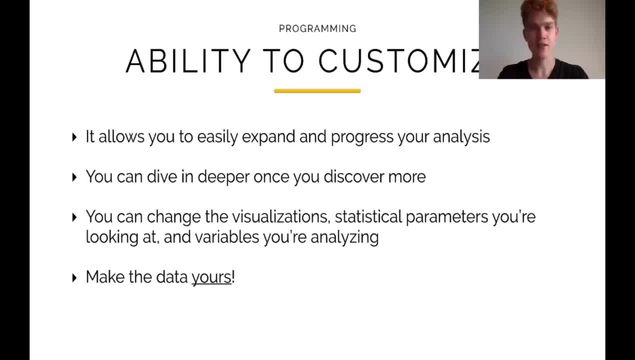 really allows us to customize. It's very easy once we go into data analysis And when we see things that we get these ideas that we want to expand or different directions that we want to progress our analysis into and being able to program. it really just allows us to take all that and put it. 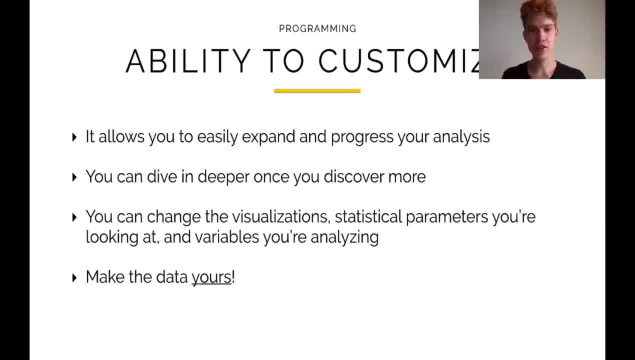 into code And just choose that direction, And we can very easily dive much deeper into our analysis and discover things fast, because it's up to us, to where we want to go. And so this ability to customize with programming- it's very, very important Because we're not reliant on anything else. We're not reliant on 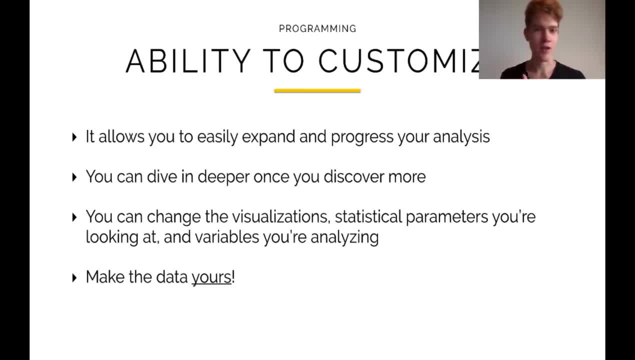 you know some software and maybe it breaks down or maybe we don't know how to perfectly use it and we have to read the manual and read it like a help section. And now we know how to program and we just type down exactly what we want to do, exactly. 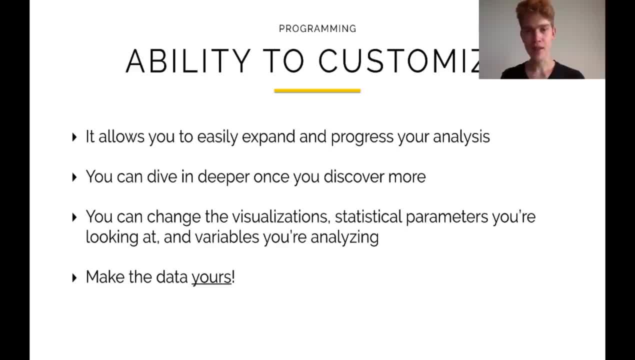 Where we want to take it, exactly what we want to see, And we can customize very, very fast with that. We can also prototype very, very fast with that And maybe, if a visualization is not working, to turn a scatterplot into a line plot is very easy. 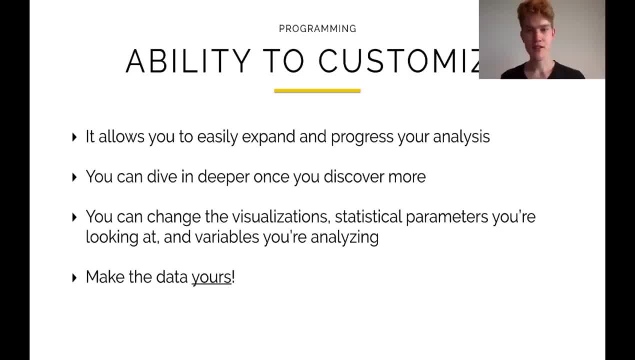 you just change one word. So all of these things are very, very easy to do with programming, because we have all that power at our fingertips And we can just, you know, change everything that we're looking at, everything that's being calculated. 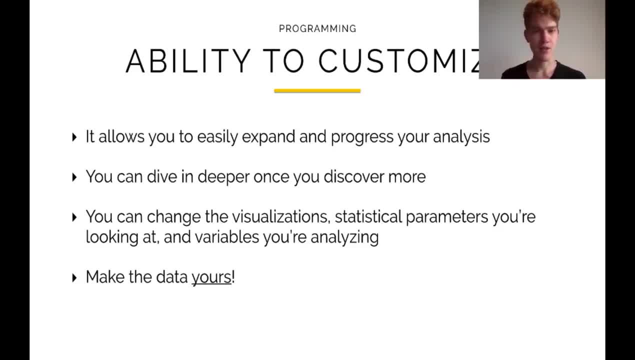 maybe we want to calculate an extra thing and take out something else, because it's irrelevant. all of these things we're able to customize and all of that we can do because we're able to program. so really, what we're doing is we're making the data ours, so we're taking full control of the. 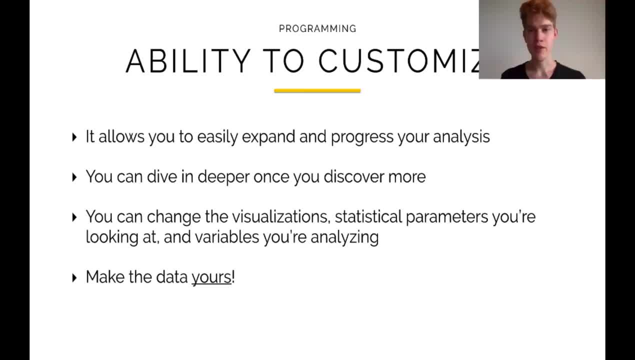 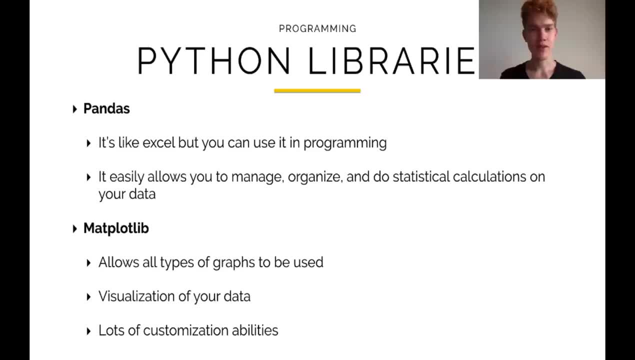 data, we're taking full control of where we want to go with our analysis, what we want to see and what we want to show. all right, so let's talk about first libraries, but also give you two great python libraries that you should- you know, maybe feel comfortable with, or that you should maybe. 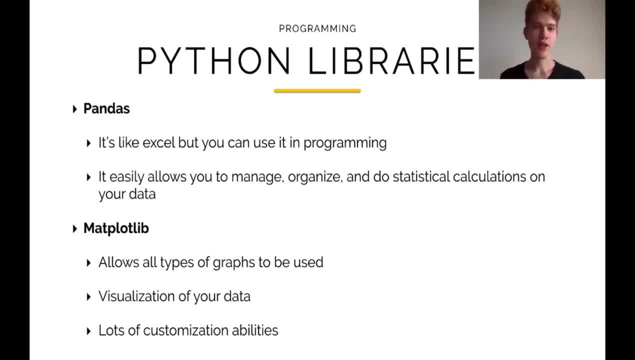 consider using for data analysis. so, first of all, what are libraries? well, libraries are pieces of code that have been pre-written by others that you can just take in and use, and so a very good example of this is something known as a math library, and so that has all of the square root functions taking 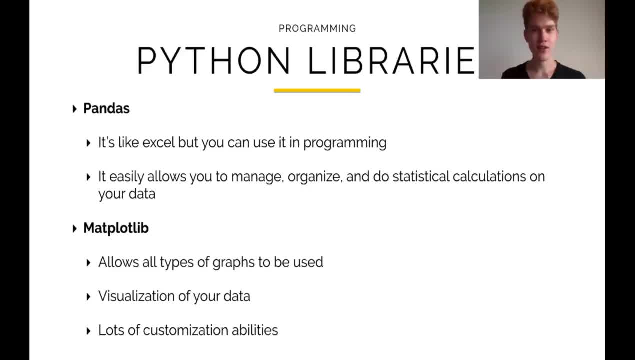 to the power you know, taking the exponential, the sine, the cosine, all of these things that you know and you want to use but you don't want to program yourself, so like it pretty much avoids that middle step of you. know you want to program yourself, so like it pretty much avoids that middle step of you. 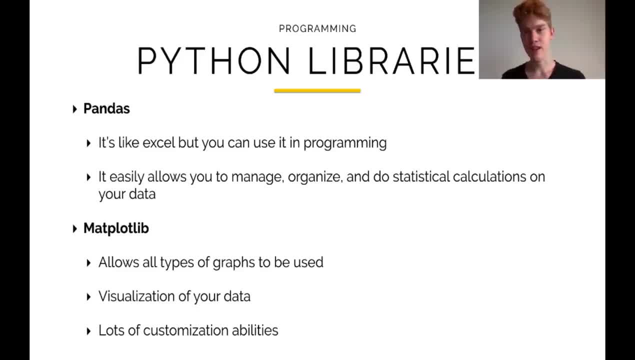 having to program the equation to calculate a sign, because all of these things, those are things that we don't want to do. we don't want to get distracted from our target. we want to be able to do exactly what we want to do without having to program completely other stuff, and so that's what. 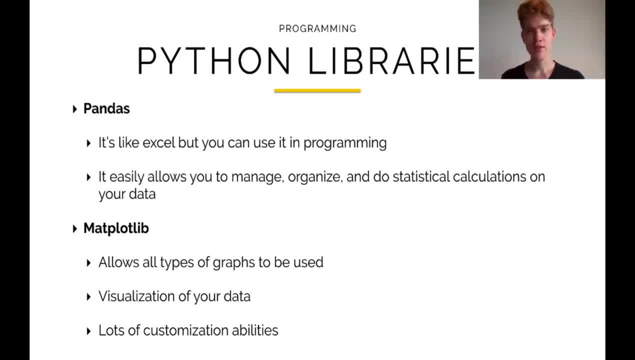 libraries are great for they're developed for by the community, for everyone to use. you know everyone is helping each other, um, and these libraries, they just bring a lot of power with it, and so one of these libraries is called pandas, and pandas is pretty much like xbox. 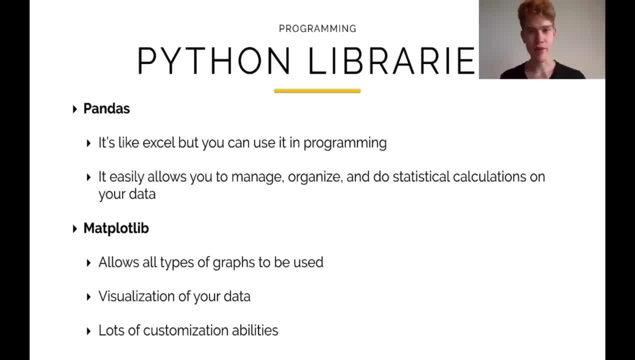 it's not so much about what's good for you, but it's rather about the if you want to use it, which is you can use a lot of stuff anywhere like, which is you can use a lot of stuff anywhere like it can be a lot of programming with it, which just makes it so much better because we can do things. 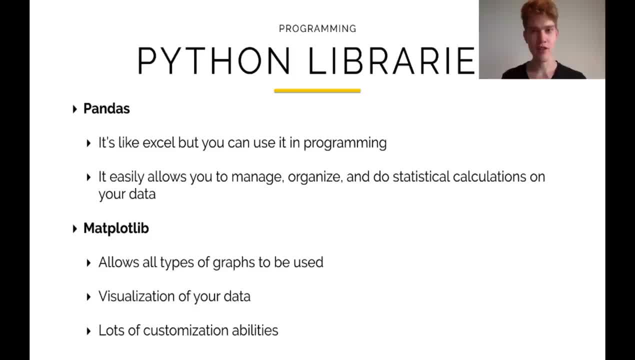 so fast with it we can do all this customization, we can do all this automation, whereas you know, like excel, if you give it too much stuff, too much to run, it would just start to crash because it has to handle all of this other things, all these other visual things. you know the ui and there's a lot more. it's a lot. it's not structured as well. 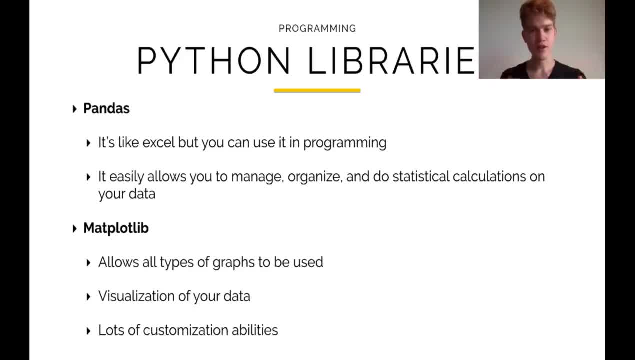 whereas in programming- the program you know, your computer just goes through everything step by step. it doesn't have to take care of all of these visualizations. it doesn't have to take care of all of these visualizations. you know those things. I mean like things. it just does the calculations down below. But we can still do all sorts of data management. 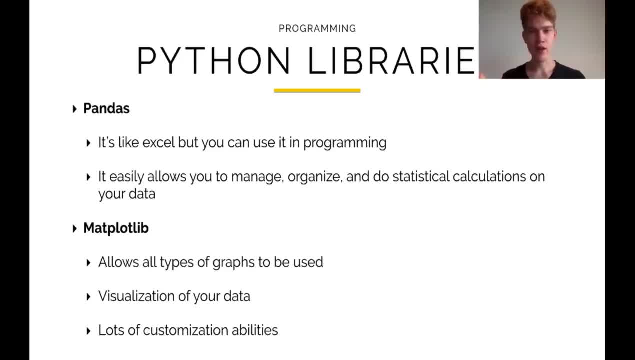 with it, So we can shift our data around. we can drop columns, we can split things up. you know, we can split things up by row, we can pick out certain rows. we can even do statistical calculations on our data, So we can say: you know, hey, calculate the mean for this, we don't even have to. 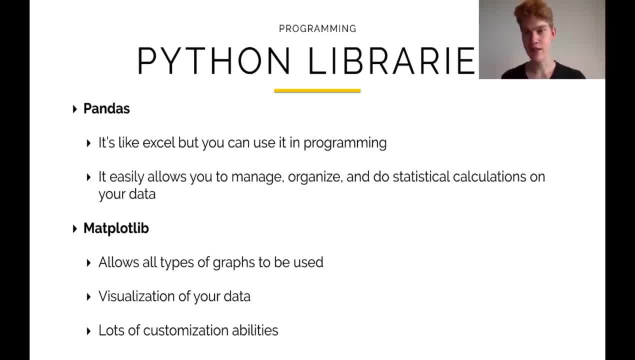 you know, make our own formula for calculating the mean, or for calculating the standard deviation, or for calculating correlation between different columns. all of that can be done with pandas with just a you know a couple of keywords, And so it's really easy to do data analysis with it. 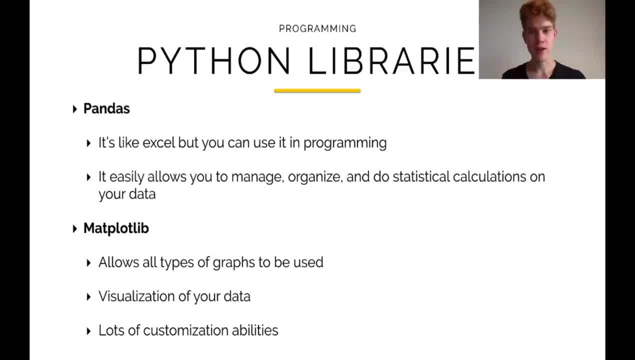 Because all of the functions are there and we know exactly what we want to do, But we don't have to write the code for all of it. So if you wanted to look at correlations, we just say, hey, pandas, do correlations rather than having to, you know, code all the correlations for ourselves. 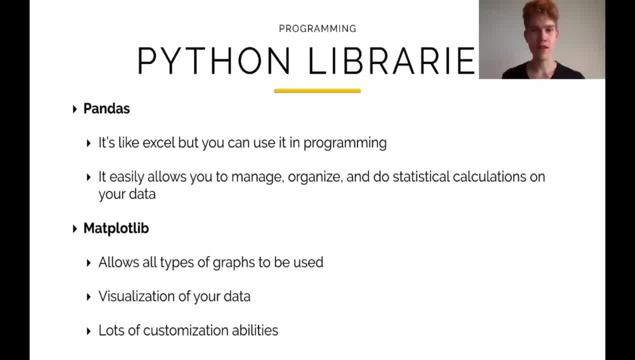 doing, you know, coding that whole algorithm And that makes it really easy and really fast to get results and to get to where you're heading, because you don't have to go into any of these middle places. you can pretty much just skip the. 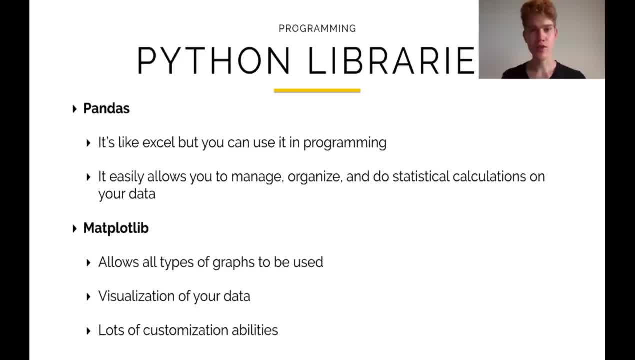 middleman, of having to, you know, write all of those algorithms yourself And you can just use them so that you have your start, you have your idea, you know exactly what you want to do And you can do exactly that to get to your goal. The other library that is very cool would be. 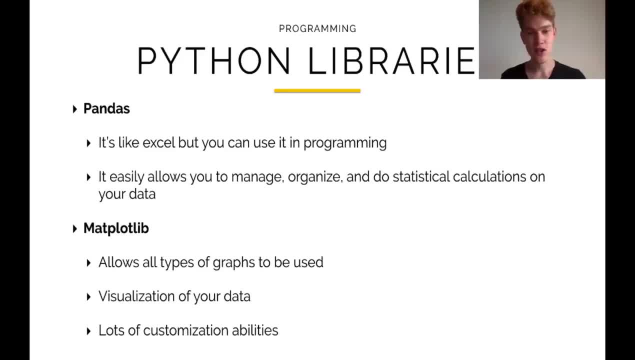 matplotlib, which is what I use a lot for data visualization, allows me to create graphs, allows me to visualize my data, allows a bunch of customization, so I can really just move everything around it. I can move my spines, I can turn things. 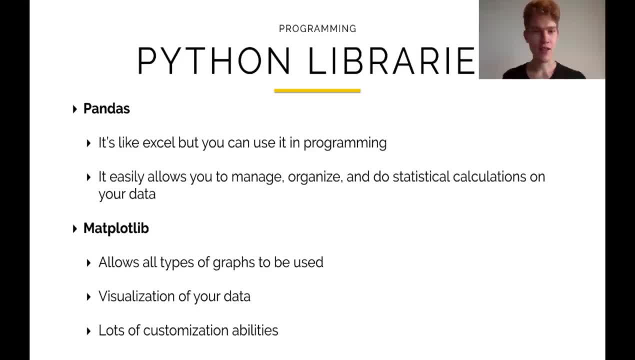 on and off. you know all of these things are very easy to do with matplotlib. there's a lot of great customization that I'm able to do with it. So these are like kind of two basic Python libraries that you should probably maybe get to know. or you can look at some of my other courses. 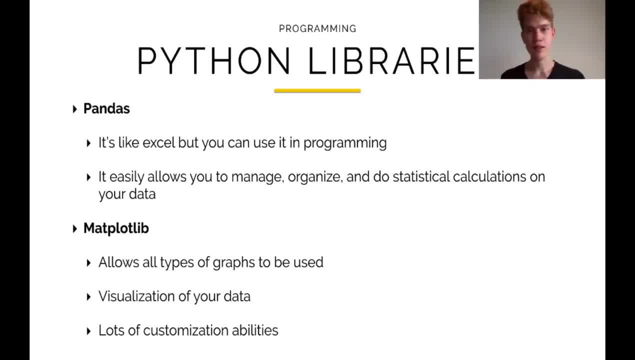 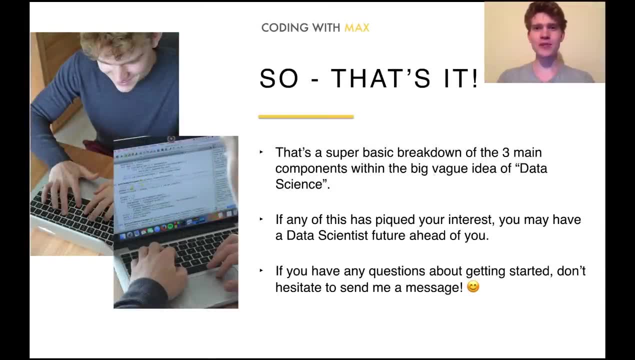 One of them, pandas, would deal with the data analysis part, and matplotlib would help you deal with the data visualization part of it. So that's it. That's a super basic breakdown of the three main components of the otherwise vague term data science. If any of this has piqued your interest, 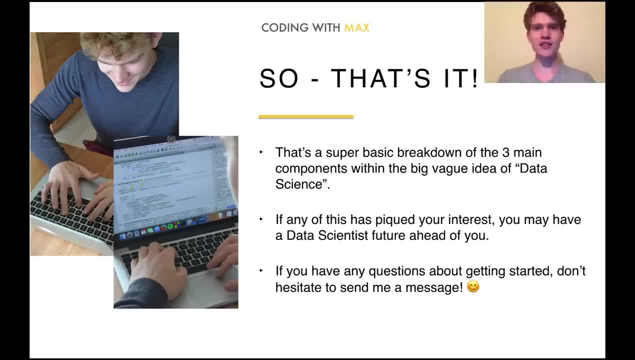 then you may have a data science feature ahead of you, And I encourage you to continue to pursue your interest. If you want to learn more from me, I've got a blog on my website, codingwithmaxcom, that dives more into different topics related to data science. 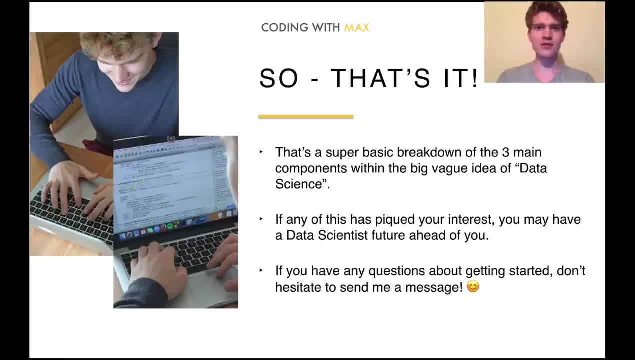 You can also get access to some of the resources, such as cheat sheets and workbooks, that I've compiled for you there. If you're serious about learning data science, you can also check out my courses on data science, which are designed to teach you all you need to know about data science. 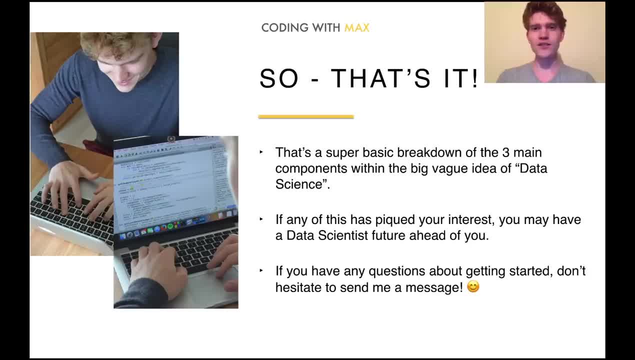 even if you have no prior experience. Of course, if you have any questions that aren't answered on my website, you can always feel free to reach out to me personally.